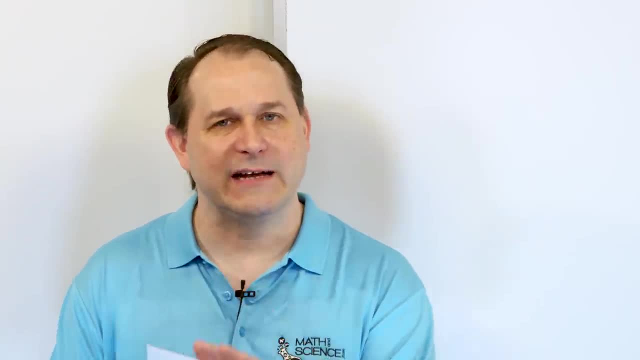 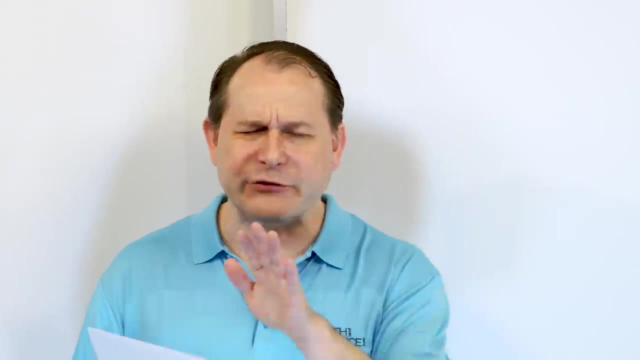 a lesson in three or four years, because this is the lesson that I wish somebody would have taught me right at the beginning of my journey throughout physics and chemistry. So in here we're going to talk about, primarily, topics in physics dealing with energy. But what? 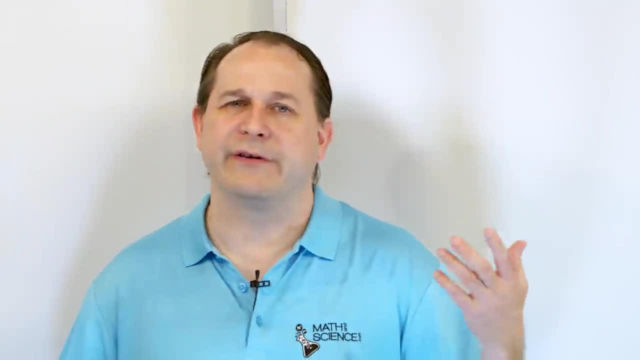 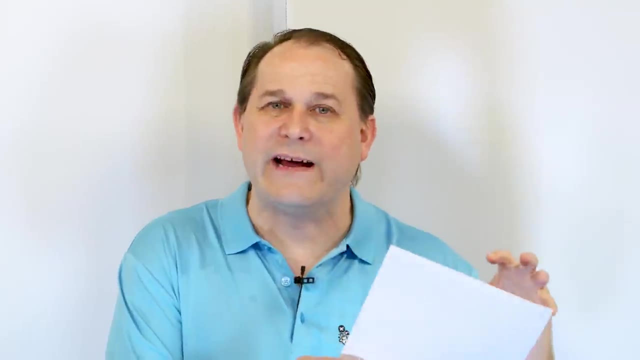 usually happens in a chemistry class is you start out learning about molecules and chemical reactions and you kind of like don't talk at all about what's actually happening really in the detailed level down low in terms of energy. But then about six or seven chapters into chemistry you start to learn about what's actually happening And then you start to 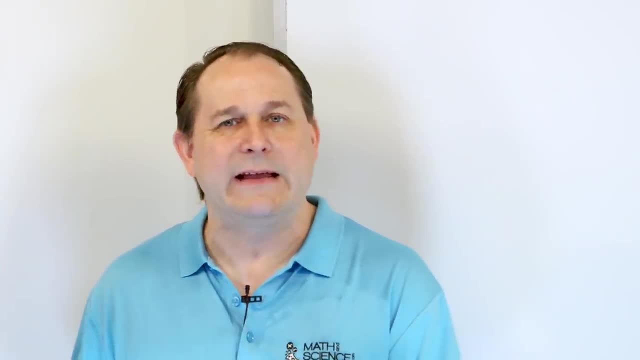 learn about what's actually happening in the detailed level down low in terms of energy. You start talking about energy a lot, And I really think that it's very beneficial to start that discussion earlier so that in the back of your mind when we talk about chemical, 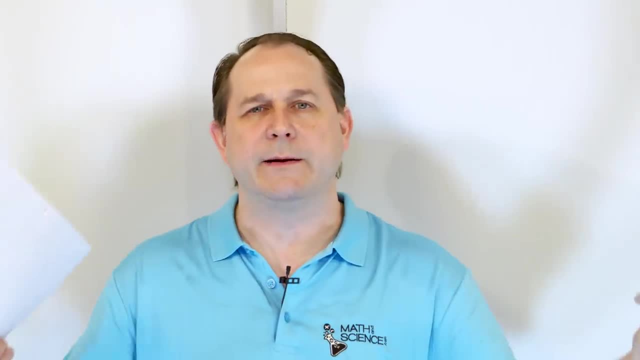 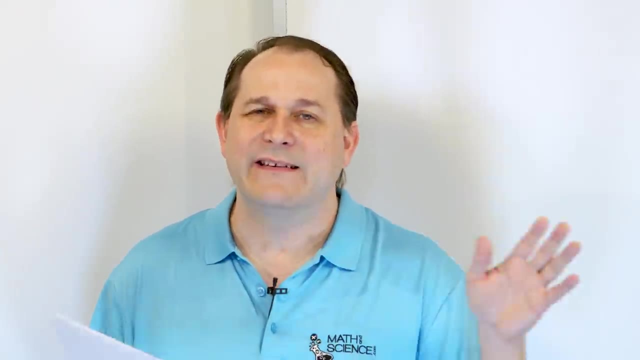 reactions. when we talk about electrons moving and things bonding and breaking bonds, then you know in the back of your mind what is happening at an energy level down below. Because, as I said many times before, if you understand what's happening in terms of energy, then 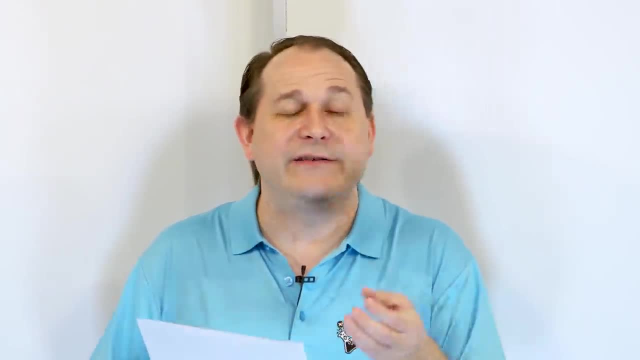 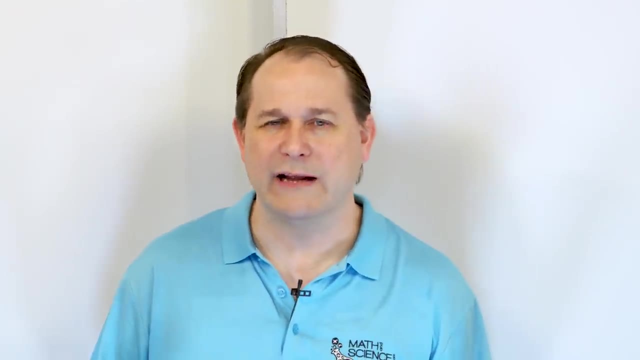 you understand the keys of the kingdom. the keys of the kingdom. I could teach you how to balance a chemical reaction right now, right, And you could do it, But you wouldn't really understand anything about what's happening at a lower level, And so a lot of times people push that off. But I really 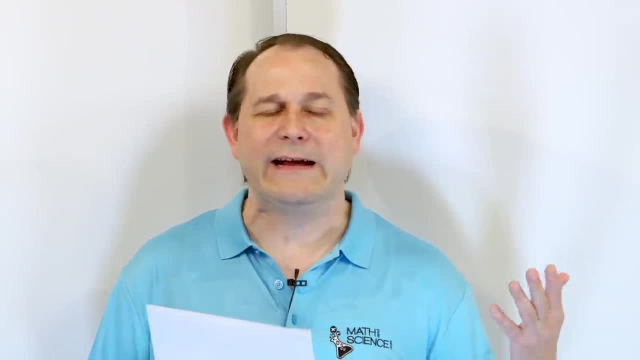 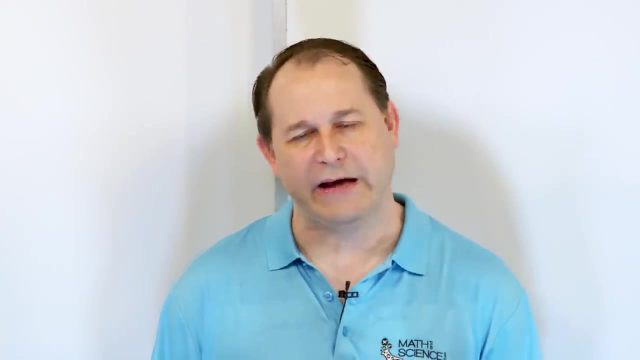 think that's not a great idea, because it's not hard to understand and it helps you grasp the material so much better. if we understand it early on, All right. So what are we talking about? the nature of energy? It sounds complicated, but actually you have everyday experience with all. 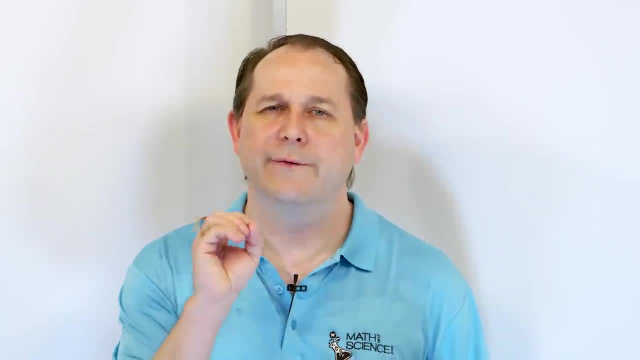 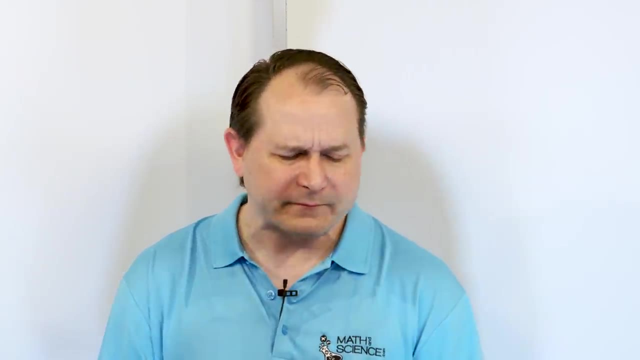 of these concepts, Okay, The most important one that I want you to focus on early is the concept of potential energy, And I want you to focus on potential energy, And I want you to focus on potential energy Now. I could write a definition for potential energy down, but, honestly, that's in. 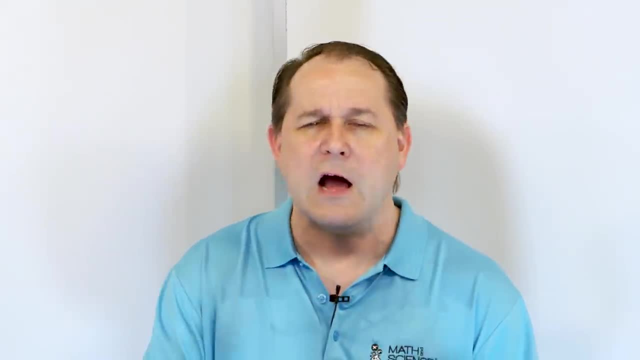 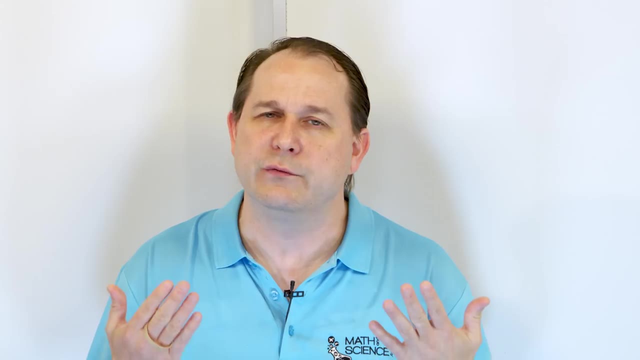 your textbook and it's not going to be that helpful to watch the word to see the words. I'm going to show you what potential energy is in terms of something you can understand, And just keep in mind that you might have to watch this lesson a few times because we're 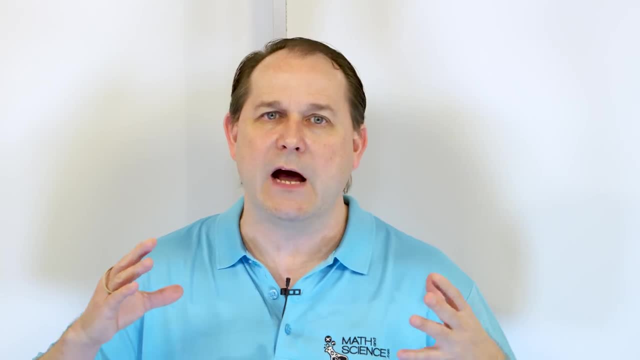 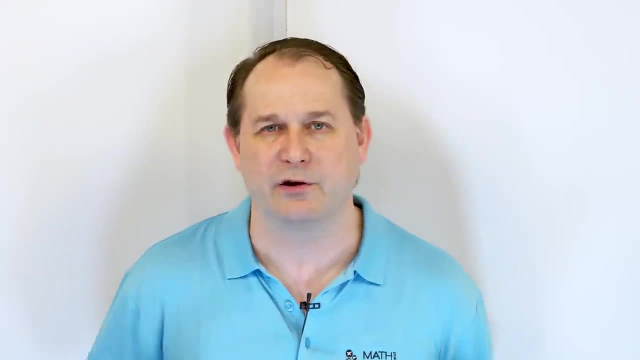 going to talk about a lot of different things and I can't break the lesson up. I need to keep it all together so you understand the differences. but you may have to watch it a couple of times so that it comes together in your mind. I promise it'll be worth your time. 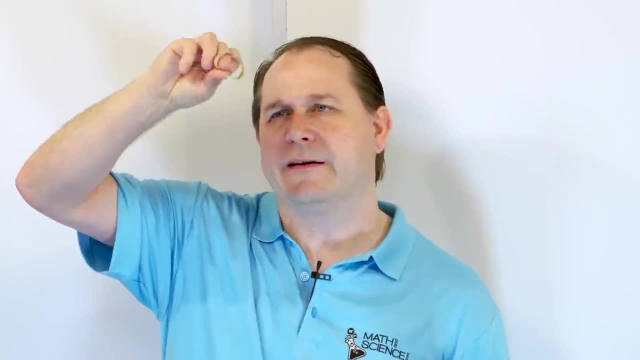 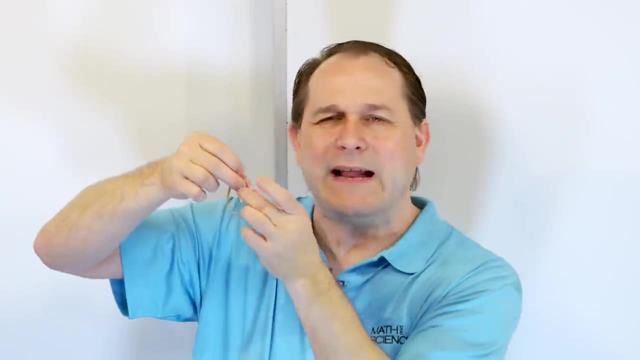 All right, Here is a rubber band. Right now, when the rubber band is freely dangling like this, it is not in any kind of tension, It's not pulling on me. Obviously it's in a relaxed state, right. But I think you all know that if I stretch this rubber band out, maybe to an extended state, 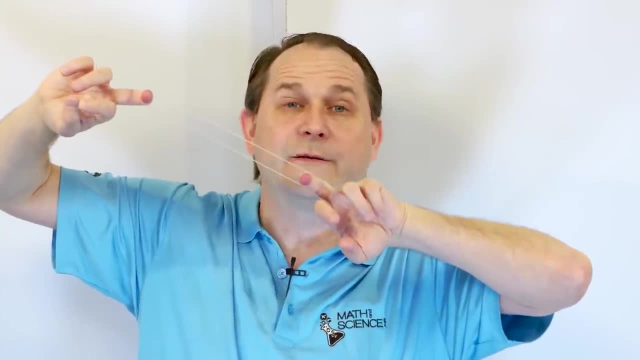 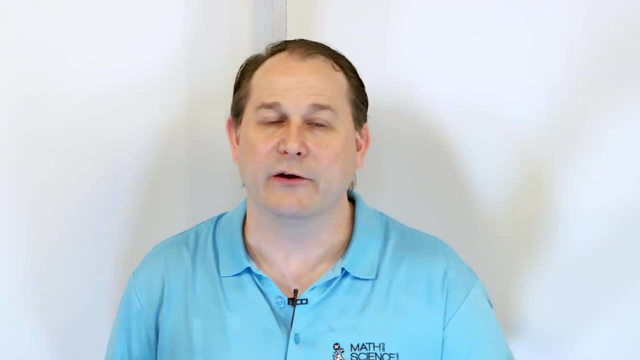 like this: it's pulling on my fingers, It's trying to pull my fingers together. There's an attractive force pulling my fingers together. Now we're going to get into a lot of detail later as to where these attractive forces come, but I'll tell you the attractive forces come from. 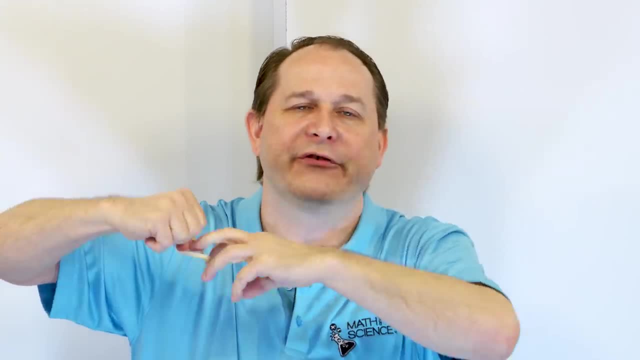 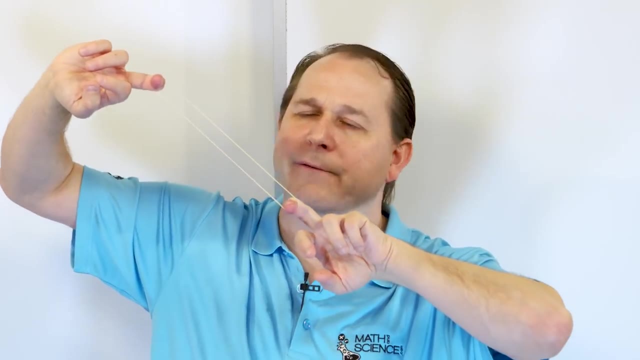 the bonds between the atoms. in this rubber There's a big attraction force down at a microscopic layer right. But when we zoom out and look at the whole rubber band, all we know is that our fingers are being pulled together. Now my fingers are not moving, Nothing is moving. 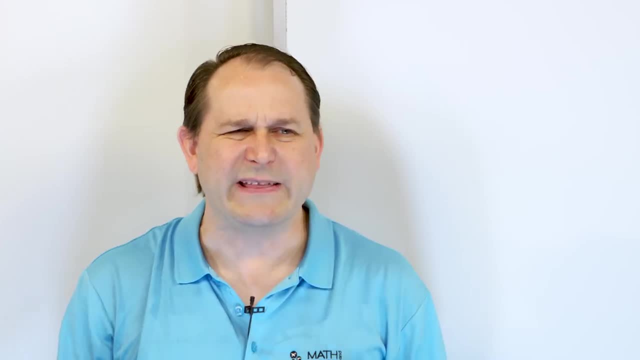 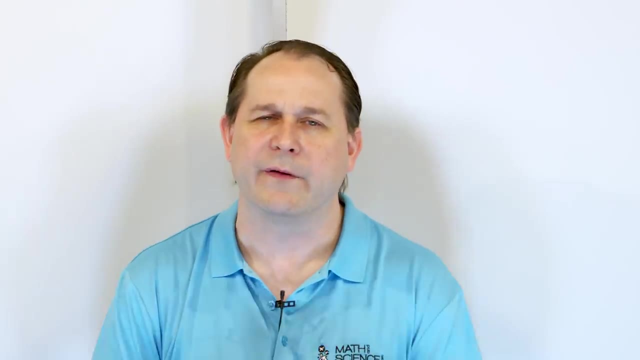 So you know, usually we think of energy, we think about somebody running or we think about firing a bullet going really fast, We think about a spacecraft, high energy going around the earth. We don't usually think about things that don't move like this as having high 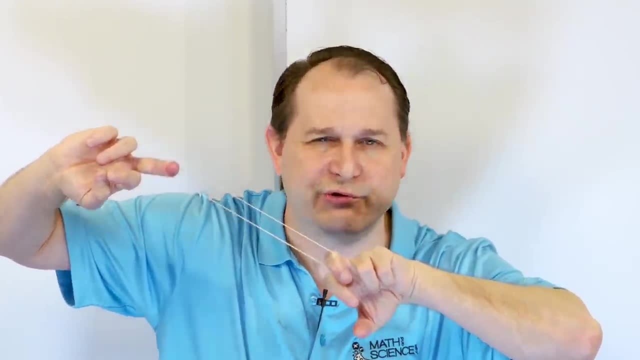 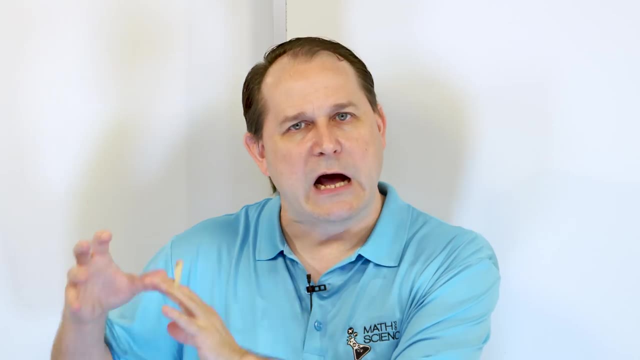 energy. but it does have high energy. So in chemistry usually usually when it says: this molecule is in a high energy state, this atom is in a high energy state, this electron is in a high energy state. Usually in chemistry when we say that, when we talk about energy, usually 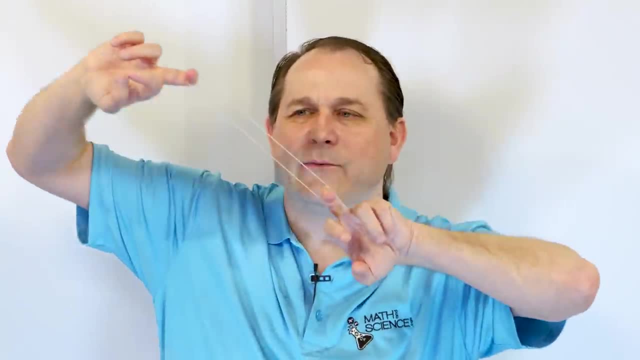 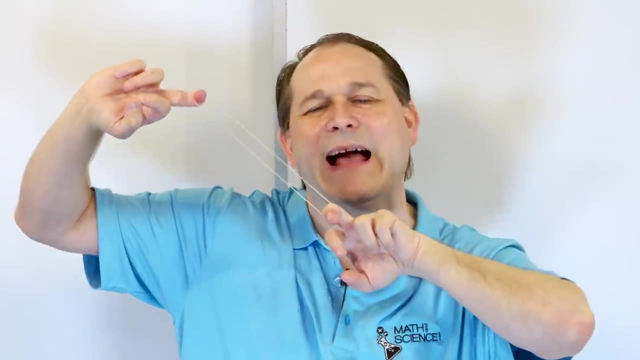 they're talking about potential energy. So this rubber band is not moving, but there is a force between my fingers that the rubber band is exerting And because of that force there is a high potential energy situation. So when we talk about energy, usually they're talking about 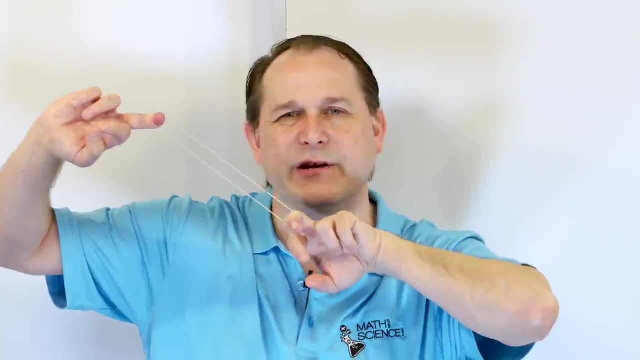 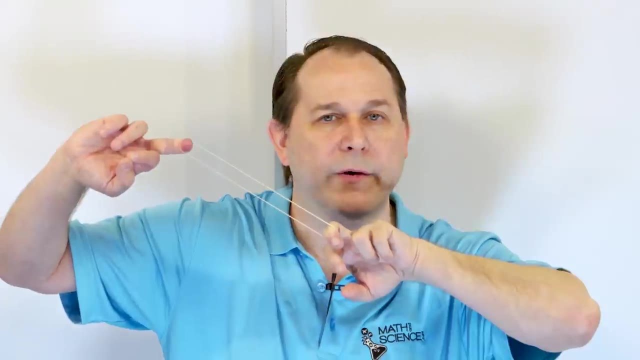 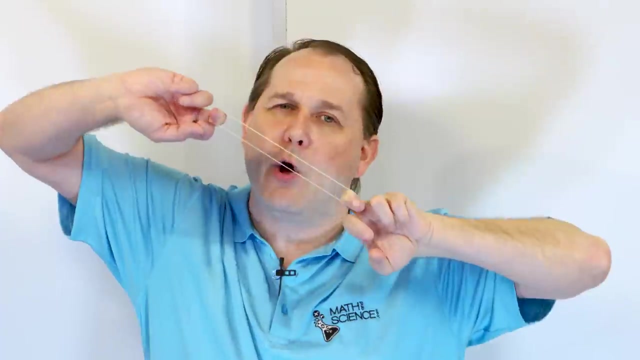 a situation going on here. You could just say it's high potential, but usually we can use the word potential energy. Potential energy is just the propensity or the ability or the potential to do work. Should I allow the system to go in the direction it wants to go? So right now I'm 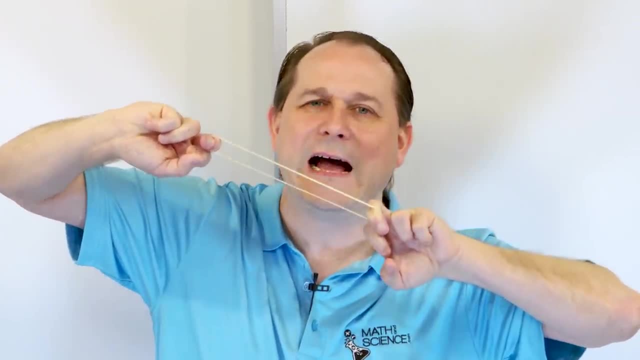 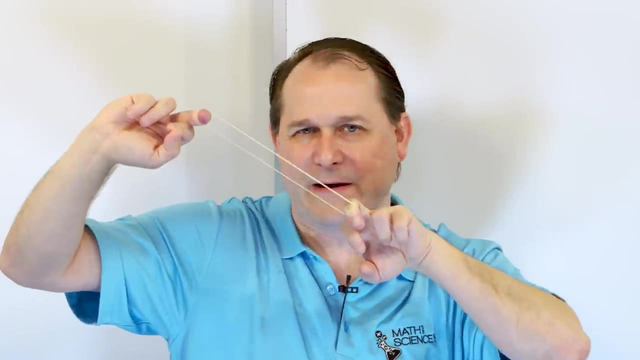 holding it back with my fingers right, Nothing's moving. So it's still in a high energy state. It wants to move. So if I were to let it go and let the force of this rubber band act on my fingers, then my fingers are going to come together. 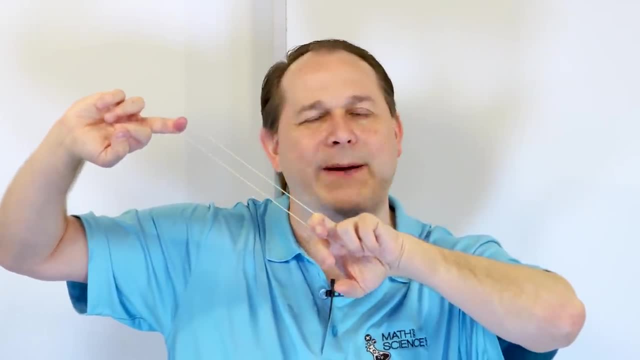 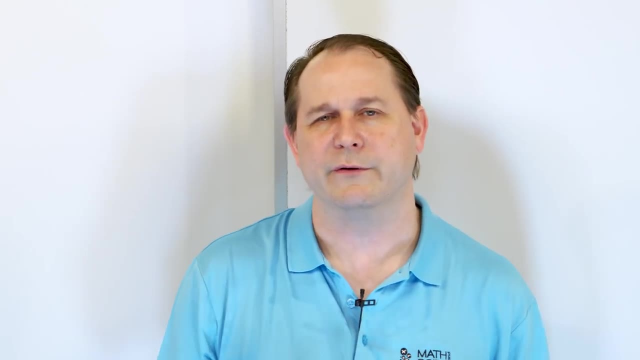 And the potential energy that the rubber band had exerting on my fingers is now changed into the energy of motion, essentially when the system starts to move. So when you have a system that basically there's a force involved but nothing is moving and you're kind of holding, 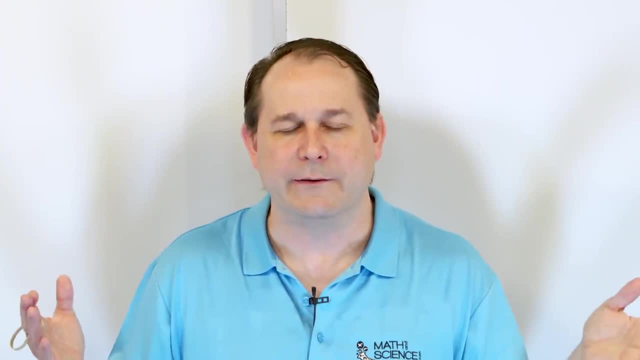 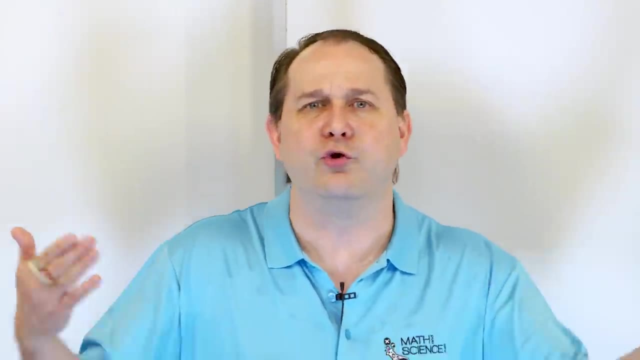 the force back, you're in a high potential energy situation. It means if you look at textbook definition up, the book definition will say something like: potential energy is the potential to do work- Work we're going to talk about in just a minute. 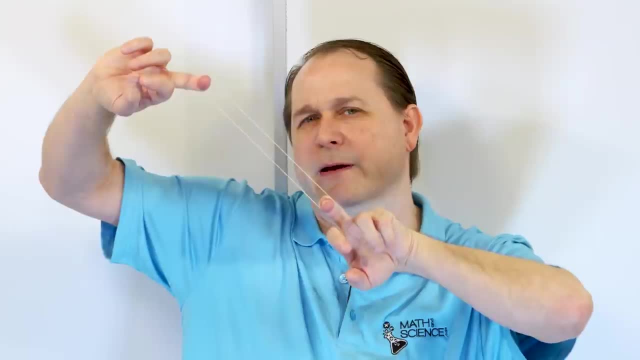 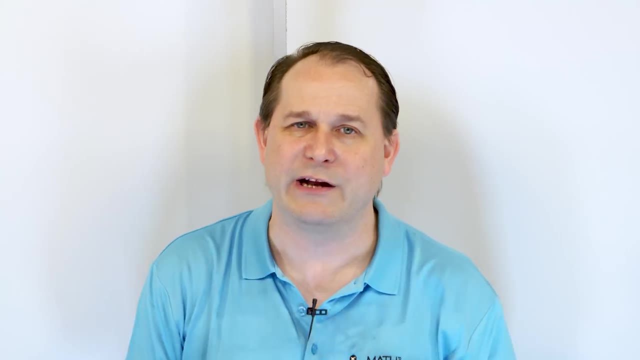 Work is when things are moving, when things start moving. right Right now nothing's moving, So there's just the potential to turn this energy, this potential energy, into movement. We call it potential energy because if you let the system then move, then it can, that potential can turn. 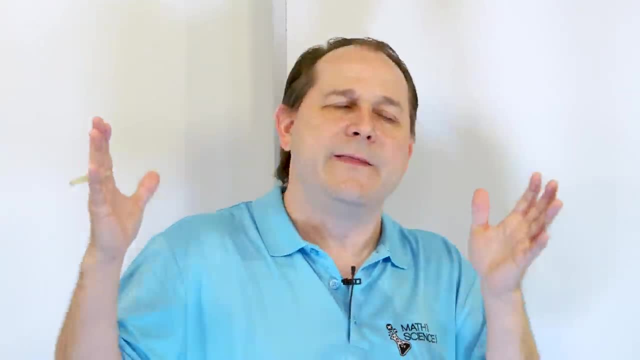 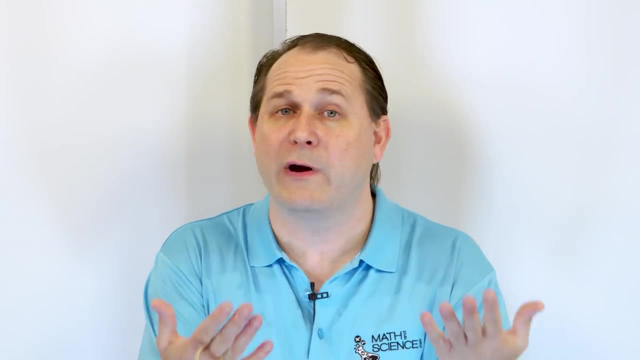 the potential that it had then become something that is moving essentially. So you can think of the word potential energy being when you have, when someone grows up, and they have great potential. you know someone has great potential to be a doctor, someone has great 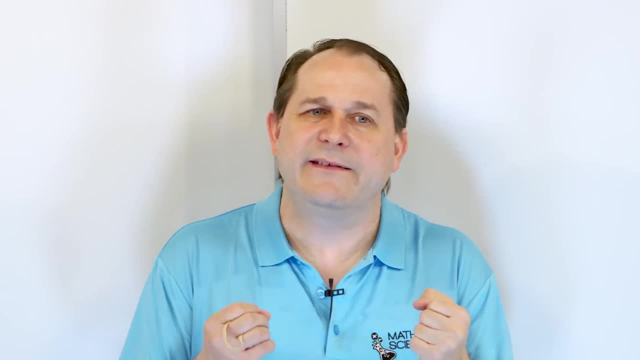 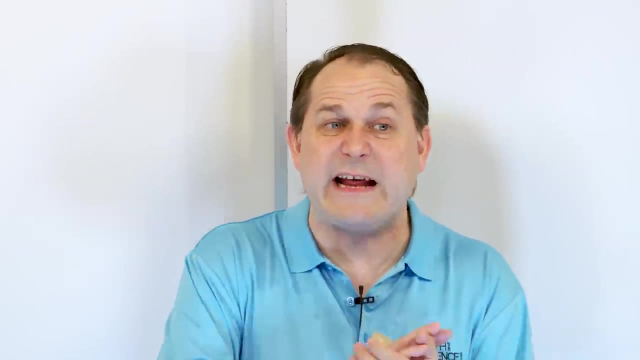 potential to be a- you know whatever- an engineer or whatever. It just means that they have some ability inside of themselves. You think they have some sort of ability, right, And if they just harness that ability, then they can do a lot of good or do a lot of whatever it is they want to. 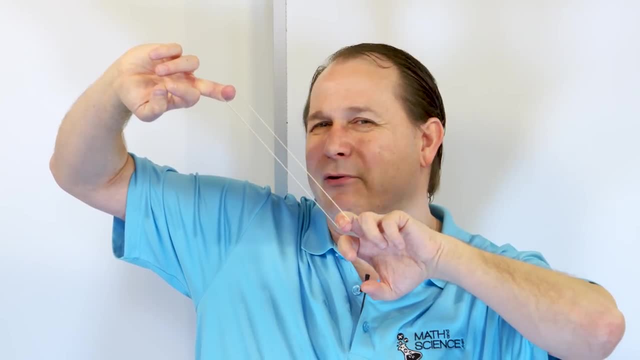 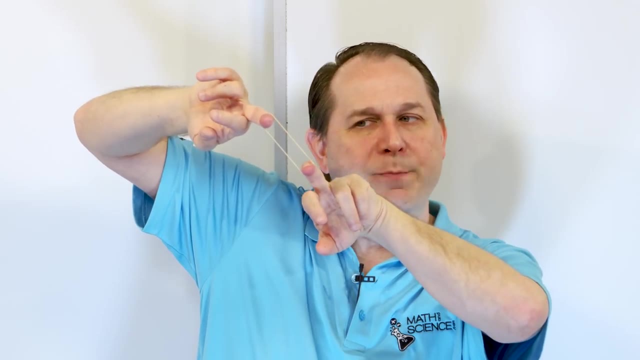 do. Potential energy is when something wants to move but now it really can't. But if you let it move, then things will start moving. The potential energy is that situation. This is a low potential energy. This is higher potential energy. This is higher potential energy because, as I pull the, 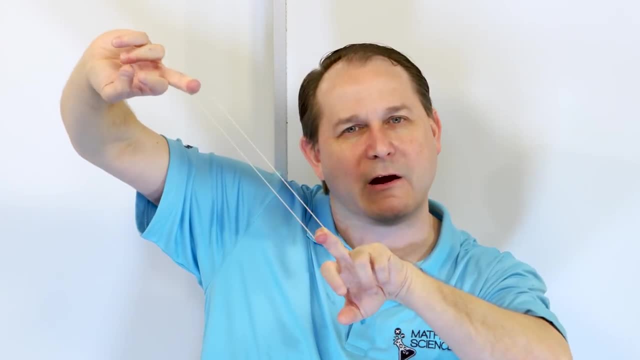 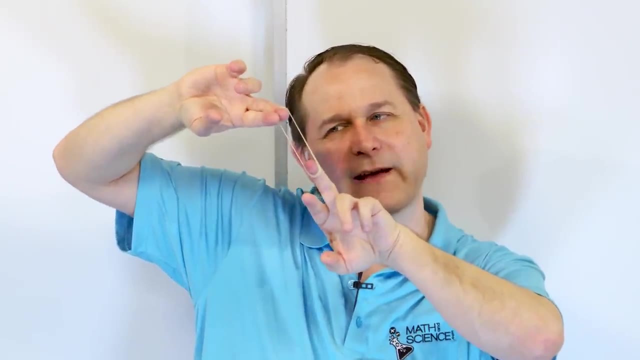 thing apart, it's pulling back harder. There's more potential here, because if I let it go, then a lot of movement happens. A lot of motion happens and there's less potential energy here, because if I let it go, then of course less less movement happens. that I keep talking about it. 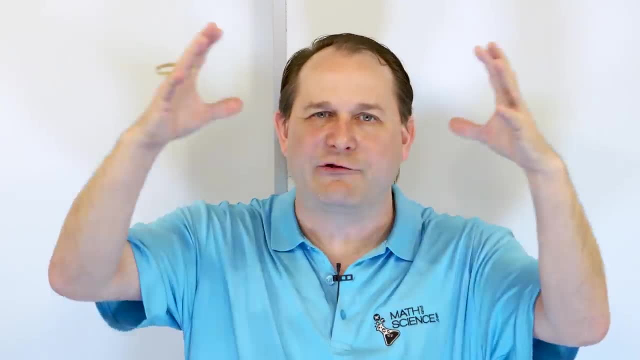 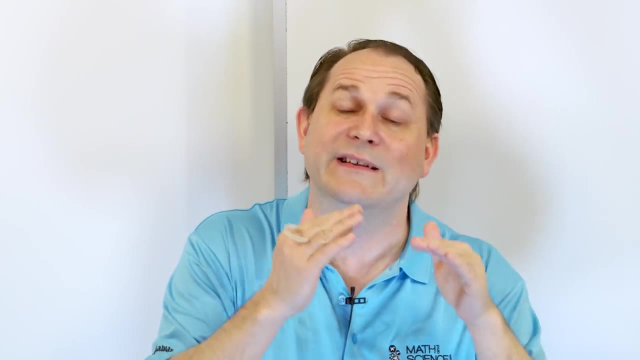 because potential energy is central to chemistry. When we talk about electrons and where they are orbiting around the atom, we're going to talk about energy levels. Well, guess what? Those energy levels are potential energy levels. They could pretty pretty much call them potential. 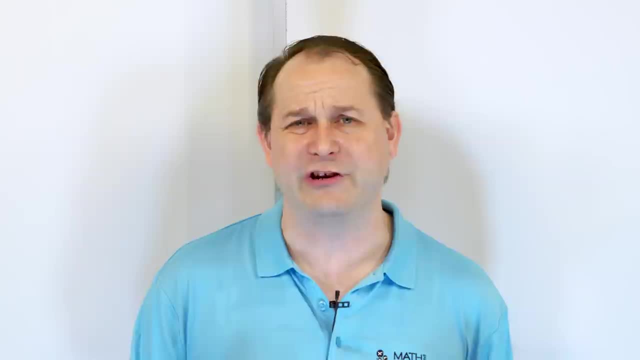 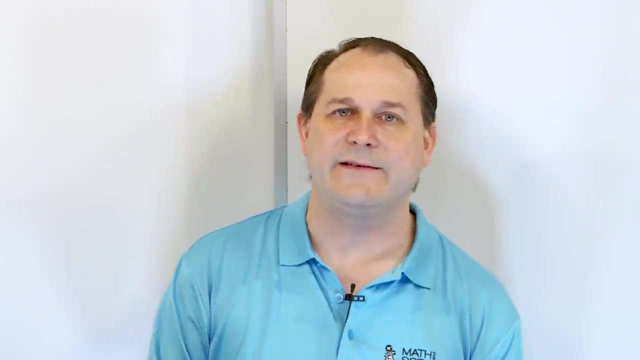 energy levels. They could call it that, but they don't. They just call it energy levels. right Now, the next thing we have to talk about, because we have three things we have to talk about. we have to talk about three things and then we tie it together. The first we just covered. 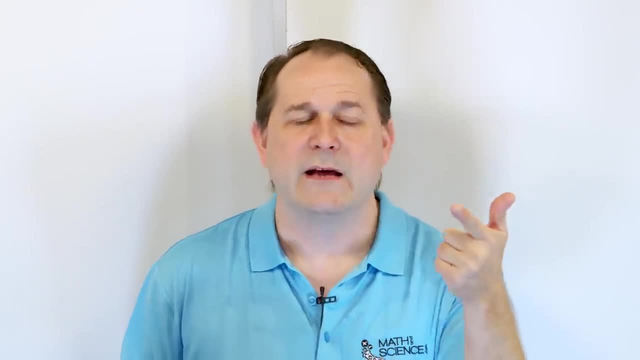 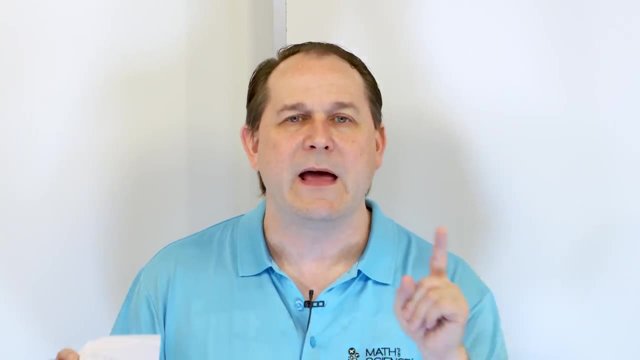 potential energy. The second one we have to cover is work. The next one after that we have to cover is kinetic energy. Once we get them all down on the board, then we can talk about the interplay between all of them, And then we'll also tie it back to what's going on in an atom and why we are. 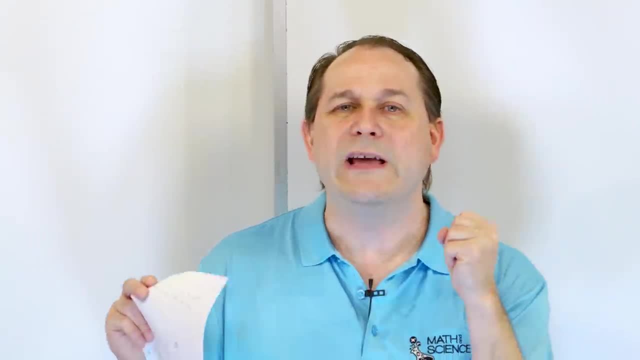 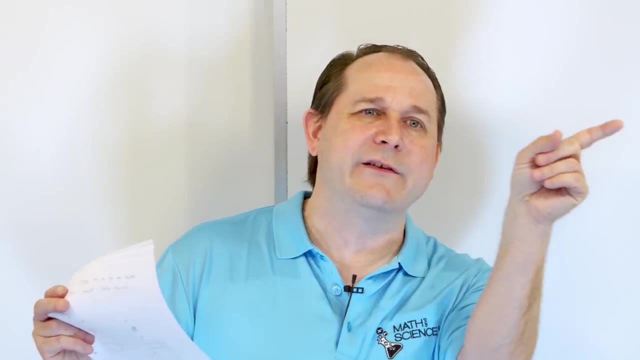 caring about this And I will tell you, the punchline is that we're going to talk about up front. We care about the energy level, or the energy state of atoms and molecules, because a chemical reaction is more or less going to happen when you get to a. in general, nature likes to go. 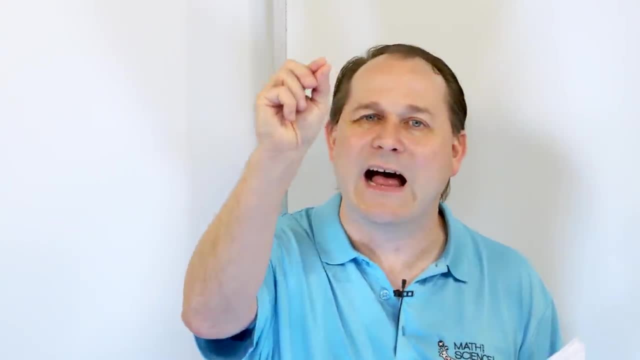 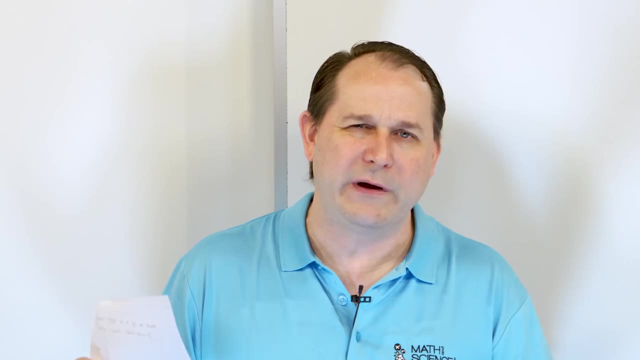 to a lower energy state. right When you go down the slide, you fall down to a lower energy state, falling down. When you do a chemical reaction, it generally unless something weird is going on. we'll talk about those situations Generally, when you start with something and your chemical 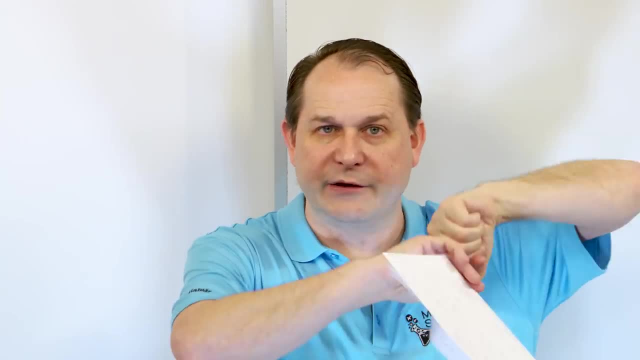 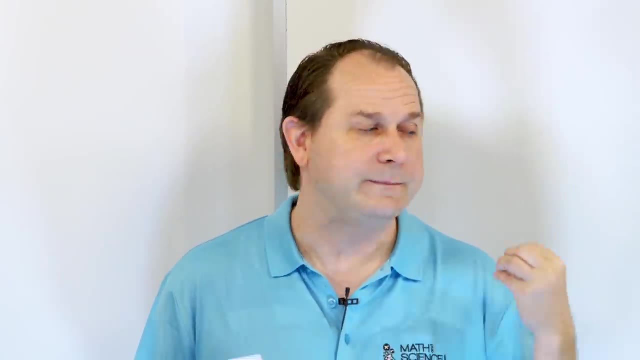 reaction happens and you end up with different problems. you're going to have a lot of energy products, different molecules, bonding together. They're doing it because they're trying to get to a lower energy state. So that's why I'm bringing up energy so early, So you have a in the back. 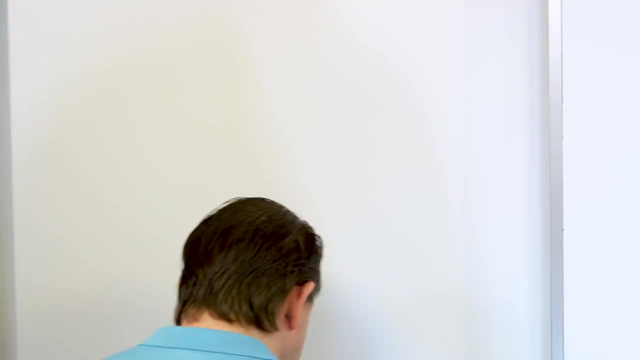 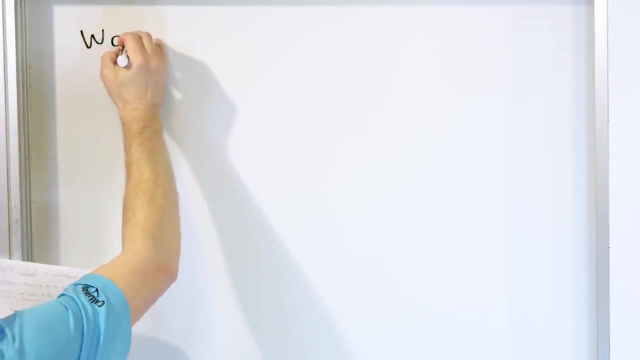 of your mind. Now we have to talk about work. What is work? Because work is very closely related to potential energy. So we have work and I'm just going to read the definition to you. It's going to be in your textbook, but mostly I'm going to draw a picture to explain what work is. So backing up. 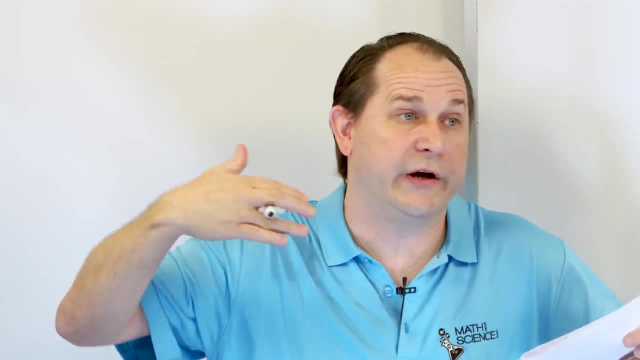 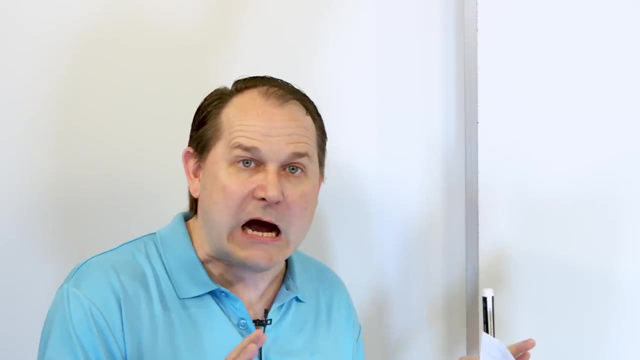 potential energy is the capacity to do work. What is work? Work is energy used when a force moves an object through a distance. right, If I have a box and this box is in front of me and I push the box, I'm exerting a force. The box then. 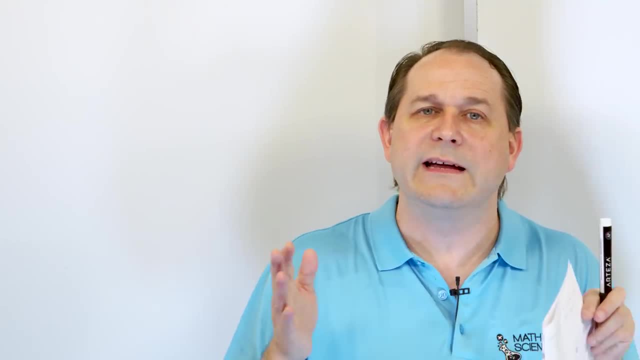 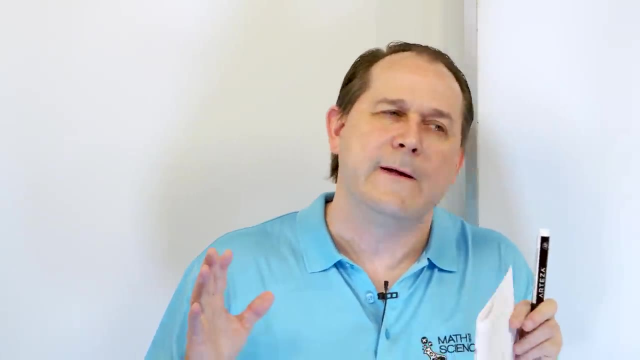 moves through a certain distance in the direction of motion. Then it said that I have done work on the box. in moving the box from point A to point B- That is the physics definition of work- I have to be exerting a force, and then it has to also move through some distance. D. And then what do we have? 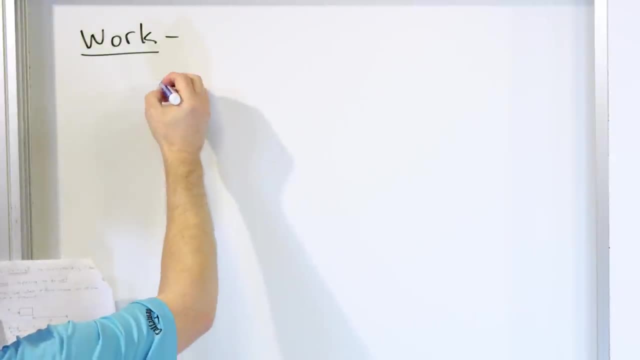 We have this situation here. So here I have some box, I'm just going to draw a little box, nothing special. I'm exerting some force, I'm just literally standing here pushing this direction, And then the box ends up in some final position. So I'm putting a little dot there, because some 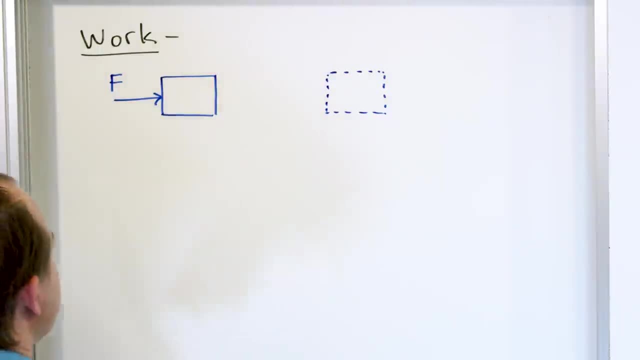 time has passed and I've moved it here. Now, how far did the box move? Well, you can pick the trailing edge to the trailing edge or the leading edge to the leading edge. Either way, if you pick a consistent place, it's going to move through some distance. 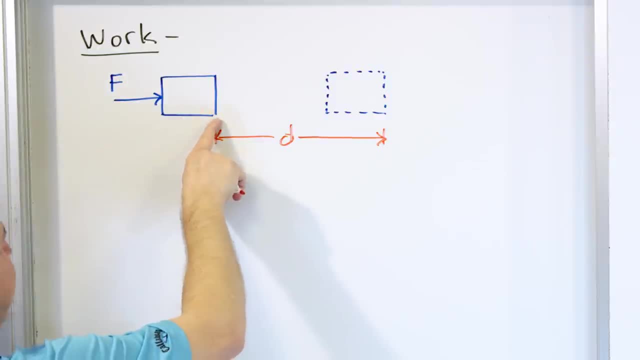 D to get to its final destination. So the trailing edge of the box to the new trailing edge of the box moves through some distance D. So if you push a box with a force F and then- as now, don't forget- once it's moving, you're still pushing on it with a constant force F. See this equation I'm about to. 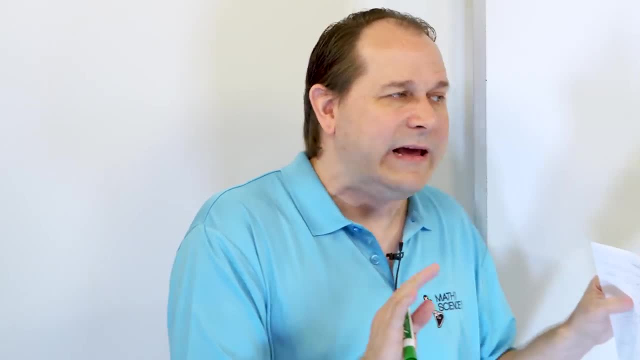 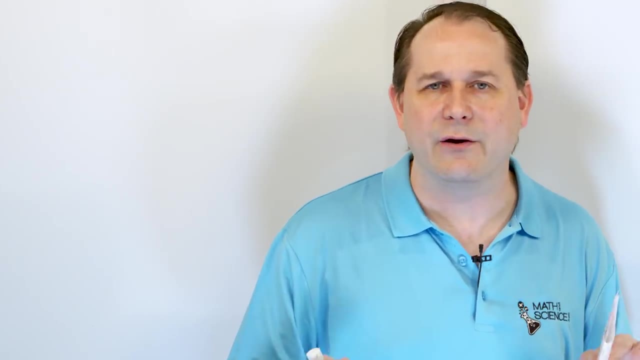 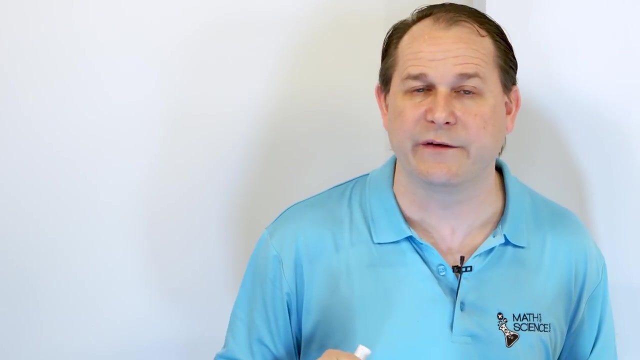 write. It's assuming that the force that you're applying is a constant force that doesn't change. If the force changes, like if you start pushing harder or softer, then you have to use calculus to handle a more complicated situation. We're not going to do that here. We're going to assume the force I'm pushing is a constant force. 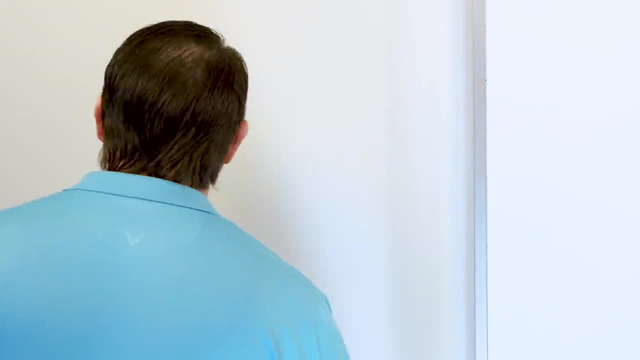 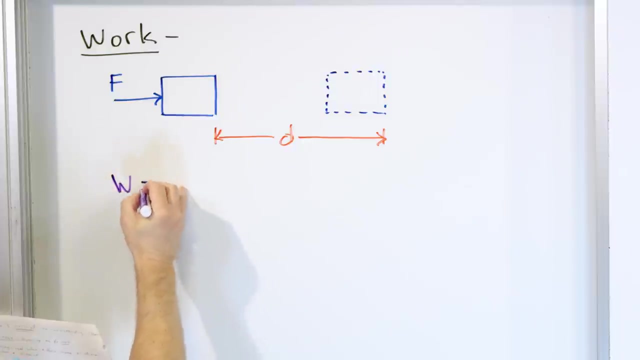 It never changes. And then the box moves through some distance, D All right. And then, once we have these two conditions here, then we say that the work done on the box is equal to the force multiplied by the distance. Now I have to explain a few things here that are very important. 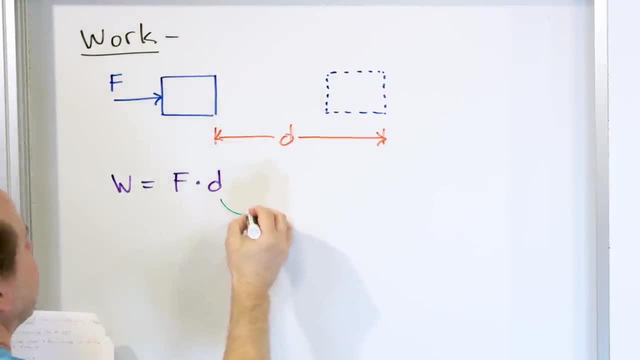 All right, The distance. the distance is in meters, which is a constant force, And then the distance is a constant force, And then the distance is a constant force, And then the distance is in right. Now I'm telling you the units that we have to use. 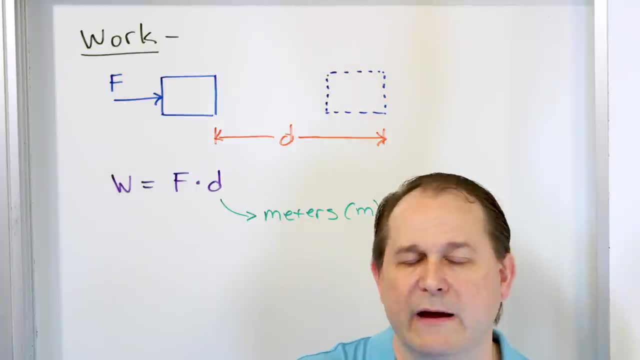 so that when we calculate things we have to have them in the proper unit And then you know what unit you're getting, what you're calculating here. So the distance are in meters. If the distance not given to you in meters, then convert it to meters and then stick it in here. The force is a unit in. 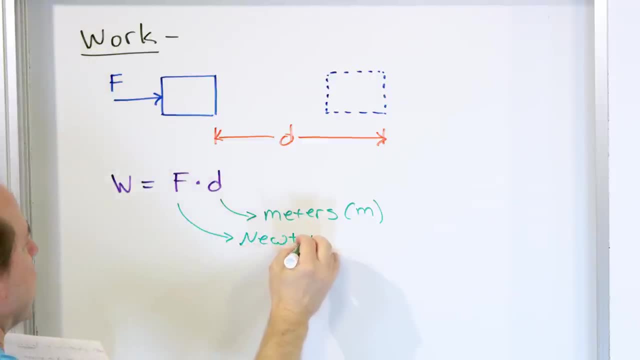 physics we call a Newton right And we call that capital N. So you might be thinking pounds of force in the English system. In engineering and science we use Newtons. You can do a straight conversion from pounds of force to Newtons. Not hard to do. but you always want, we don't want to. 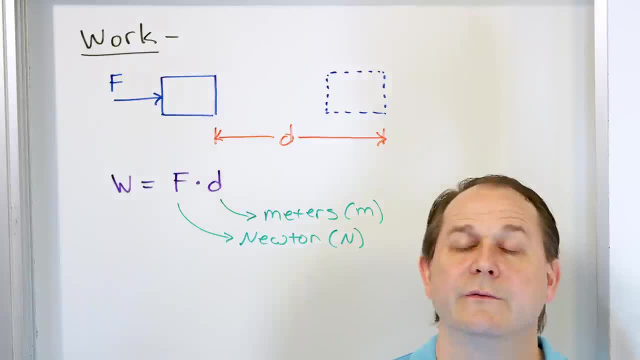 deal with pounds. Okay, Ever We want. a force is going to be a Newtons and distance is going to be in meters. And so when you take a force and a given number of Newtons and it's acting on a body that moves through a distance D in the same direction of the motion, then the work is given in. 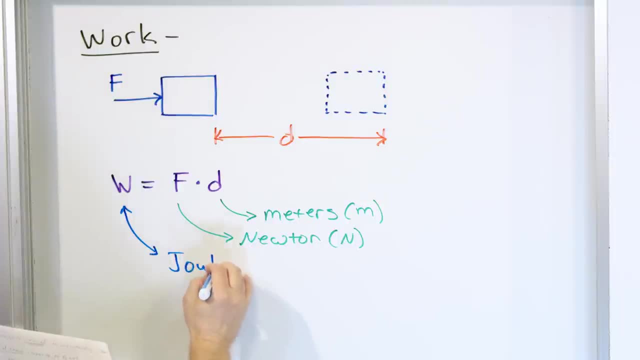 a unit which is called a joule right, And a joule is the unit Which we just abbreviate J. Now most people here in the beginning have never really heard of a unit of a joule. but actually you do have some sort of experience with joule, You may have. 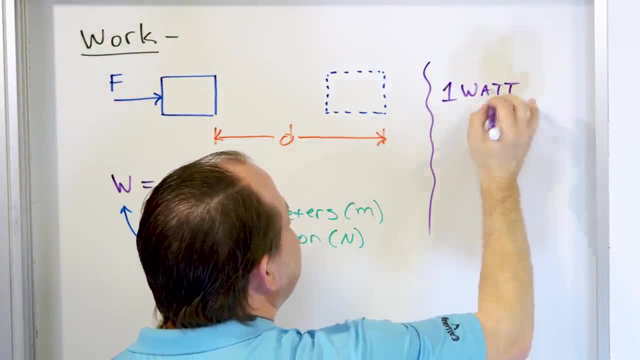 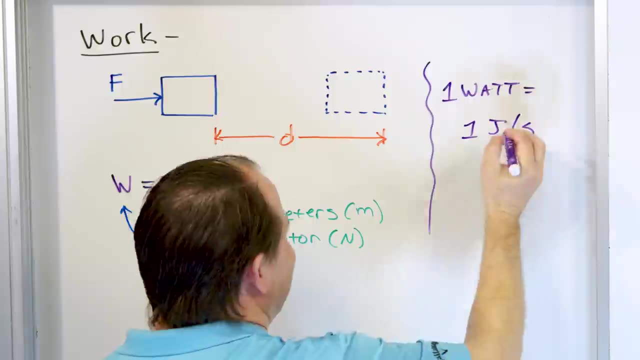 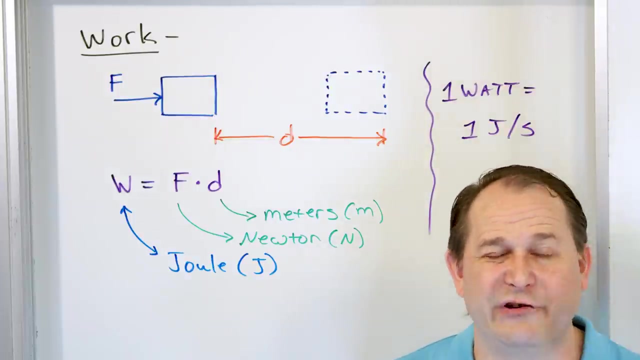 heard of a watt right: A 60 watt light bulb, a 120 watt light bulb, something like that. A watt is equal to one joule per second. So you see, the watts that you've heard of throughout your life like this many watts, that many watts. that is actually not a unit of energy. It's a unit. 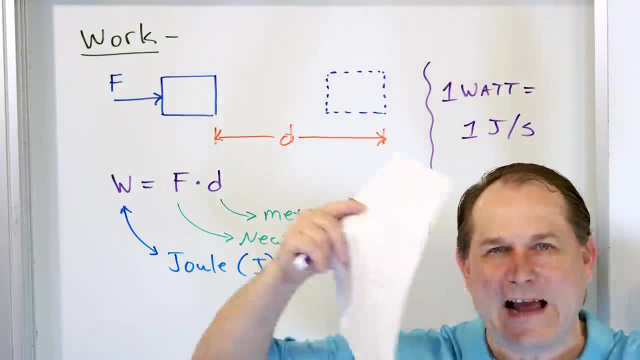 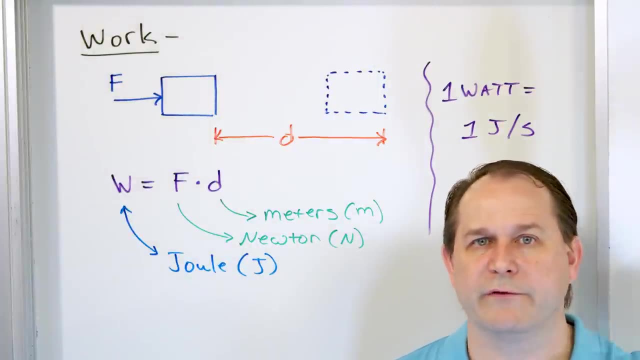 of energy flow. It's joules per second. So here I have lights hitting me from everywhere. Let's say that we had a 60 watt light bulb, Then every second it would be that 60 more joules If it's. 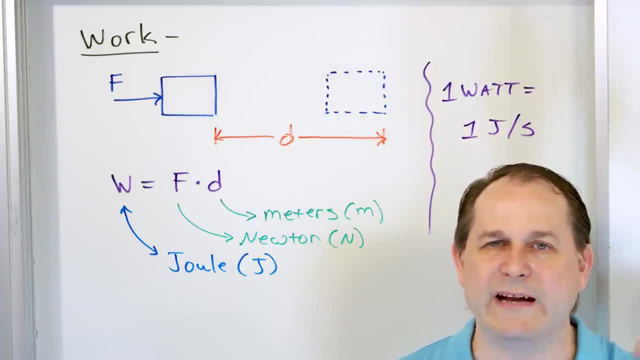 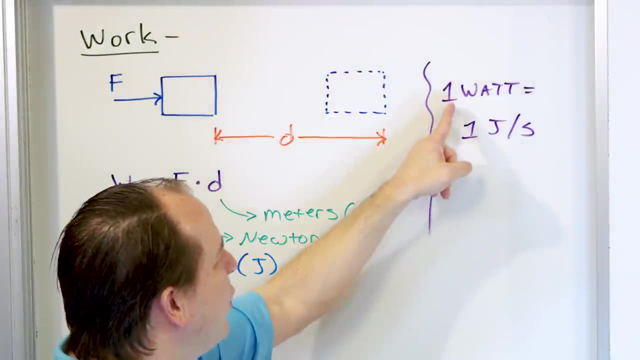 a 60 watt light bulb. that second, next second: 60 more joules hitting me, 60 more joules hitting me. 60 more joules hitting me, 60 more joules hit it. You see how that goes. So when we use the word, 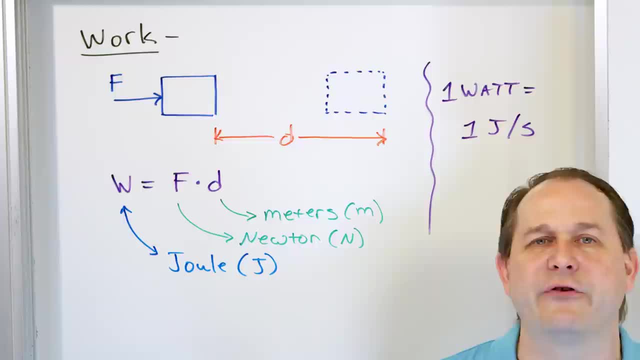 watt. that's a shorthand way of telling you how much energy is coming per second. And when you have a 60 joule light bulb or 60 watt light bulb, it's 60 joules per second. So when you have a 60. 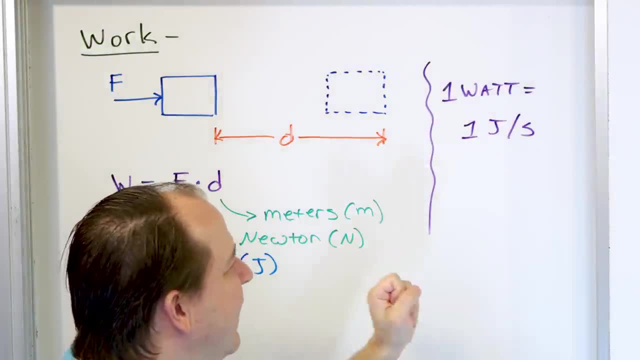 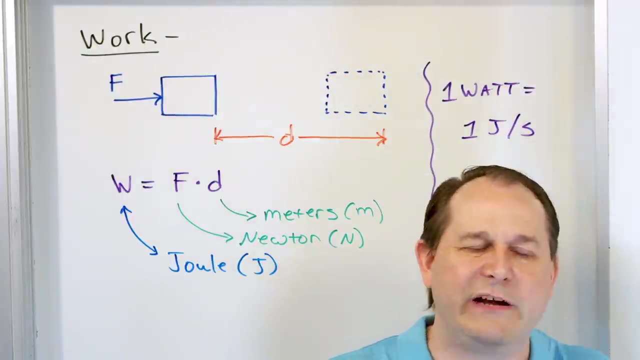 joules per second, because one watt is one joule per second. So it's kind of a crash course in units here. but I just don't want you to get confused with watts and joules. Joules is just how much energy you have available to do something. Watts is like a continuous flow of energy over. 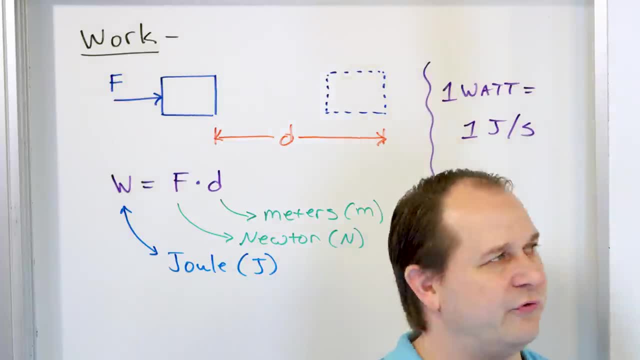 time, every second, every second, that many more joules, that many more joules, and so on. So the unit that you calculate this work is in joules. We're also going to learn in a few minutes that the unit of potential energy is also in joules and the unit of 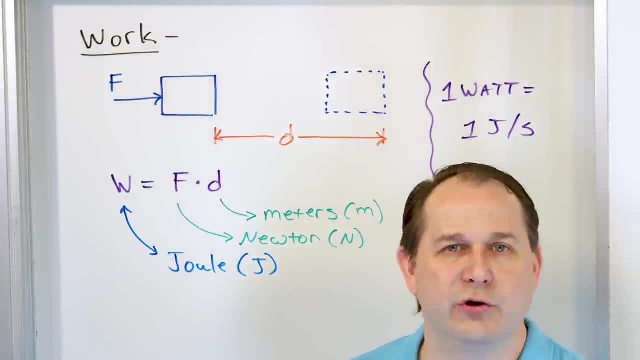 kinetic energy is also in joules. So kinetic energy unit of joules, potential energy unit of joules, work unit of joules- they're all in the same unit. They're all in the unit of energy. That means they're all very closely related And that's why I can't break this long lesson up. 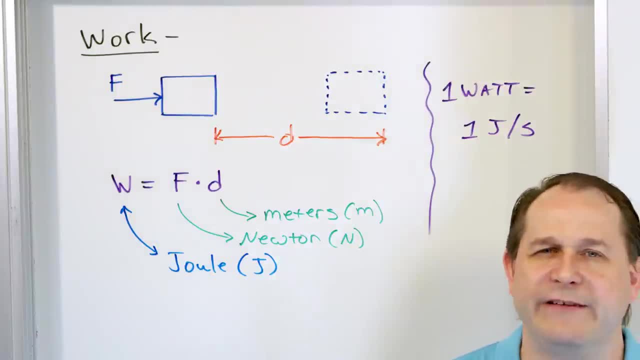 because they're all interrelated. If I broke it up, you would never see the continuity between them. All right, So unit of joules force distance. Now another thing I need to say. I wrote this as a dot here: force times distance, but this is a dot If you take a physics. 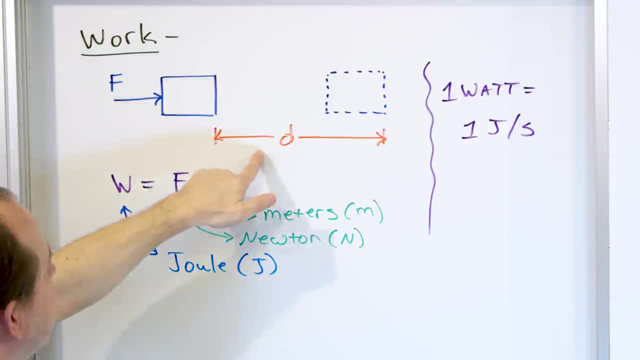 class you will learn that this works great if the force is lined up in the same direction as the distance. But if the force is angled at some angle, then it's not a straight multiplication. Basically the dot there comes from the dot product in math. I'm not going to get into it. 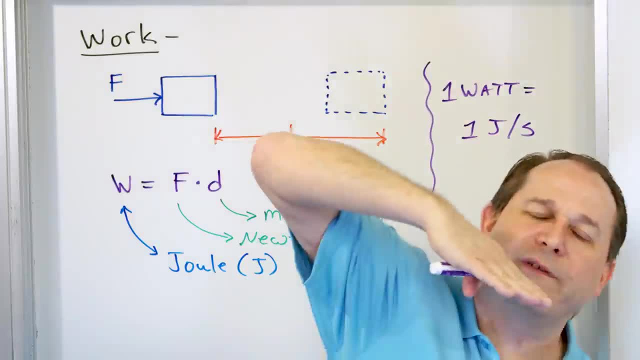 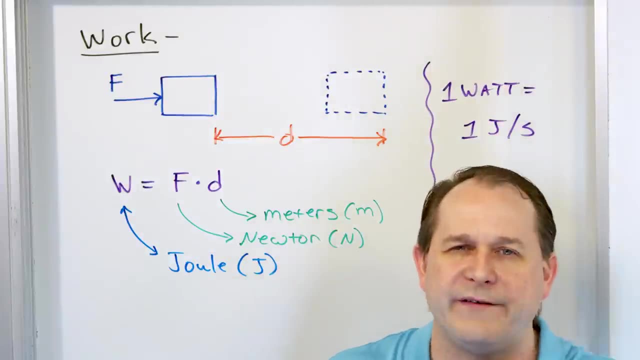 now, but basically the dot product handles the situation. If the force is angled to some angle, relative, like if the box is moving like this but you're pushing down at an angle, the only force that is really contributing to the work is the amount of the force acting in the direction of motion. So if you have a force, 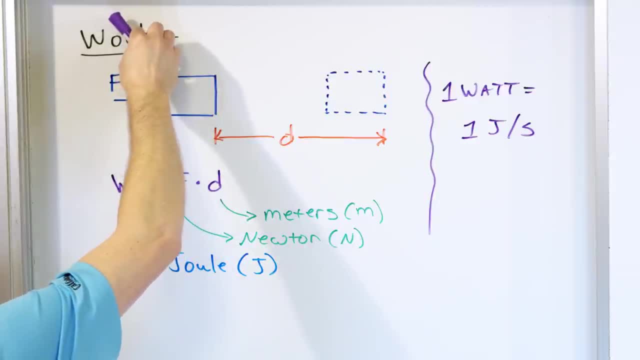 that's acting down at an angle instead of straight across, then you need some way to figure out how much force is, how much of that force is acting in the direction of the box moving, And the dot, product from math, from physics, is what handles that. So we're going to avoid all that, because in 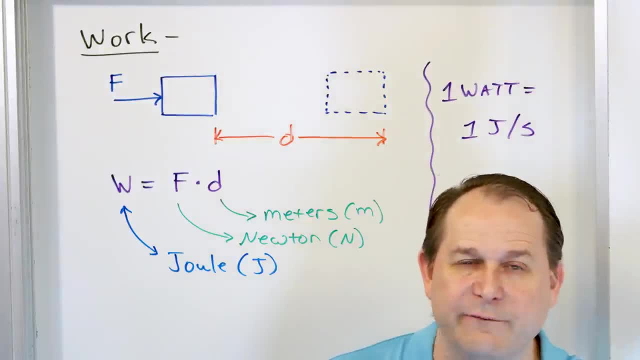 this little example I wrote: I drew the force acting in the direction of motion, So it's just a multiplication. But I just want you to know that if the force is acting in the direction of motion, if the force is at an angle or something else weird is happening, then you need to basically: 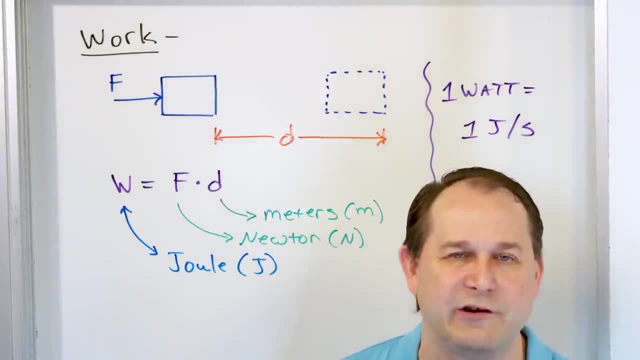 calculate the percent or the amount of force in the direction of motion. That's all that matters for the work. So basically, when I move a box, the amount of work that I do on that box is only related to how much force I push in the direction that the box moves, multiplied by how far the box 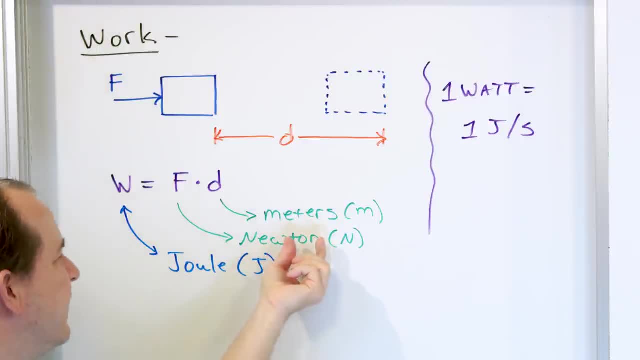 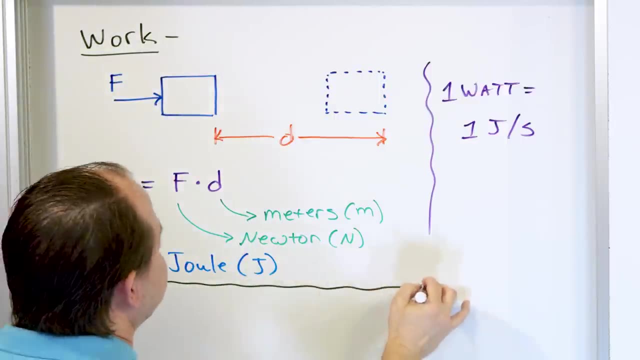 moves in newtons or in meters, and then times newtons and you get a unit called joules. All right, so that is one third of what we really need to cover. This is the concept of work. Now we need to cover the concept of potential energy, which we talked. 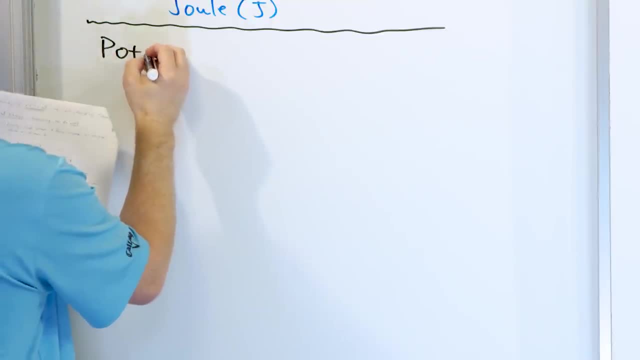 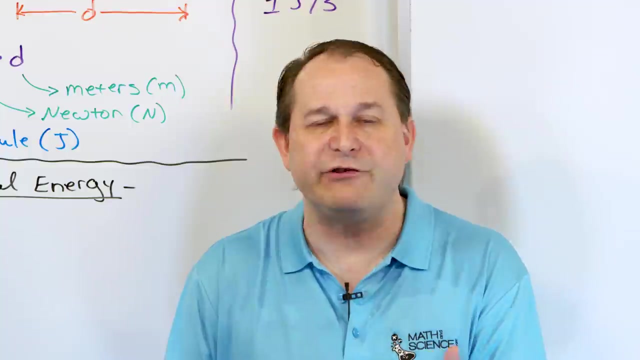 about, but we're going to talk a little more about it here now. So, potential energy, All right, potential energy. We already gave kind of an intro here, and the intro was essentially that potential energy is the potential to do work. That's literally the definition. 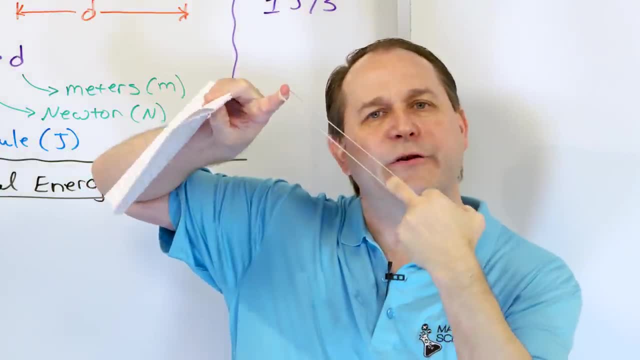 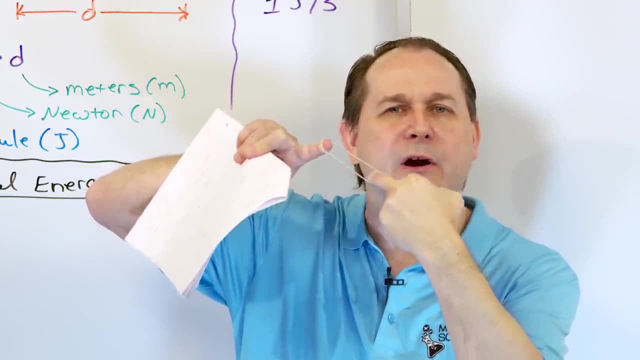 the capacity to do work. This rubber band is exerting a force on my fingers And because of that, if I were to work with a rubber band, I would be able to do work with a rubber band If I were to let it act, if I were to let that force act on my fingers and pull them together. 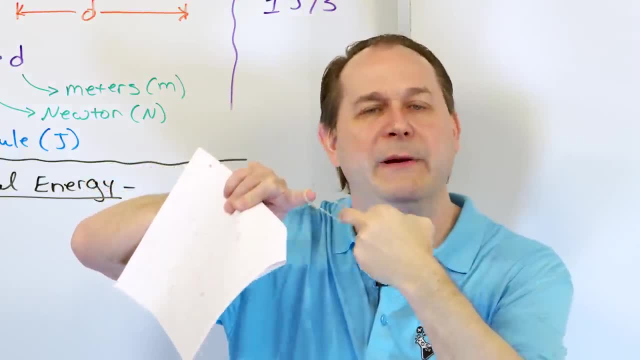 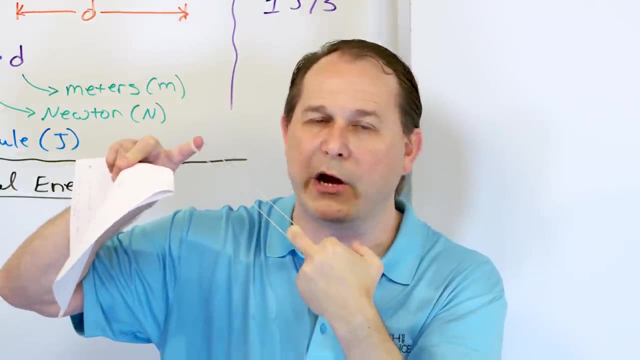 then there is a force and there's a distance, my fingers moving, and so work is being done on my fingers, right By the force, basically by the molecules inside of this rubber band, the forces that are going on in there, right. So potential energy is when things are not moving. I have the 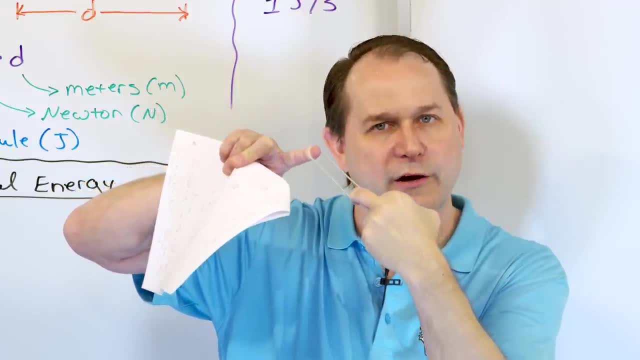 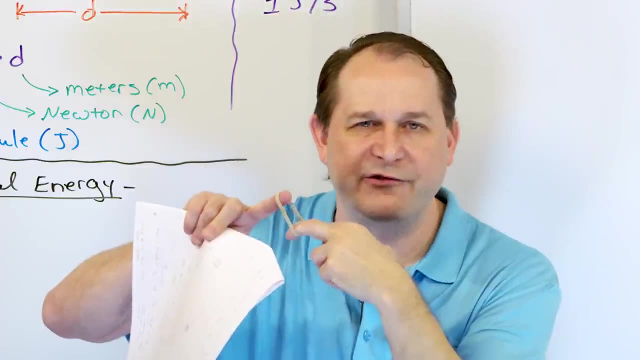 potential to do work. When things start moving, then I'm doing work, Even whenever I get down to the point where my fingers aren't moving anymore. now I'm in a relaxed state. the force has done its act on my fingers. my fingers have moved through a distance and I've basically converted the 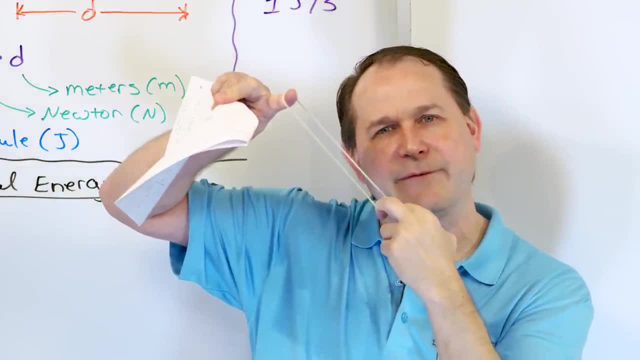 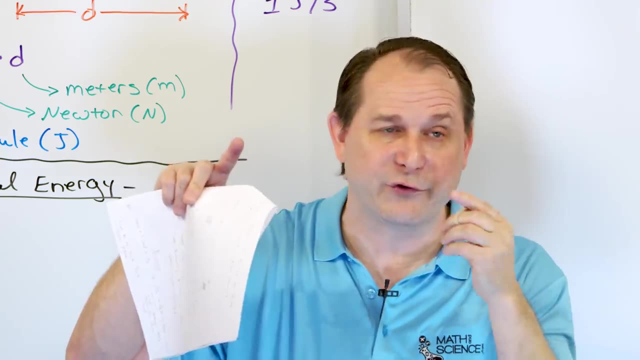 potential energy, which was very high in the beginning. I've converted it as my fingers have now stopped. I've converted it into work because my fingers have now moved through a distance by a force. So you see how they're tied together. The potential energy is what's happening before the 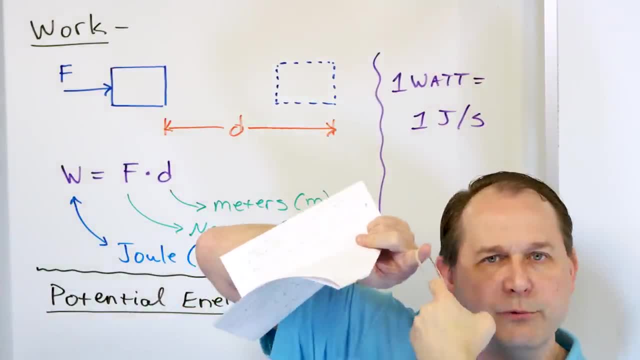 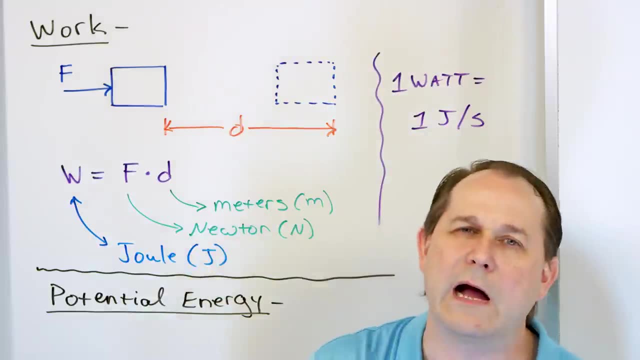 motion happens As the motion happens. you see, my fingers are no longer moving anymore, so you would think nothing's happening, but what's really happened is the potential energy that I had is converted into work. That's why the units of all these things are the same. They're just sort of 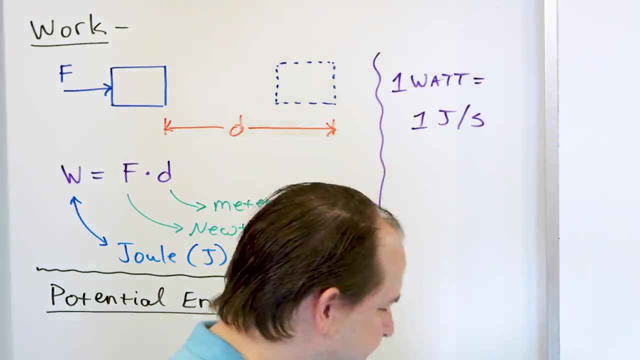 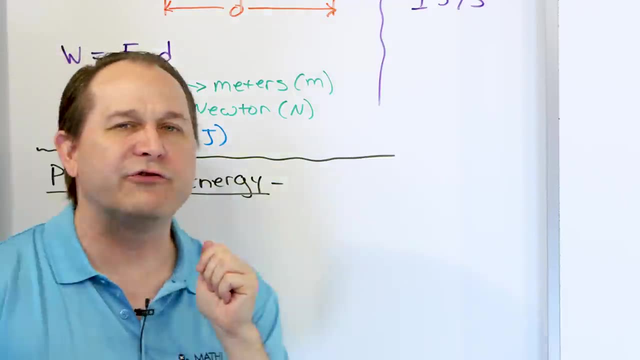 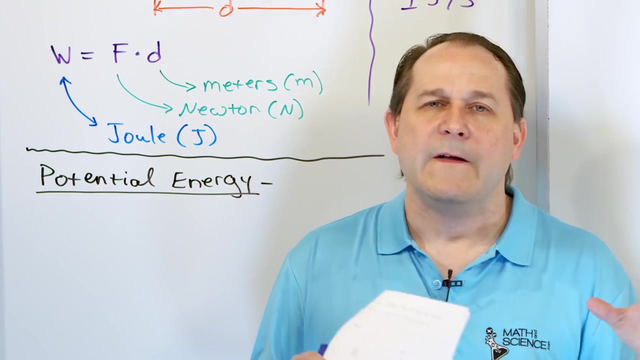 different ways of thinking about the same thing, as the process happens. Now I've talked about rubber bands. Rubber bands are great, but in the discussion of potential energy, I want to transition to talking about gravity, because it's actually much more closely aligned to the electric force. So in 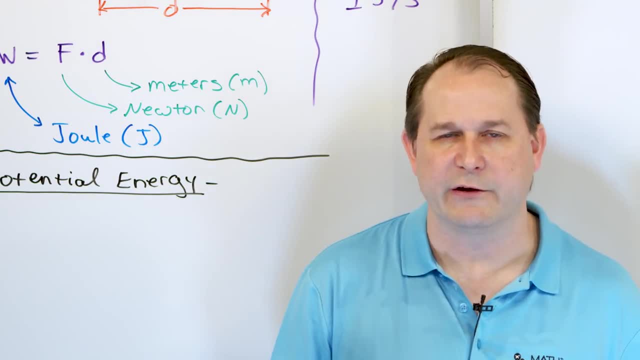 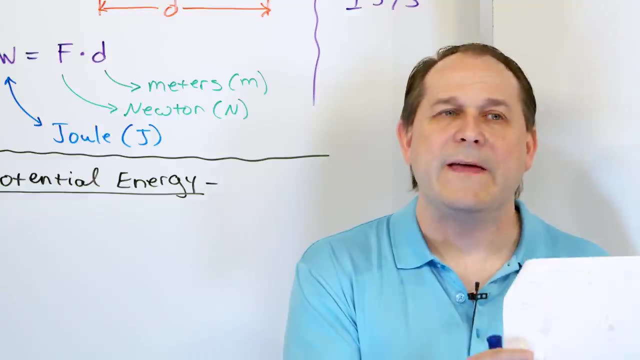 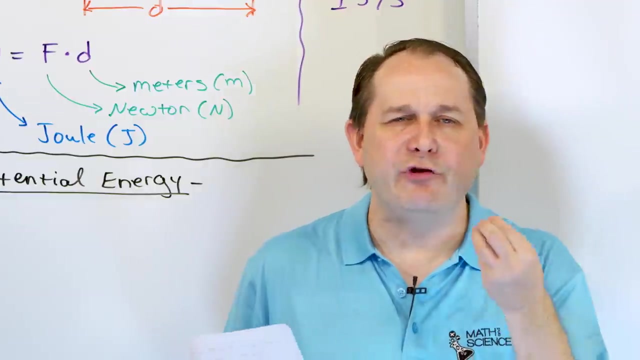 the electric force. you have electrons and protons attracting or repelling each other. Actually, the electric force is very, very similar to the force of gravity. We all have an intuitive feel for gravity and energy with gravity. So we're going to use that because we're going to use that with our 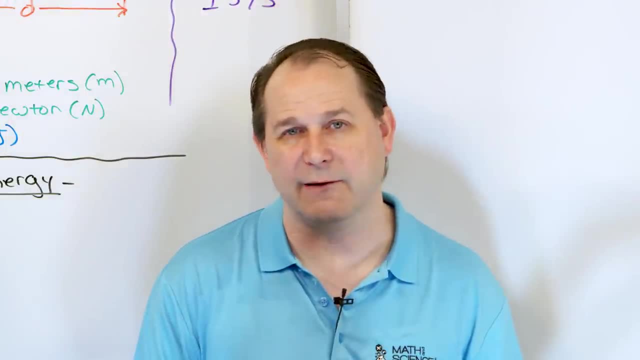 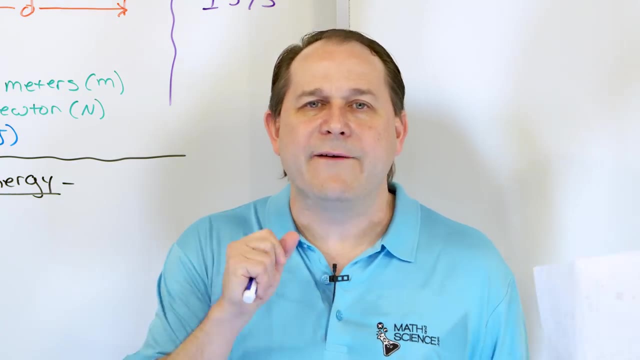 everyday experience to help us translate to what's maybe happening at the atomic level. So let me ask you a question. I'm standing on the ground right now. If I had the situation of me standing on the ground right now and compare it to the situation where I climb up on a ladder or on the top of a 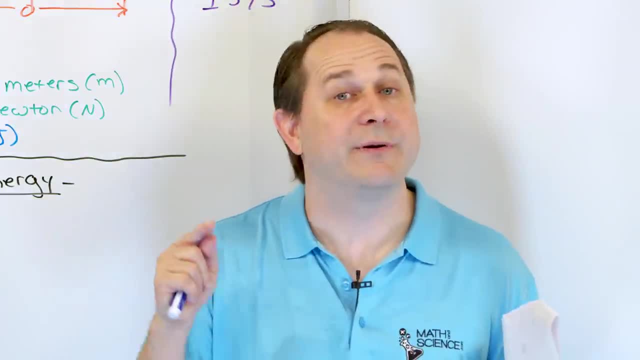 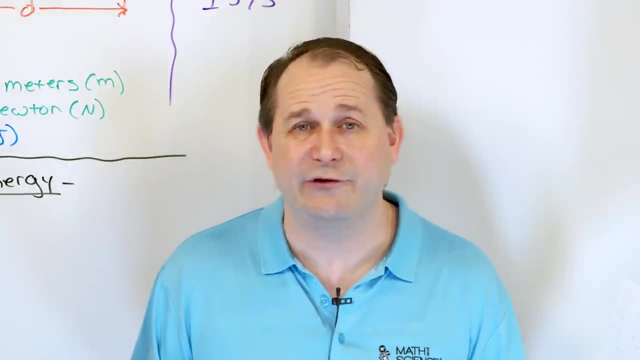 very tall building. which of those situations would have higher potential energy? Well, right now I'm at ground level. I really can't fall, I can't really hurt myself, So I have a low potential. Maybe I even have zero potential energy because I can't really do it. I guess I could crush. 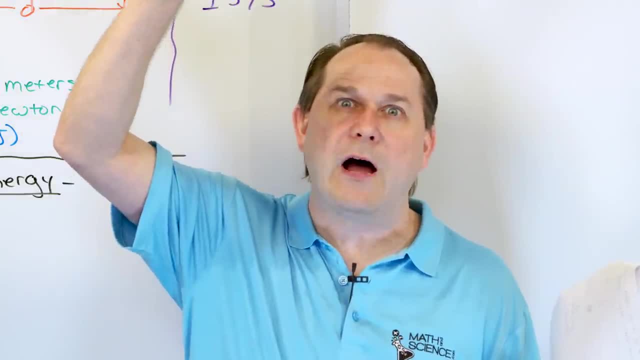 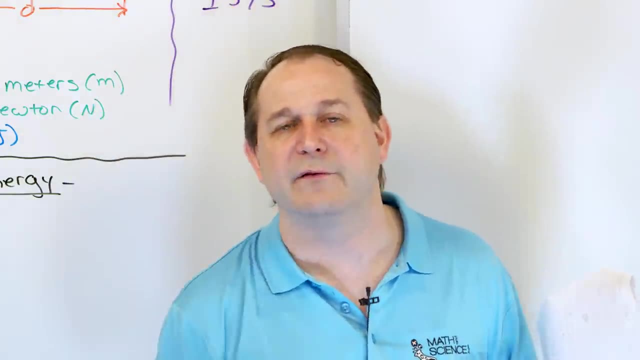 myself to the ground, but that's it. But if I'm at the top of a building and jump off, then I have a very large potential energy right before I jump, because if I were to jump, I can convert all of that into motion, And so I have a high potential energy the higher I am above the ground. 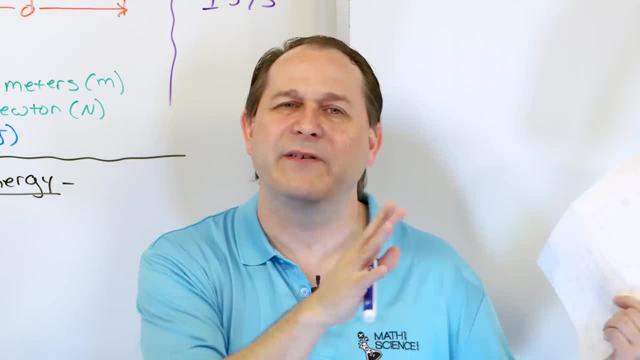 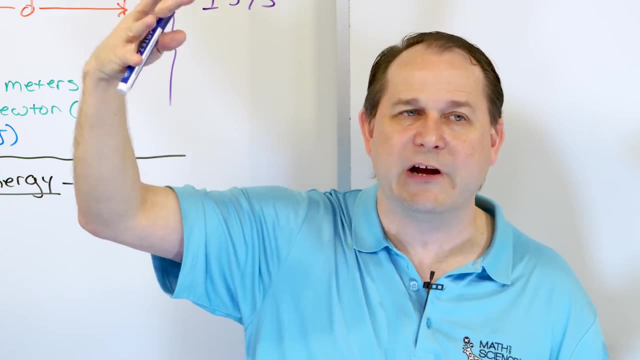 And I keep saying like this, I'm trying to drill it in your mind, because we have the same thing happening with electrons. Electrons that are far away from an atom, far away from the nucleus, have a higher potential energy, because those electrons can come crashing down through the 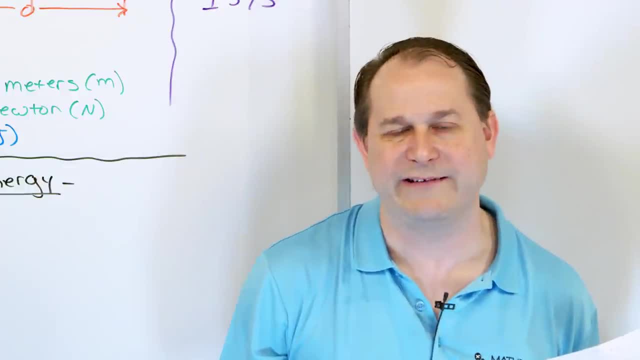 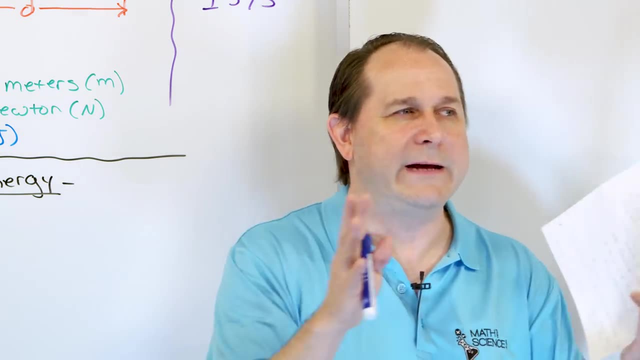 attractive force, with the nucleus crashing down into a lower energy state, And that happens all the time in chemistry, Like literally every chemical reaction is involving that kind of stuff. So we're going to use that, We're going to use gravity as a kind of like an analogy with what's happening with electrons. 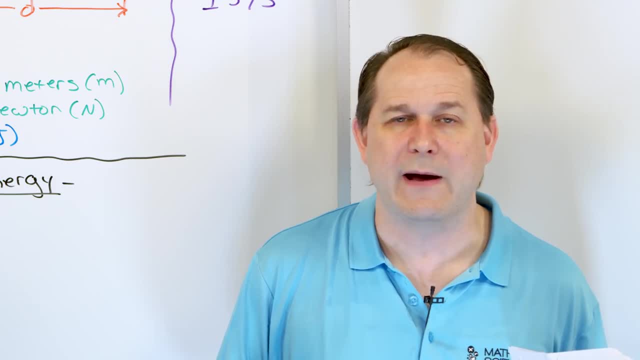 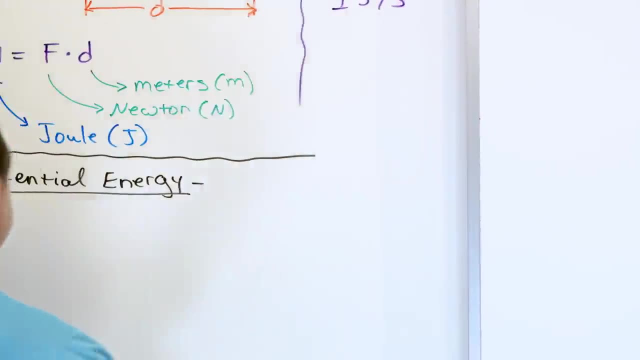 So the higher up you are on the ladder, the more potential energy you have. The higher up an electron is away from an atom, the higher the potential energy that electron has. So let's go over here and talk about this. We have this situation. We have really two situations. Here is 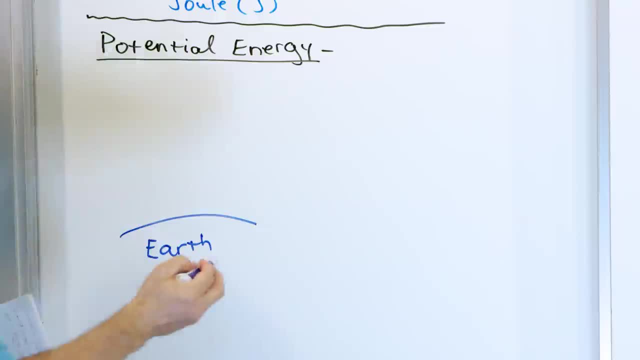 Earth right And we're going to have another situation over here I'm going to draw, which is also Earth right. It's basically the same situation that I, kind of like verbally, asked you about just a second ago. So let's talk about situation number one. Here is a 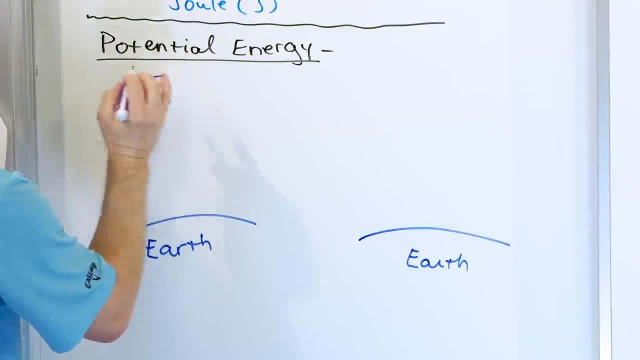 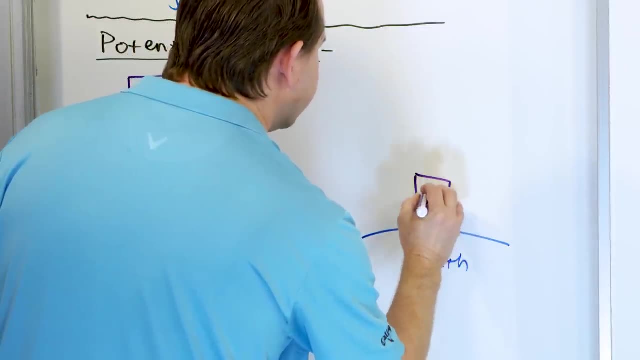 box. I'm going to put it right here: This box is some mass M, right. And then I'm going to have another situation where it's right here, closer to the ground, Another mass M. The mass of this box is exactly the same as the mass of this box. It's like, I don't know, five kilograms or whatever. 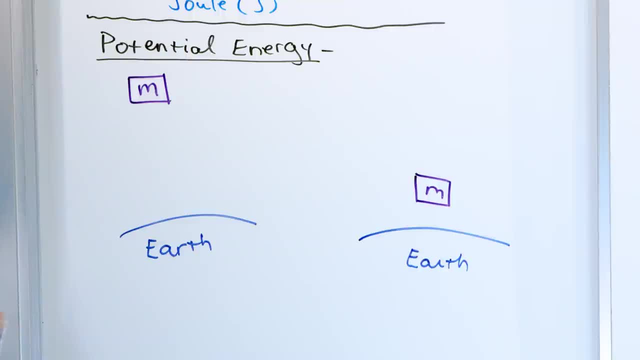 it is 10 kilograms, right. Which of these has the higher potential energy? We already talked about it. This one has a higher potential energy because if I let it go, it's going to come crashing down with a higher speed and impact the ground, And if I let this one go, it's also going to 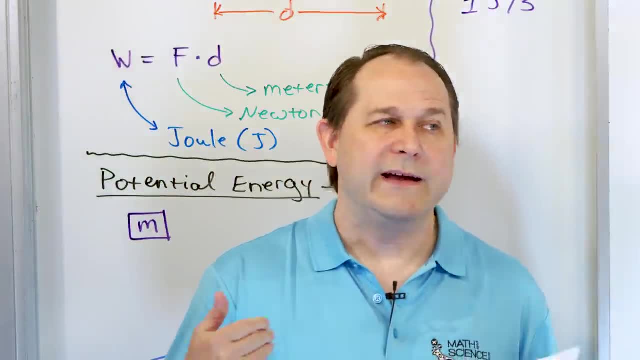 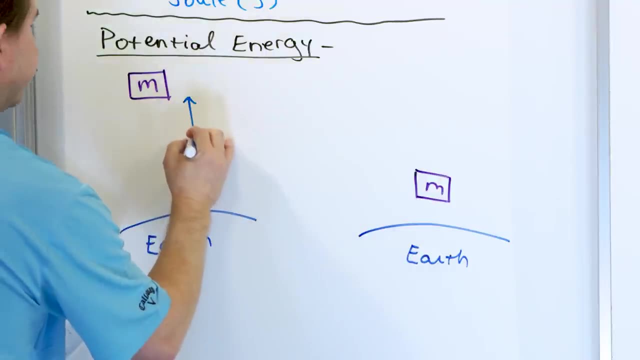 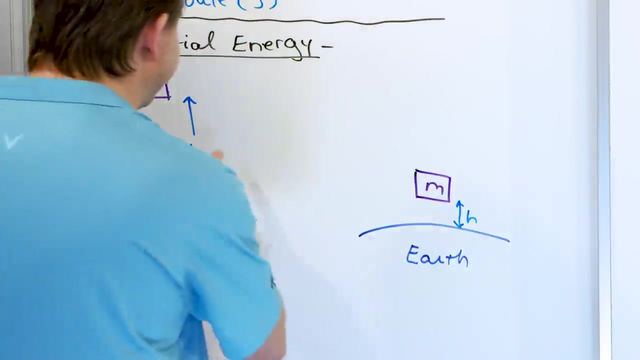 hit the ground, but it's not going to be traveling as fast, So it didn't have as much potential energy to begin with. So to continue filling in the blanks here, this is some distance H off the ground like this, And this is some distance, also H off the ground. Of course, this H is bigger than. 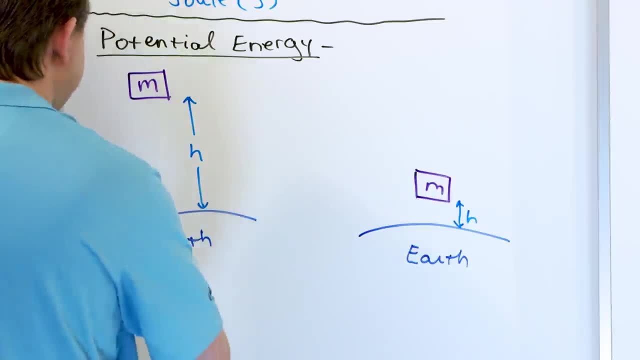 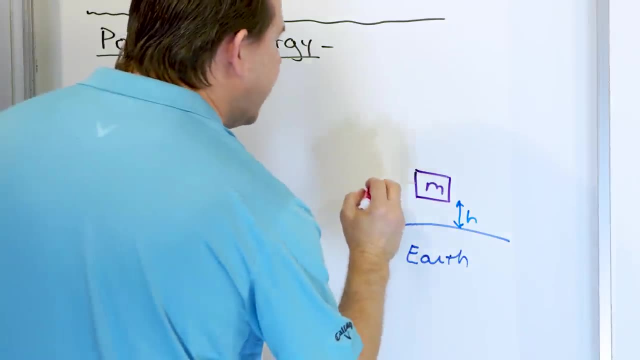 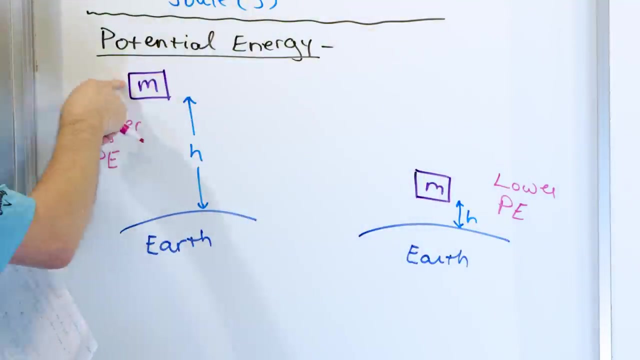 this H? all right, And we already said that this one is a higher potential energy And we already said that this one here is a lower potential energy. If we could calculate the potential energy in this situation and compare it to the potential energy in this, 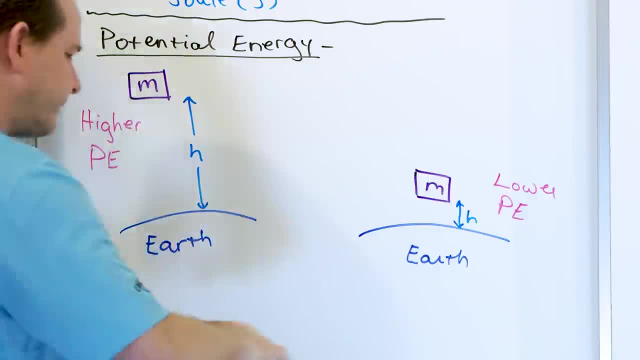 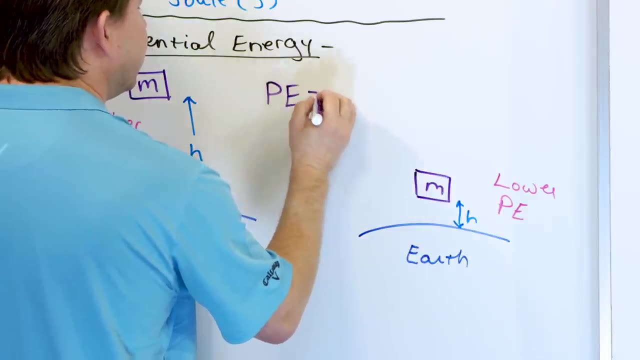 situation: this one's going to be lower and this one's going to be higher, And that's exactly what we do. So what we say is that the potential energy- and this is an equation you'll learn in physics, but we're learning it here as well- is just the mass times, the gravity, the gravitational. 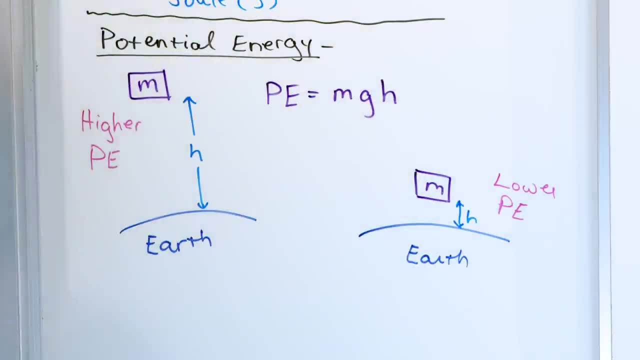 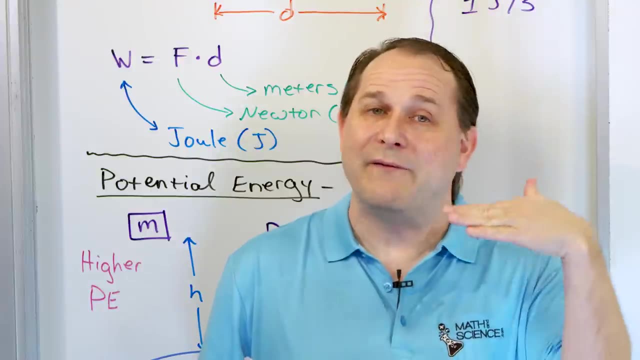 acceleration of the planet. you're on times the height of the ground And this is the mass times the height above the ground. all right, Now there's a lot of gotchas that go into this. I don't want to get into all the gotchas, but basically it assumes gravity is constant. You 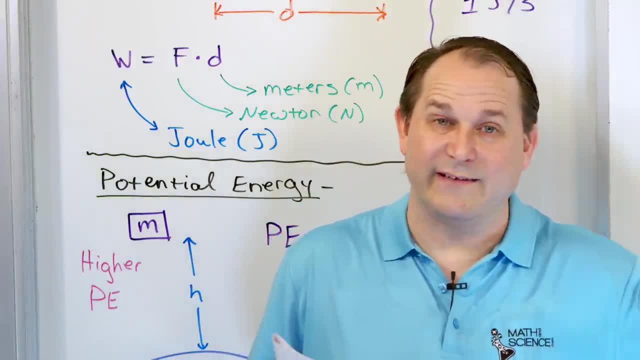 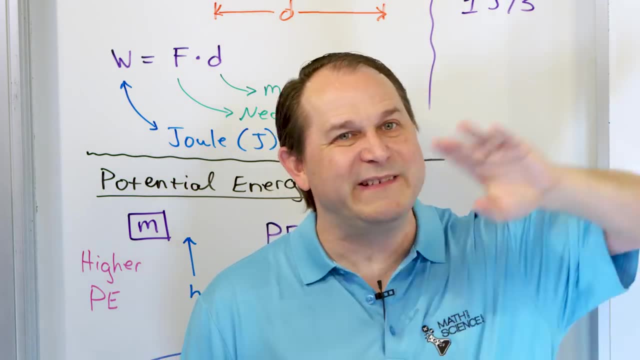 know, as you get farther away from the planet, technically, the gravitational force gets less and less. So this equation holds for everyday situations close to the surface of the Earth. But if you're in a spaceship and you move 6,000 miles that way, then yes, the gravitational force. 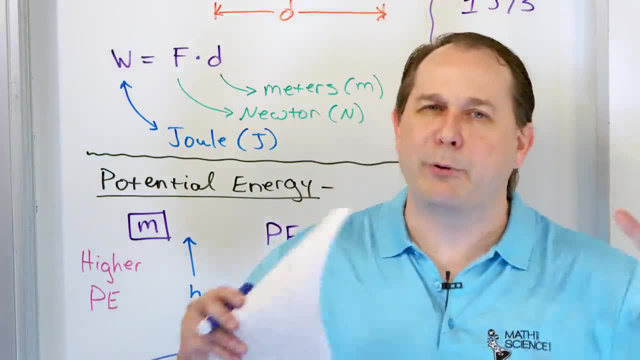 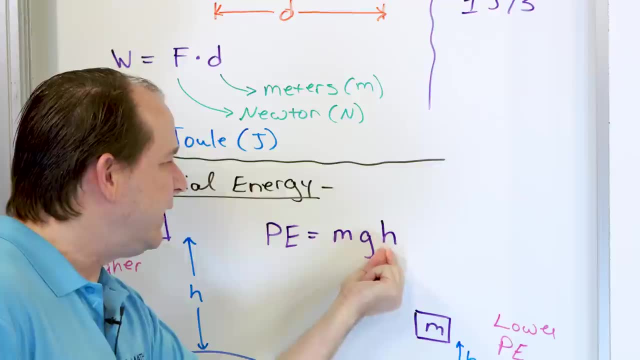 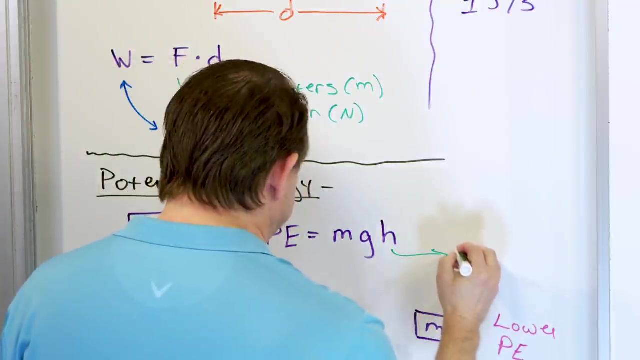 is a little different. So this equation becomes more complicated. But for the purposes of us talking about this, to understand energy, it's perfectly fine. So just say that potential energy is mass times gravity times the height. Now, what are these units here? Well, the height, you might guess, is in meters. I'm just going to put m right here. 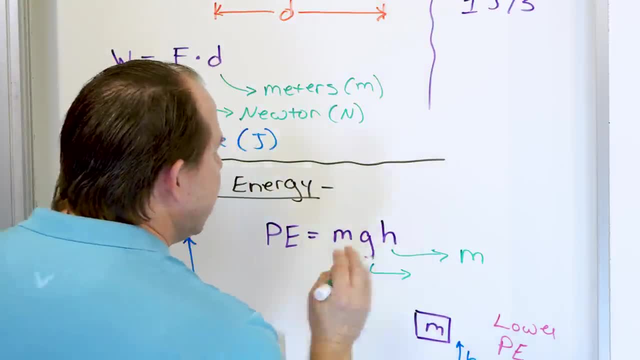 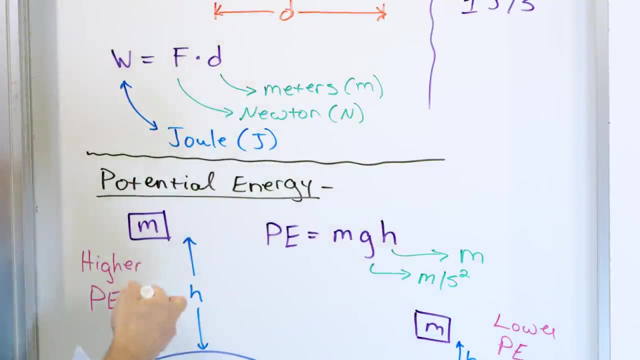 Same meters we used before And the gravity is, since this is in meters and this is the gravitational acceleration, so it's meters per second squared. Remember- you may or may not know- the units of acceleration is the units of speed or velocity is meters per second, But we're not talking about that. 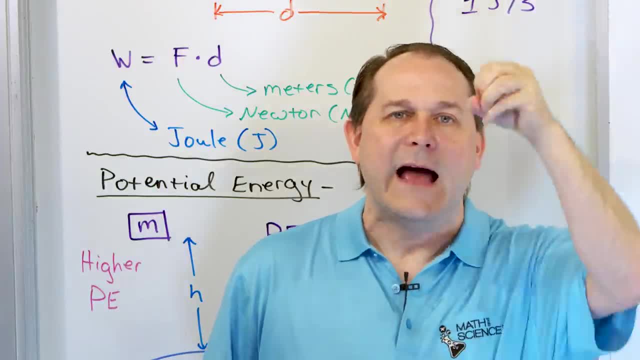 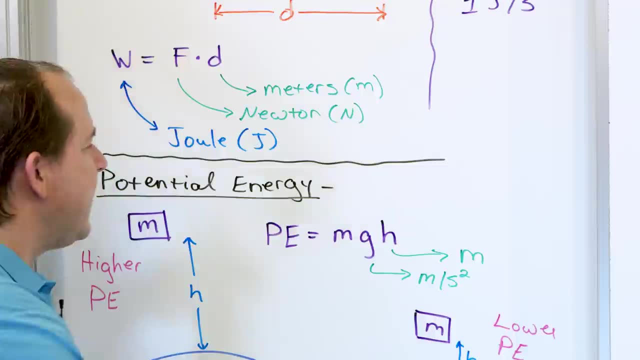 We're talking about acceleration. acceleration, How fast does something accelerate? How much does it fall if you drop it? The gravitational acceleration, that's meters per second, squared right. So that's that unit. And then this mass is in kilograms, as I told you before. I think I told you, maybe I verbally told. 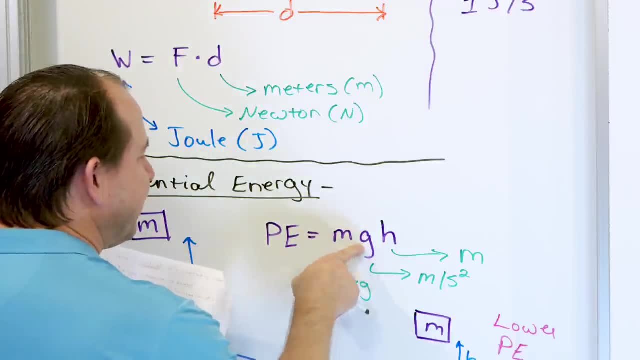 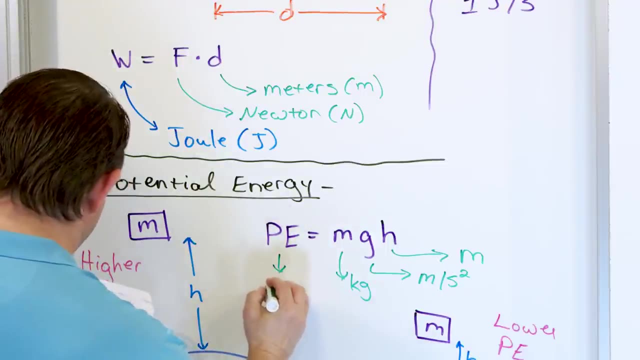 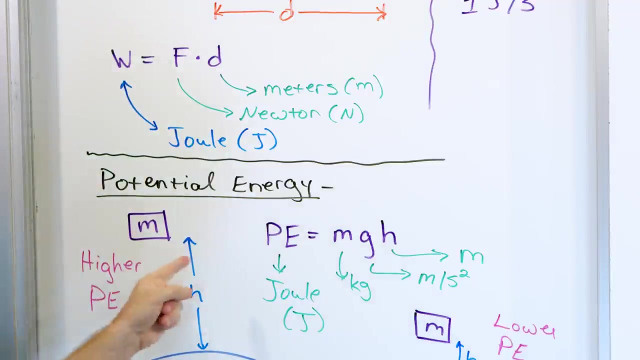 you kilograms. If you have the mass in kilograms, the gravitational constant acceleration meters per second squared and the height in meters, then what do you get for the potential energy? You also get joules. So I'll put joule, which is a unit of J. So notice that when we calculate 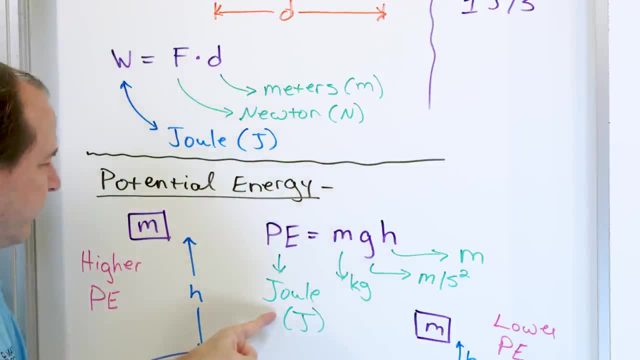 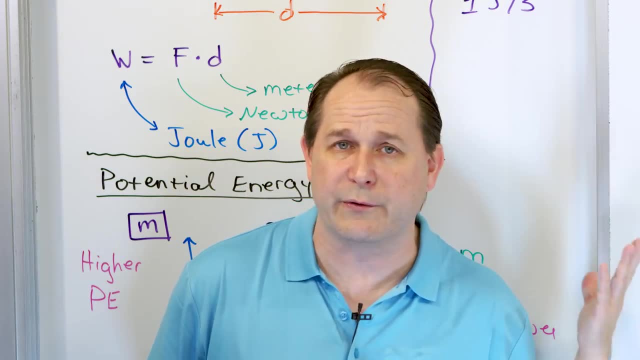 the potential energy in these situations. we get a unit of joules, assuming we use these units here. If you don't have the units given to you in the problem like this, then you convert them. There are other ways to handle it, but I would just convert them always to these basic units. 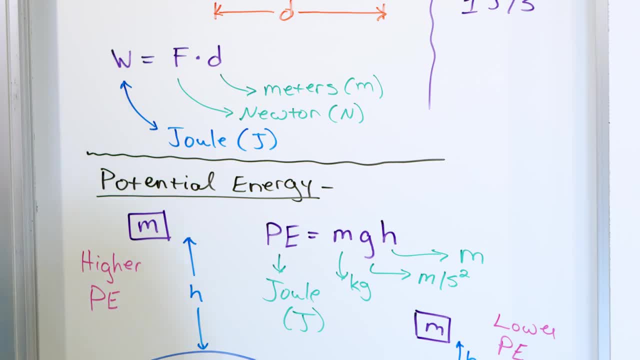 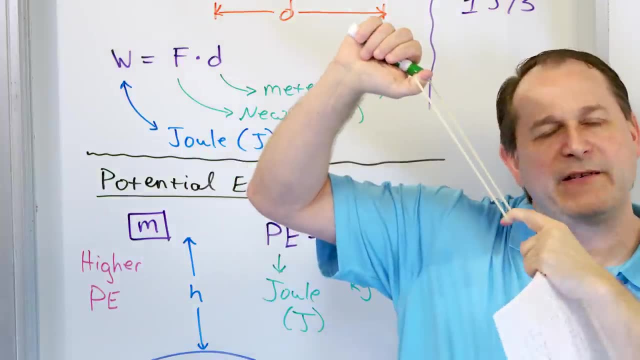 You get joules. Work is force, times, distance. You also get a unit of joule. Now, why are they the same unit? Well, it's because if you think back to the rubber band, or if you think back to this right now, the rubber band's 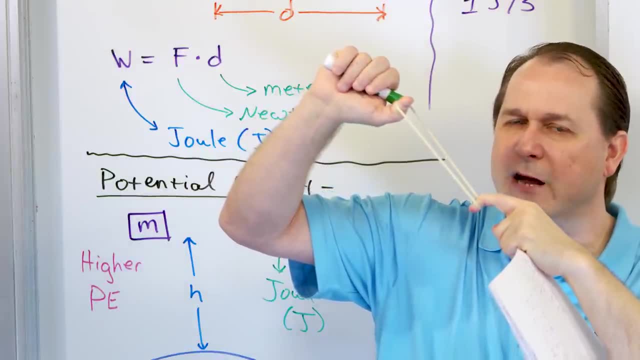 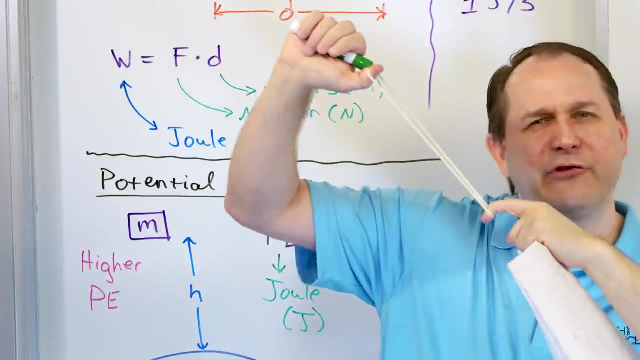 exerting a force on my fingers. If I allow my fingers to come together, the force is doing work on my fingers because it's force times distance, right, And so the potential energy I had, let's say I had 10 joules of potential energy. And then if I were to calculate force times distance, 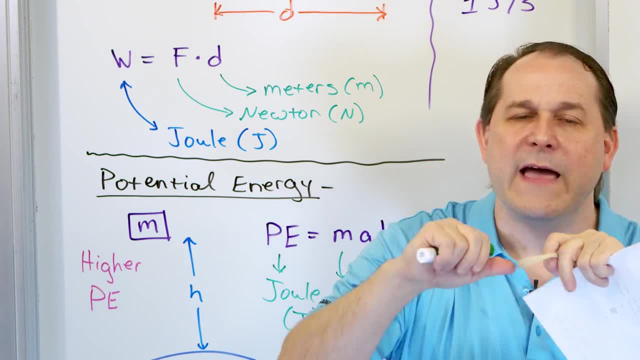 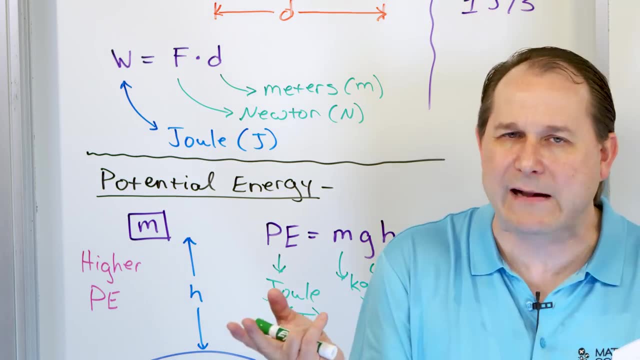 when I get to zero, maybe I've done 10 joules of work, And so the 10 joules of potential energy got converted into the energy of work, which is essentially the 10 joules. So everything balances. You have to have conservation of energy. all right Now. 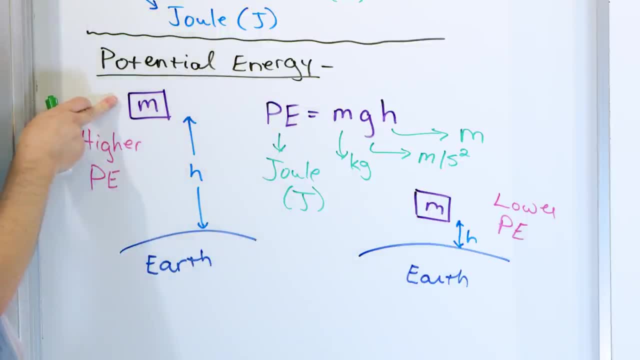 if you want to think about it in terms of gravity, here you have a higher potential energy, maybe 10 joules or 100 joules, m times g, times h, And then, whenever you're at a lower distance off the ground, you have a smaller potential energy, And this just basically means that, if I let it go, 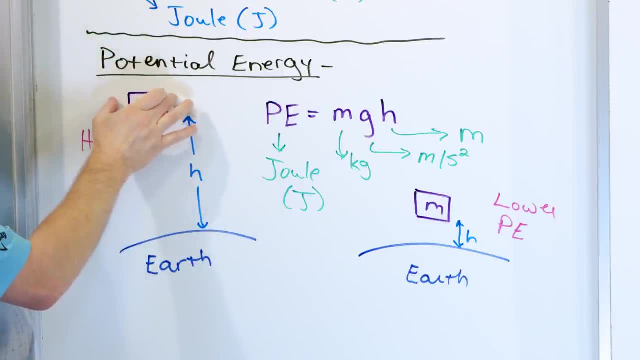 then you're going to have a higher motion, higher energy conversion from potential energy to energy when you hit the ground as it speeds up, and you'll have less conversion there because you've started with lower potential energy. And again, I'm going to say it one more: 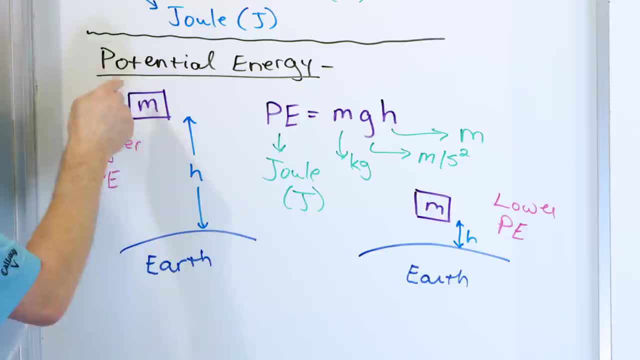 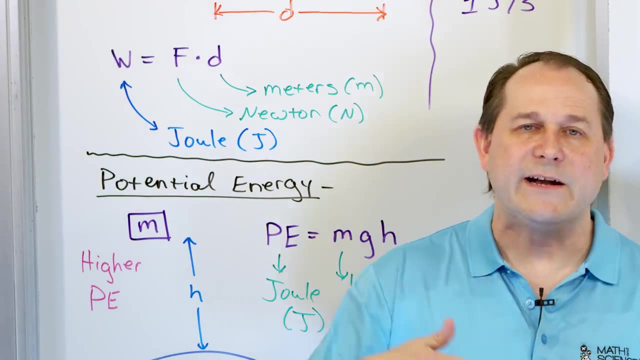 time. If you think of this being a nucleus of an atom, the higher electrons are in a higher potential energy state than the lower electrons. We actually call them energy levels. Later we'll talk about energy levels of electrons. The ones that are closer are in a lower energy level. 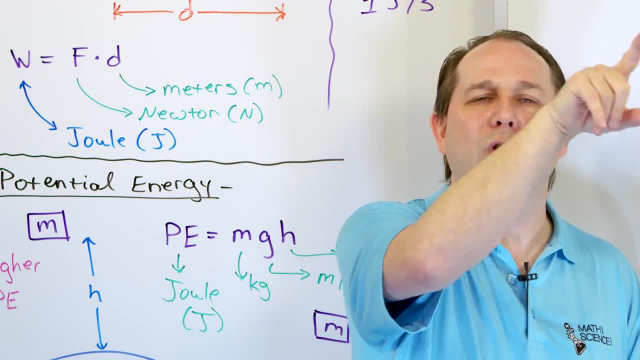 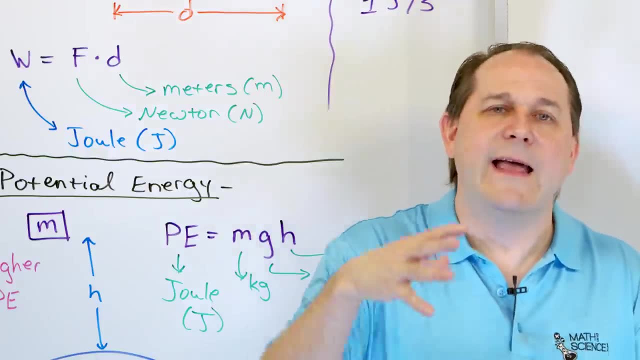 The ones that are higher are in a higher energy level. Just put the word potential in front of there. We could say the lower electrons are in a lower potential energy level and the higher electrons are in a higher potential energy level. In general, electrons like to go down to the lowest. 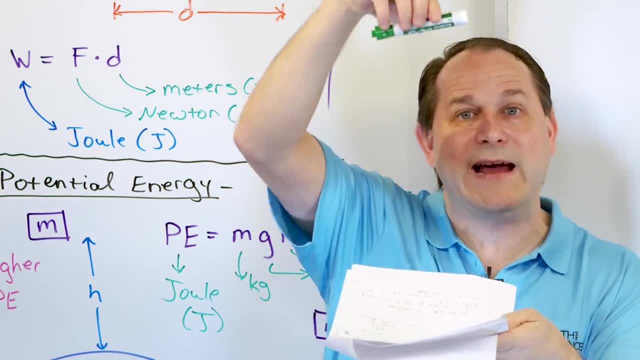 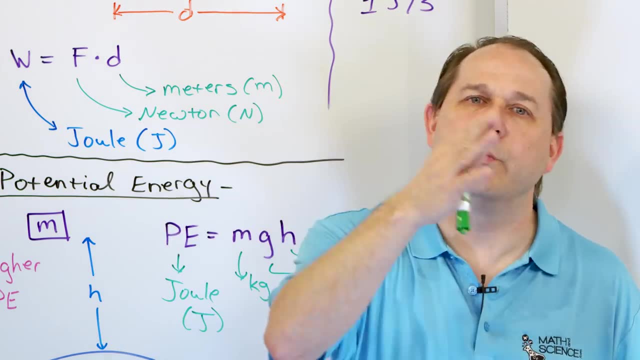 potential energy. just like when I drop this pen, it likes to go down to a lower potential energy. Throughout this class, I'm going to constantly say: nature likes to go from a high energy state to a low energy state. That's just the way the arrow of time works in our universe, In your mind. 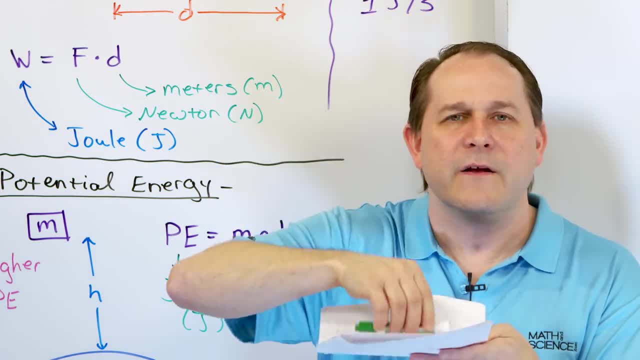 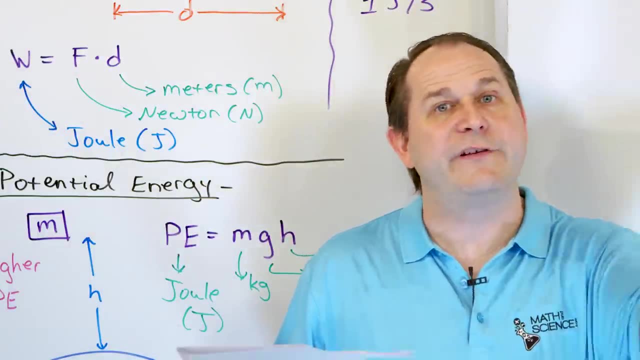 I want you to translate that as: oh, all he's saying is things like to fall down. So when you say, why do things fall down? The answer we don't really know. but the answer is because the universe likes to go from higher energy states to lower energy states. So if I hold this thing in a high 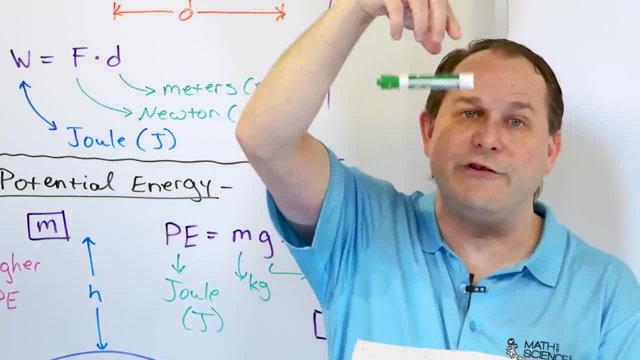 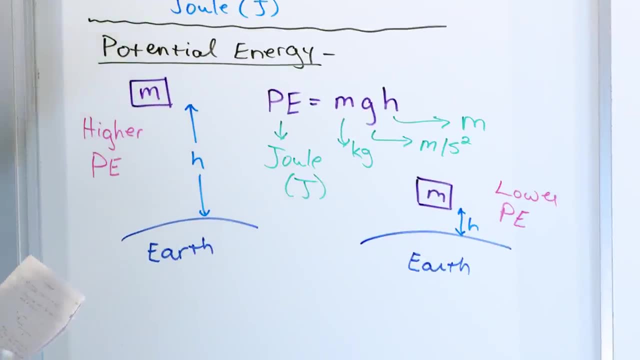 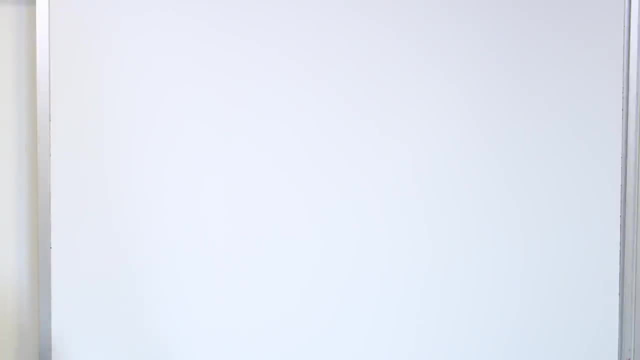 energy state, it's going to spontaneously travel to a lower energy state, because here is closer to the ground, Here is higher from the ground. So that is potential energy. Now we need to talk about the last of the important ones here, which is the kinetic energy. And actually, before I get 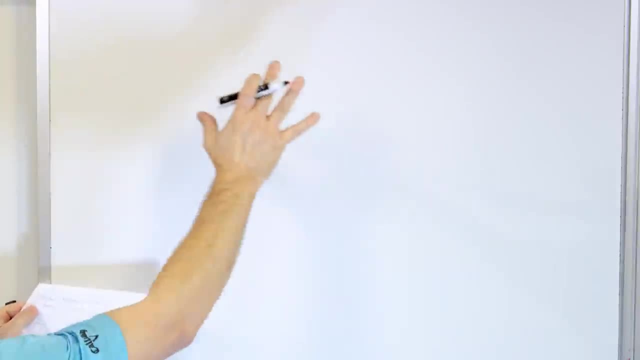 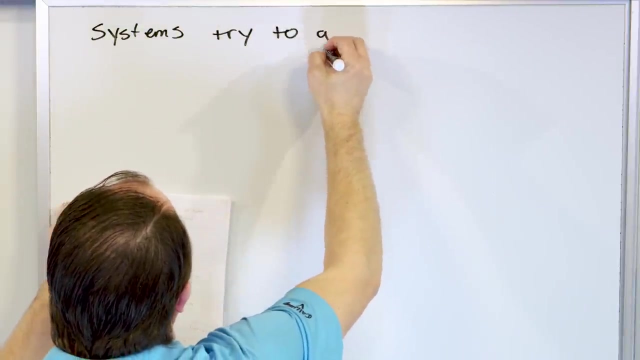 to the kinetic energy. I'm just going to tell you some things that I've said in words, but we're going to talk a little bit about chemistry on this board. I'll just say: systems, Try In general- there's always counterexamples- Generally, try to go to. 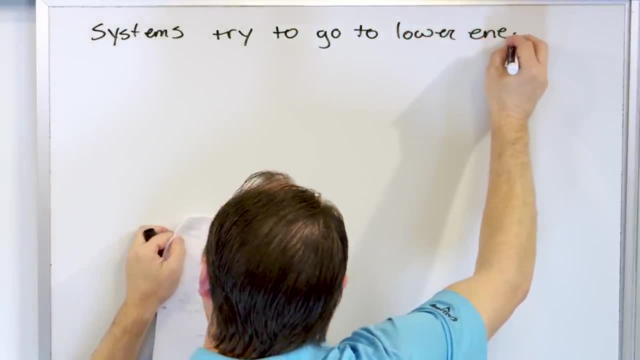 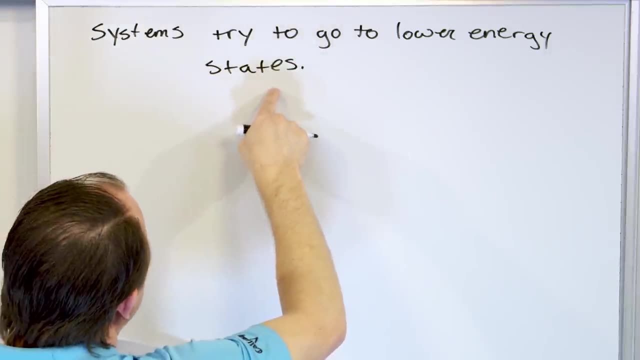 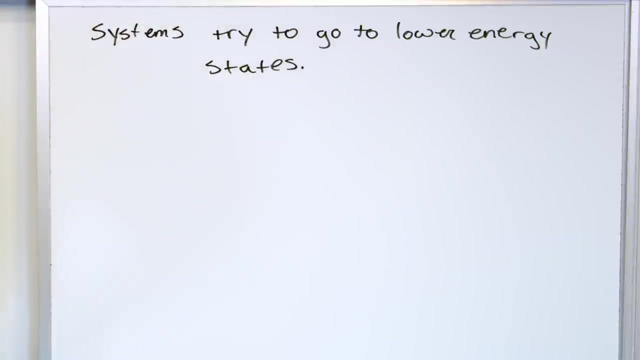 lower energy states. You can think of a roller coaster. I'm going to draw a picture. It goes up to the top, It likes to go down. It picks up speed, then goes up and slows down, then down, like this That's trying to go to a lower energy state. 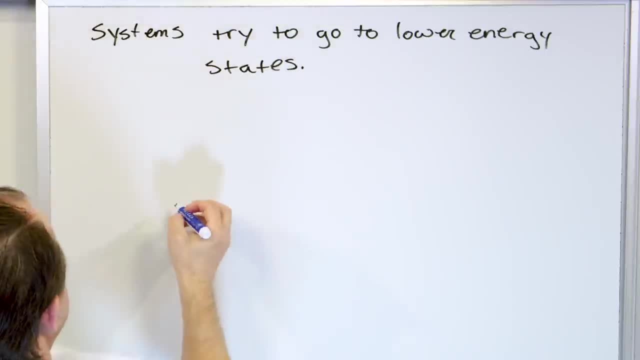 So, for instance, if I have some kind of atom here- here's a proton, here's a proton right there, here's a neutron, here's a neutron right- And I draw another atom with the same nucleus- Here's a proton, here's a proton, here's a neutron, here's a neutron. I know we haven't talked about. 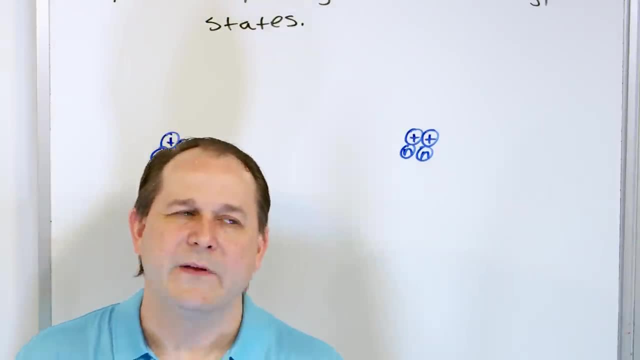 the structure of atoms. but I think you all know from fifth grade or so that the nucleus is where the positive charges are located, along with what we call neutrons, which are no charge at all, but they have mass. Those are all in a very tiny 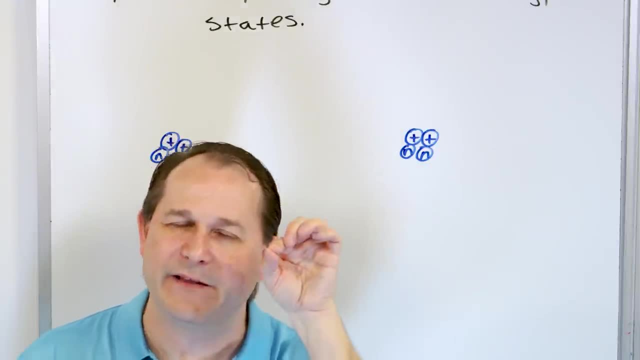 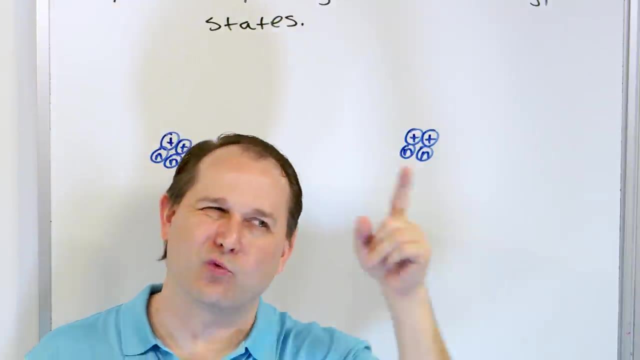 tiny. we're going to talk about how small It's. incredibly tiny part of the atom in the very center called the nucleus, And surrounding it usually we draw electrons orbiting, but we're going to talk more about that later. They don't really orbit like that. They don't really look. 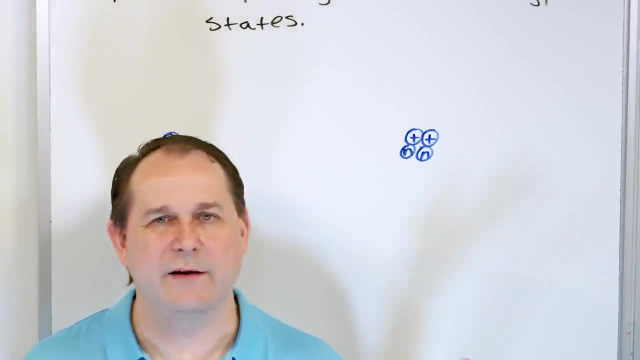 like planets. We're going to talk more about that later. Electrons, protons- they're all different than you think, but you can think about them going around them for now. So if we have an electron right here and maybe we have another electron on the other side and they're essentially in the 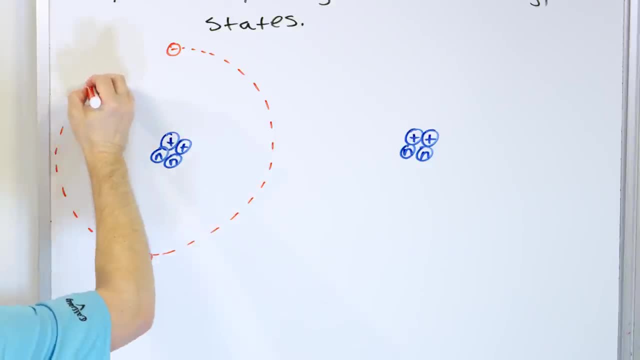 same orbit like this, which again is a neutron. So if we have an electron right here and maybe we have another electron on the other side, which again I'm telling you, right now they don't really orbit like this and we'll talk exactly why later. but this is a higher energy state than 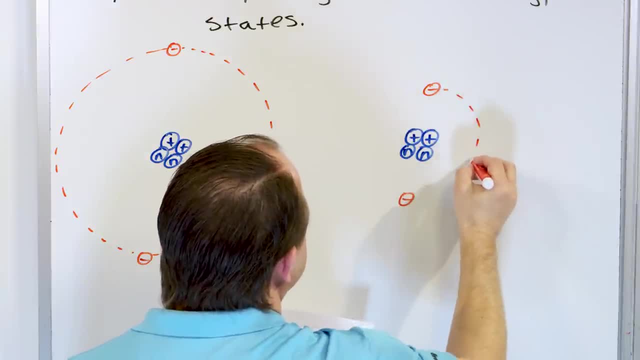 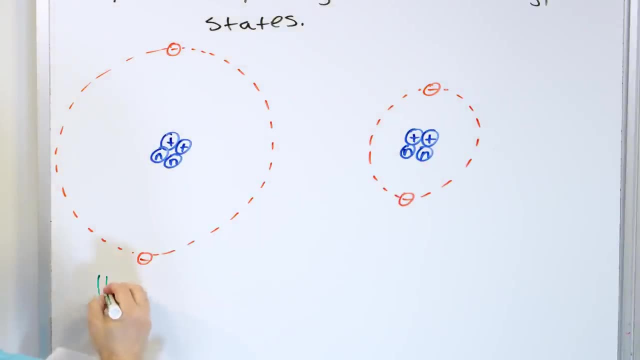 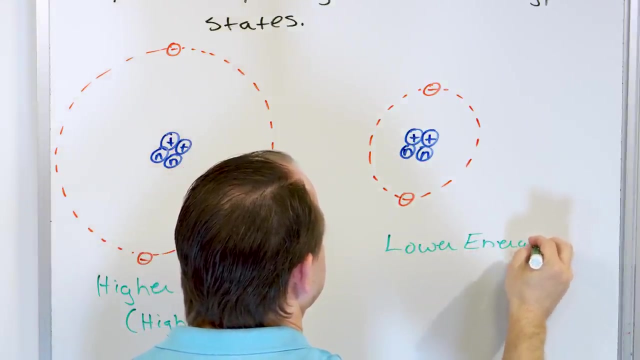 a situation like here where you have electrons that are closer to the nucleus, So this is called a higher energy state, higher energy, Whoops, if I can spell energy right, So I can say high PE, High potential energy, because they're farther away. right, And this is lower energy, Lower PE. 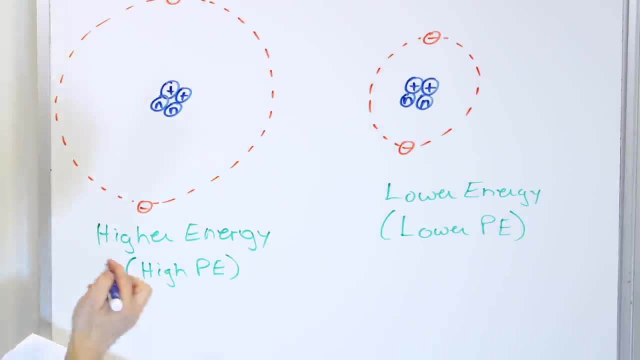 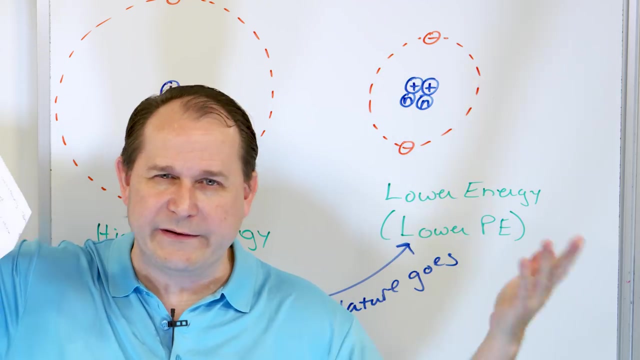 And in general, you know, system likes to go this way. So nature goes like this: from this state to this state. Not always, but because there are other situations, you know, in lasers we try to pump the electrons up to a higher energy, for reasons we'll talk about when we talk about lasers. 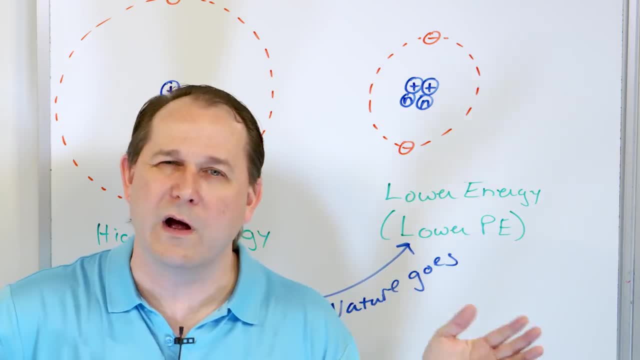 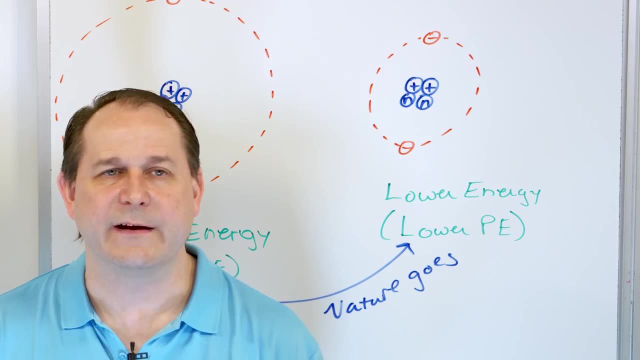 And it makes the light. if you could do that to a bunch of atoms at once, in a certain way you can make the light very focused. Sometimes we try to pump the electrons up. Sometimes we add heat to a system to get the electrons to get up to a higher energy to start then the chemical 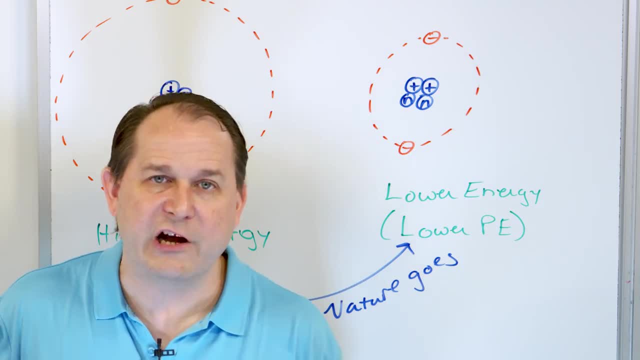 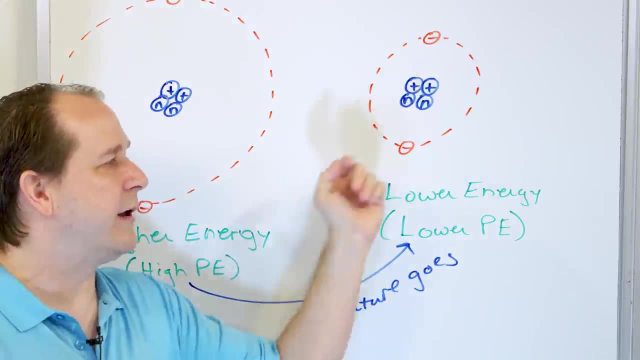 reaction can then start. There's a lot of details there, But in general is the big, big, big picture of the driving force of nature in the universe. Generally, things like to go from a high energy state to a low energy state, And so you know, we try to pump the electrons up to a higher energy. 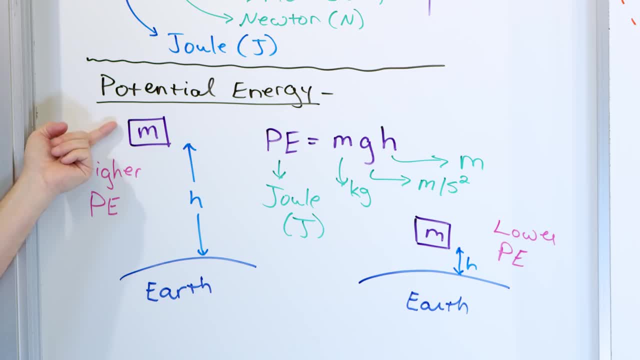 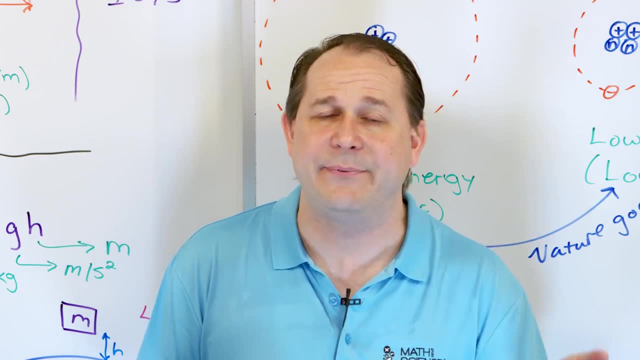 state, just like things starting from a high energy state here they spontaneously fall to a low energy state. But we don't look at atoms every day, So we don't see that. But that is what's happening to those electrons: They're trying to go to a lower energy state And that basically 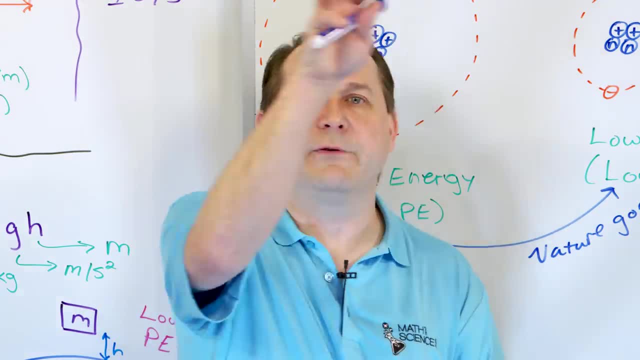 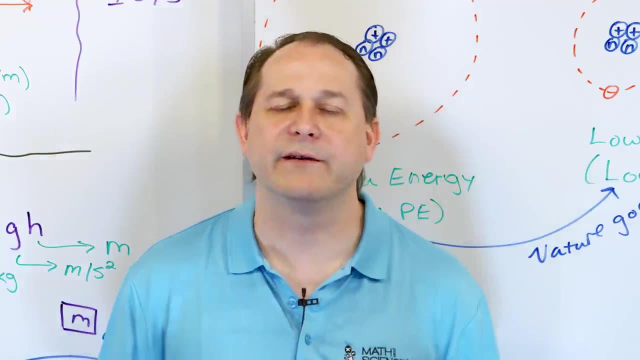 leads to chemistry, When the electrons are moving or transferred between one atom and another and then the forces are acting to pull things together and bond them. That's what we call chemistry. Breaking bonds and forming bonds is chemistry. So later on, when we talk about 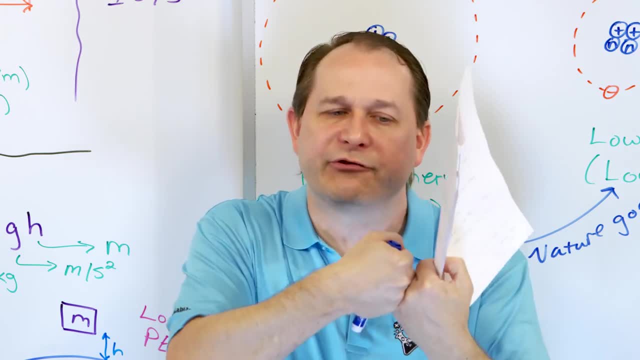 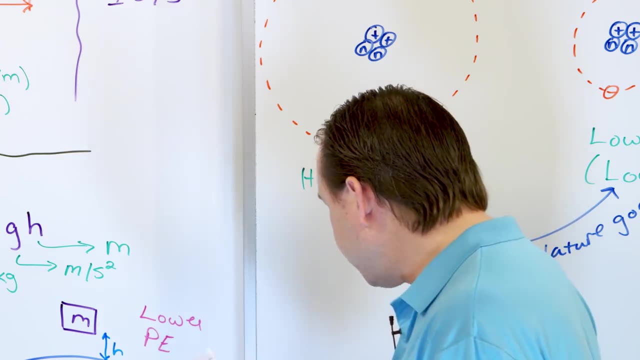 bonds we talk about, you know, two atoms coming together and sharing electrons, And then there's a force there kind of holding it together. That's a bond right. All of those forces are acting basically like this rubber band kind of force At a microscopic level. they're all pulling on. 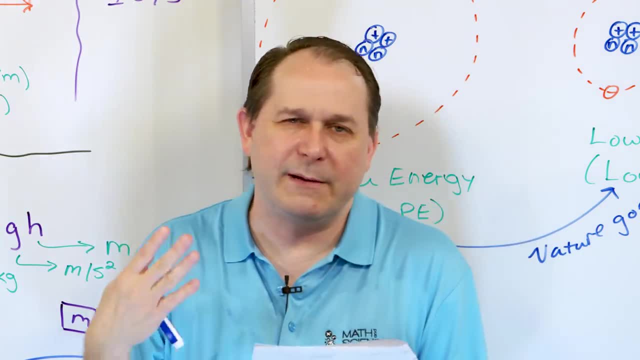 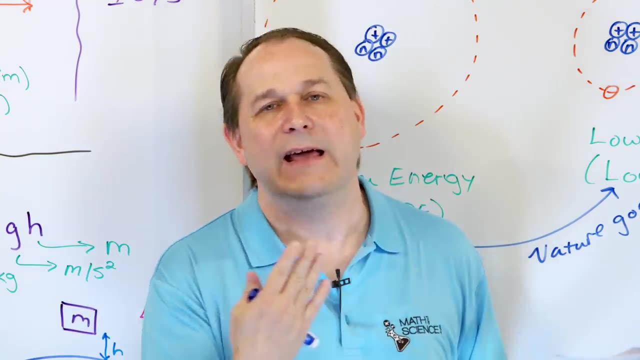 things and holding them in place. So when we in some chemical reactions, when we release heat- that's energy coming out of the reaction, Or maybe some reactions- we have to add heat. Heat is basically energy that we're adding. making things vibrate, We have to add energy. 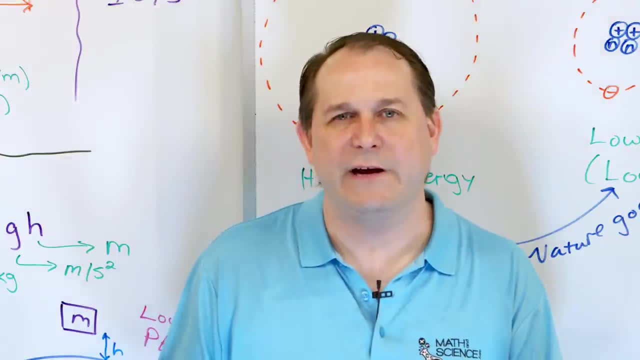 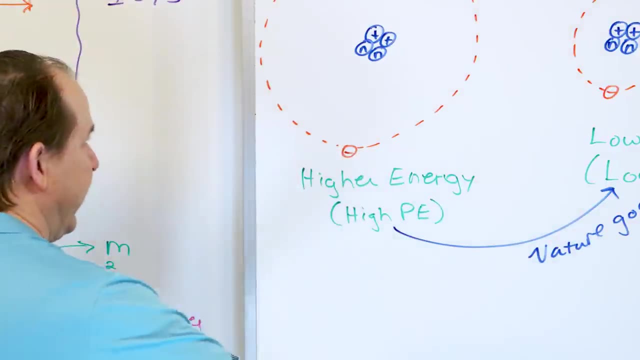 is it to the system? So all of the stuff that we're going to talk about in chemistry is very reliant on understanding these terms in physics, right? Last little example I'll leave you with before we switch over and talk about kinetic energy. Let's talk about burning. 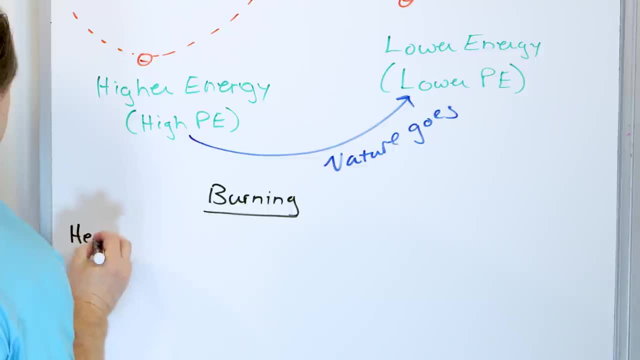 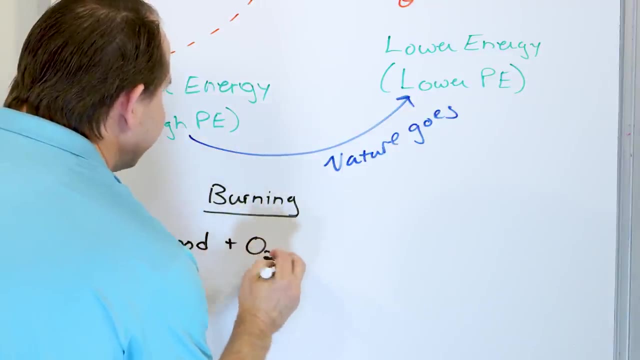 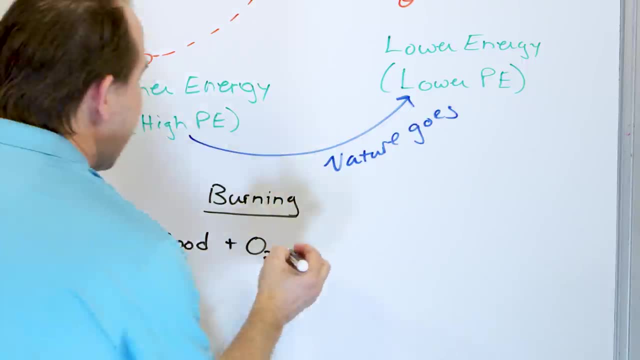 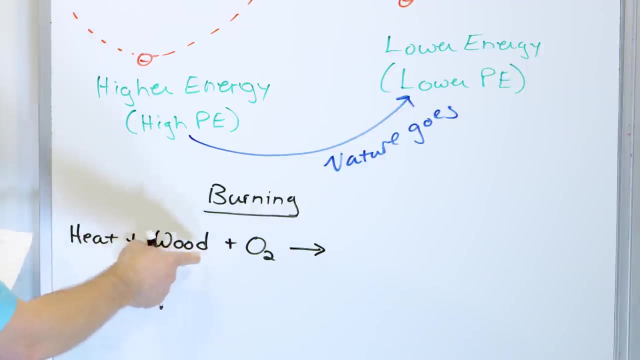 there's energy there, because it's basically bonded to itself like this. And what do you get? Because inside this wood is, you know, there's hydrogen in here, there's oxygen in here- some a little bit- and there's also a lot of carbon in here. And whenever you do all these, 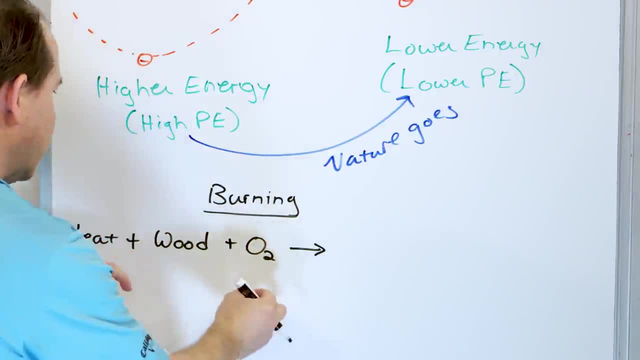 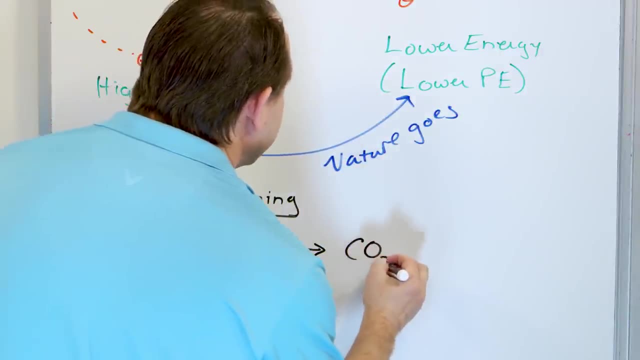 things. the some bonds are broken between the molecules. in the wood Bonds are broken to split up this oxygen. Everything gets rearranged And what do you get as a? basically, an output is CO2 plus H2O, And there could be other compounds here too. I'm not writing them all down. 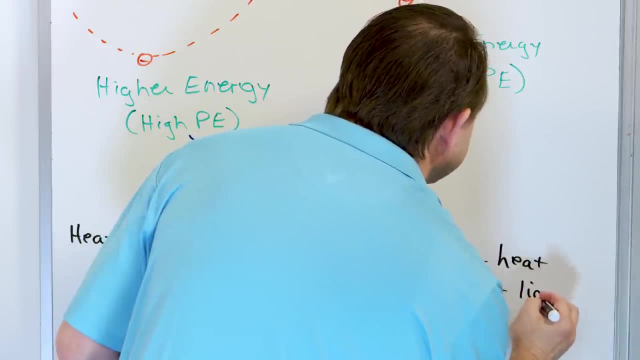 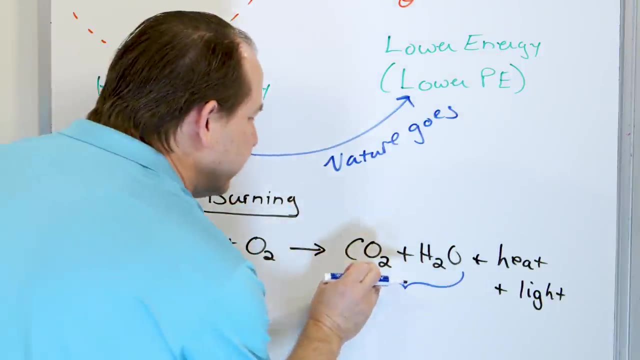 Heat comes out plus light comes out right. But I guess what I'm trying to tell you is that these molecules that are formed at the out- the CO2, the carbon dioxide and the H2O- these are in a lower energy state. 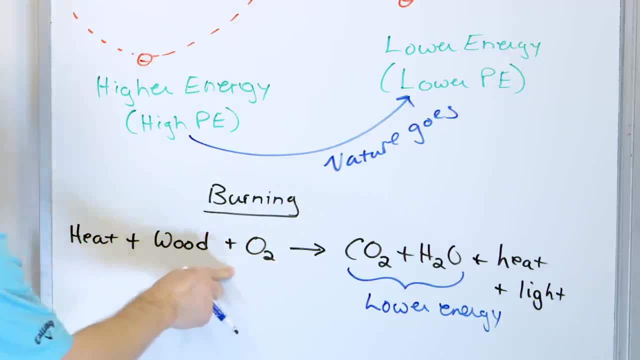 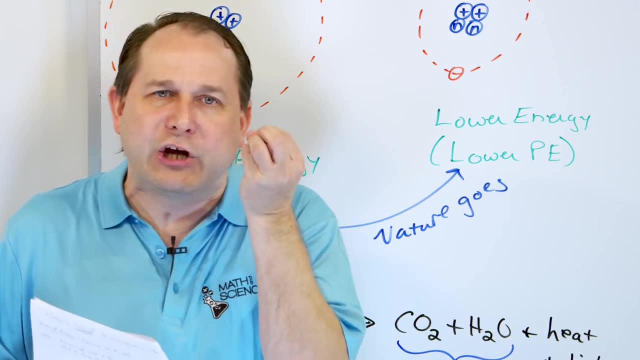 Lower energy state than what? Then the energy state of these up here? And then you say, well, what are you talking about? Lower energy state, What are you talking about? I'm saying that every molecule of this wood has carbons. 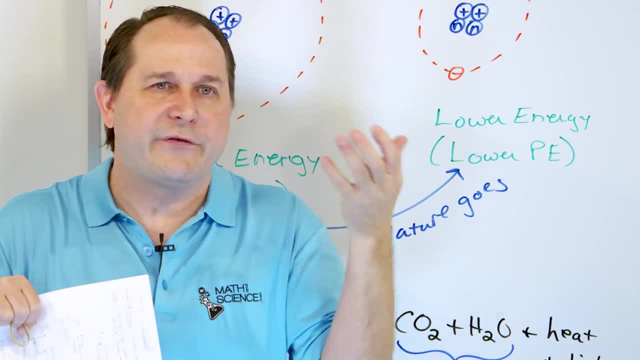 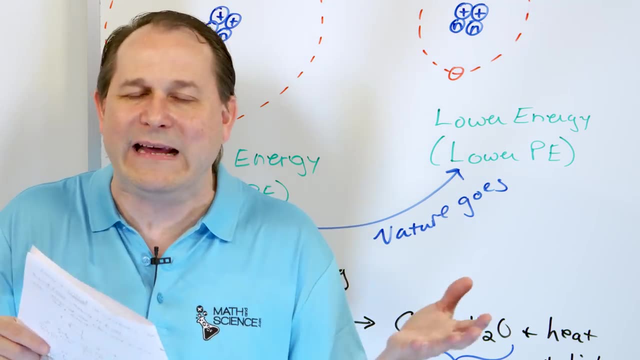 Bonded in long chains. That's what it is. When you zoom into woods, there's also hydrogen in there and there's there's a long chain. You look up what what wood is made of in the actual chemical formula of everything in there. There's long chains of organic structures there And in 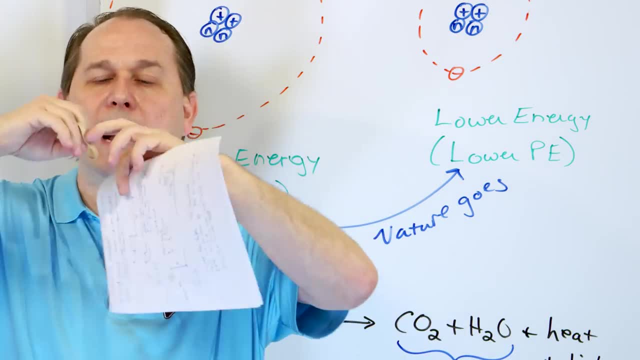 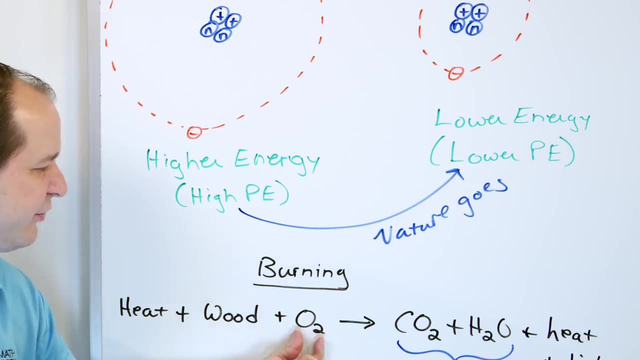 this oxygen. it's one oxygen atom bonded to another. Well, they're bonded and they're being held together by a force, just like this rubber band, that represents potential energy. There's potential energy in there because the bond between the oxygen atoms is there and it's holding them. 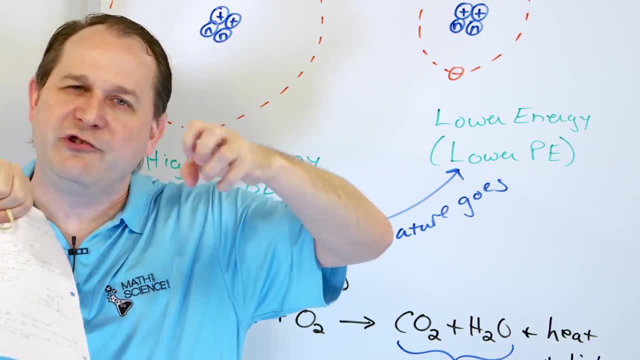 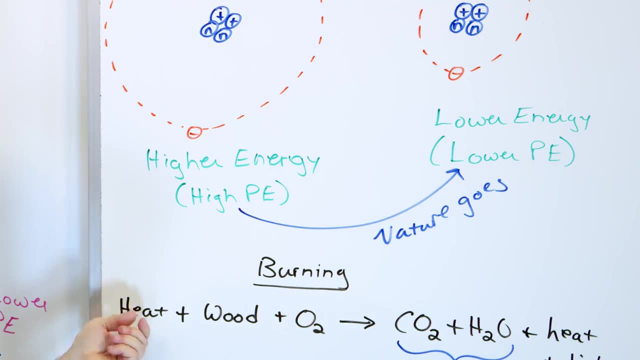 there. There's potential energy in the wood because all of the long chain of carbon and hydrogen that's there. they're also bonded. There are little rubber bands in there, right. Then you put a match to it and you give it a little bit of energy to break some of those bonds. Then you have some. 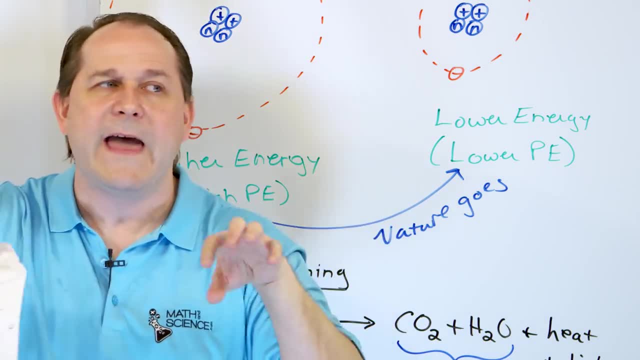 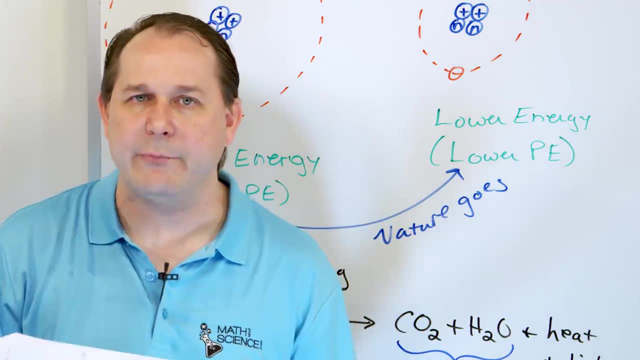 freely floating oxygen atoms not bonded anymore and freely floating carbons which come from the wood. And then what happens? They all try to recombine. And how do they recombine? Do they come back and make wood and more O2? No, they don't. Some of the hydrogen 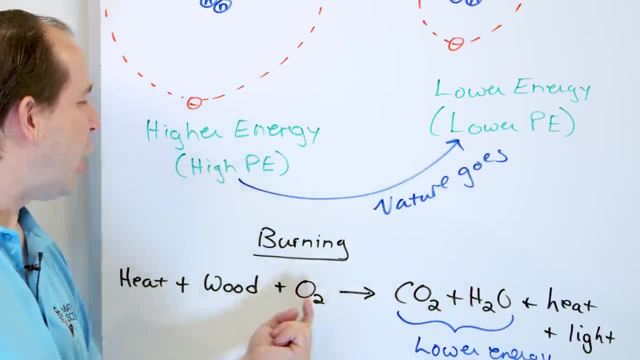 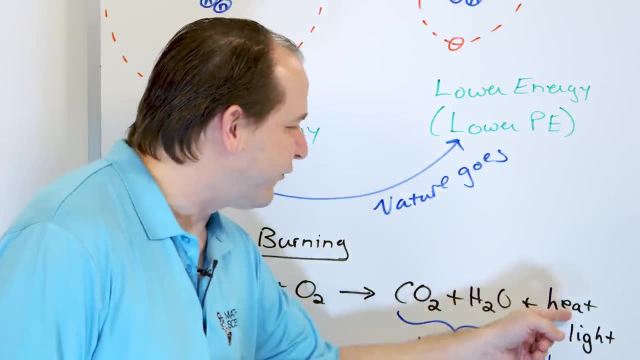 from here gets bonded to the oxygen. It makes water. Some of the carbon from the wood gets bonded to the oxygen with CO2.. And then, in addition to that, more heat is created, which is then allowing more wood to be broken down, because this heat comes back in and feeds another little. 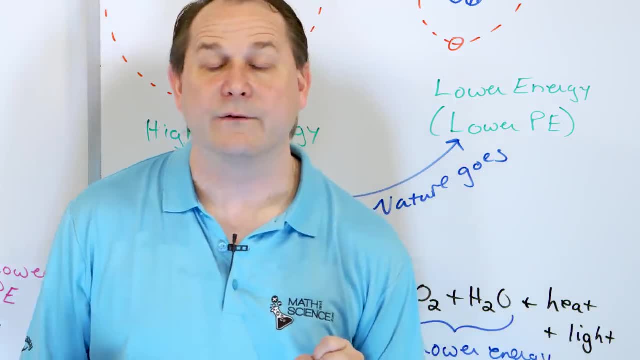 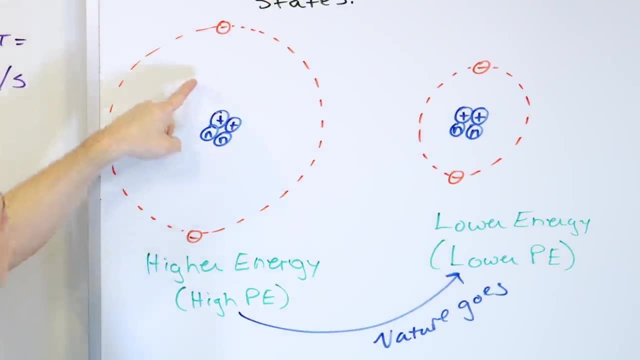 piece of wood right next door And then light comes out. And the light comes out because of the electrons moving around. When the electrons jump up and down from their orbits, like we talked about here, when an electron starts from here and goes down, it leaves the wood And then 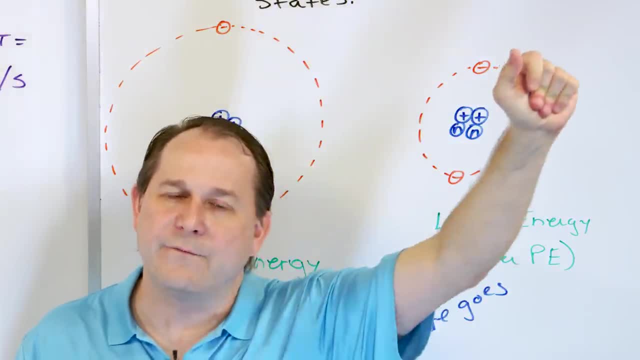 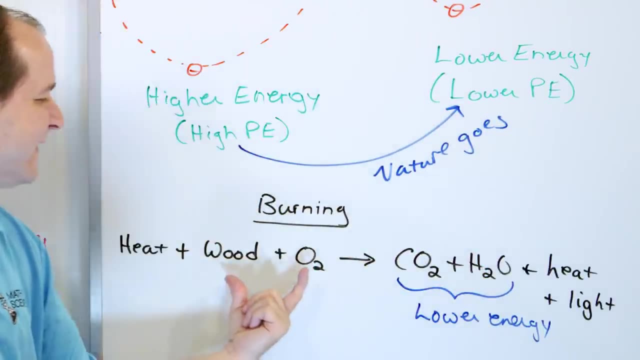 it loses energy. And what happens when it loses energy? A little photon of light comes out. We see that in a campfire- But these molecules that are formed are not the same as the ones you started with, And that's because these are in a lower energy state. What do I mean by a low energy state? 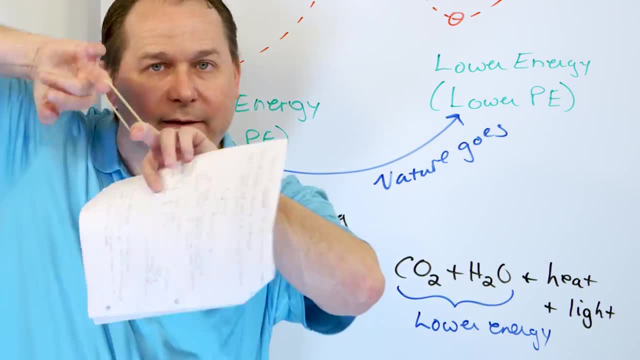 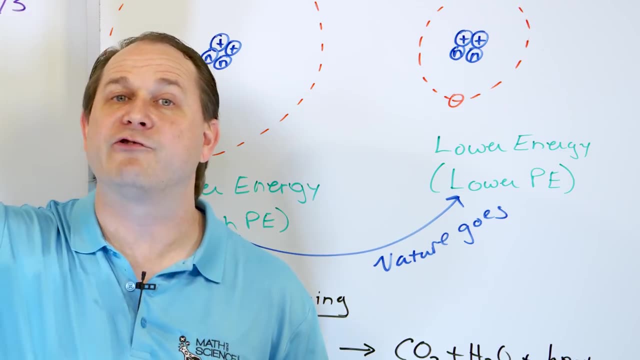 I mean, if you add up all the bonds that are here and the strength of the forces that are there, you end up with a lower potential energy than the situation you had to begin with. Nature is trying to go to a lower energy state. I'm going to stop here. I'm going to stop here. I'm going to stop. 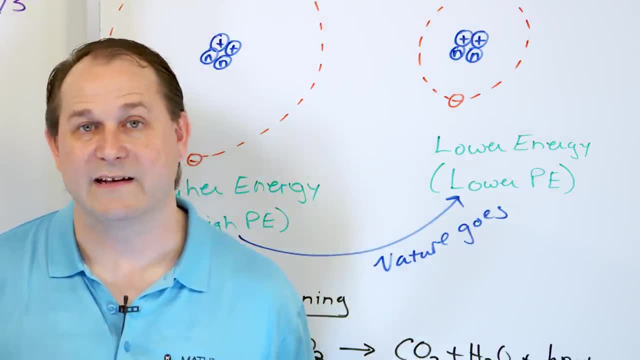 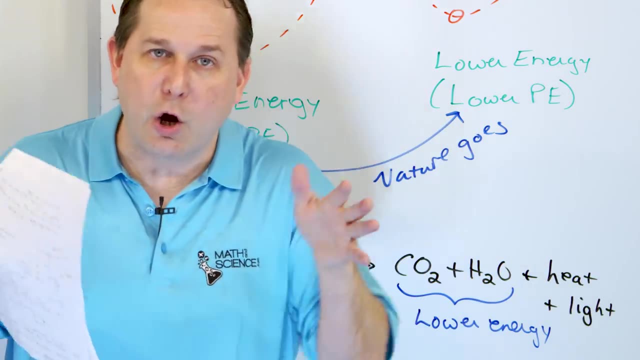 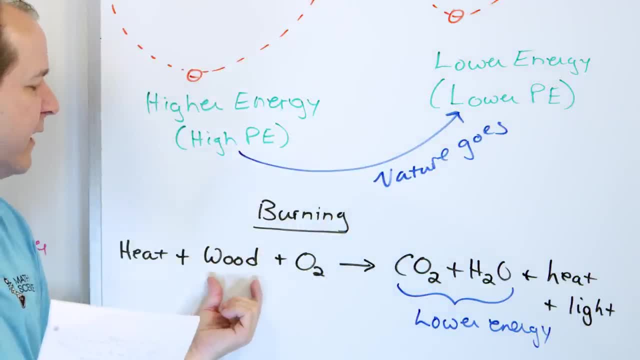 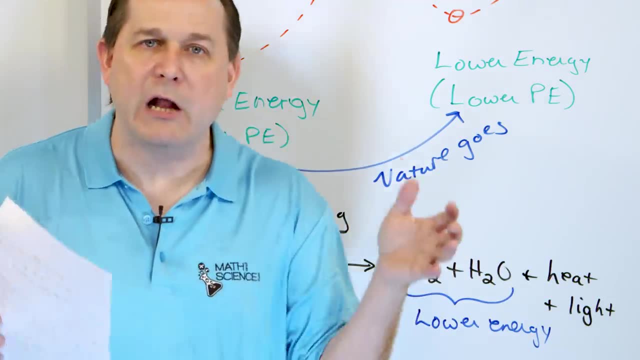 see, And if you were to add up the energies of all of these bonds that are here, which we will do later, and we add up the energies of these bonds here and we tally it all, we're going to figure out that these are more stable molecules because they're in a lower energy state. It's just like 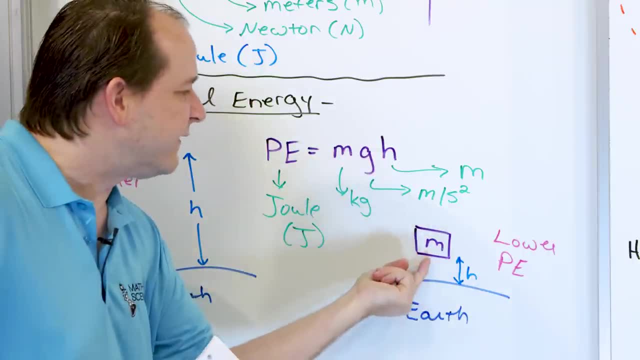 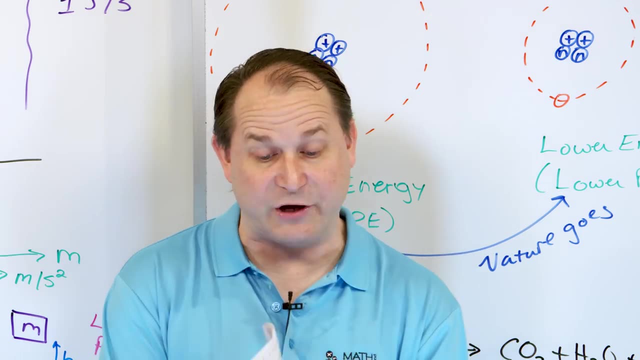 dropping this box and then it gets down lower to the ground. This is lower energy state Lower energy: These molecules are lower energy. All right Now, there's a lot of details that I haven't covered, of course, but that is the gist of it. That's the most important thing. 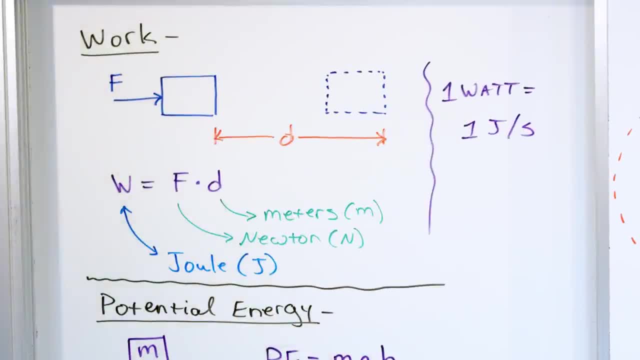 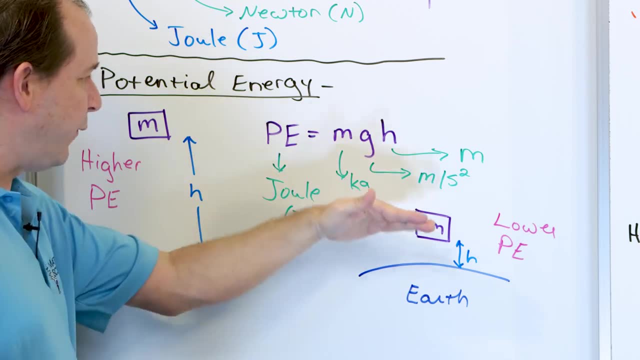 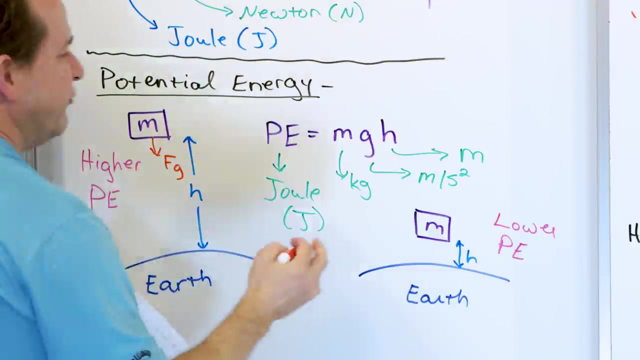 So we have talked about work when things move. We have talked about potential energy when things are higher or lower, down to, basically, to a force that's pulling on it, Because don't forget that acting on this box is some force due to gravity. Call it F, sub, G And then on this, 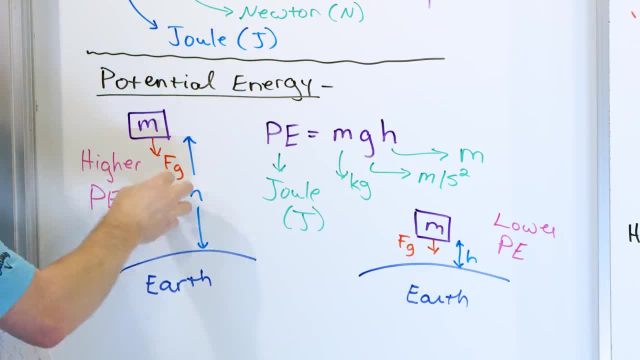 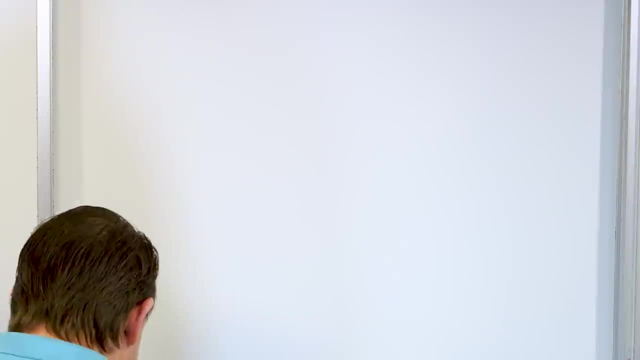 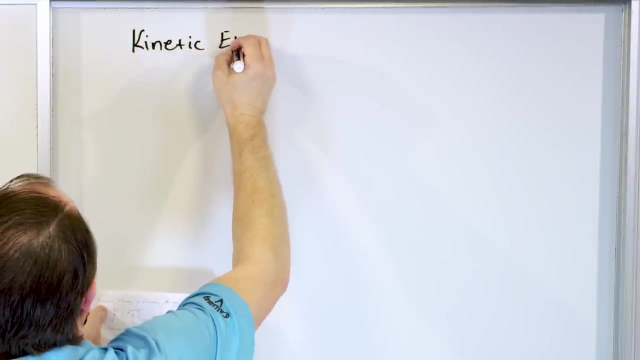 box is also some force due to gravity right, And as it moves down it goes to a lower energy state. So now we need to talk about the third important thing here, that we can then tie everything together and we call it the kinetic energy Right, Kinetic energy. Kinetic energy is the 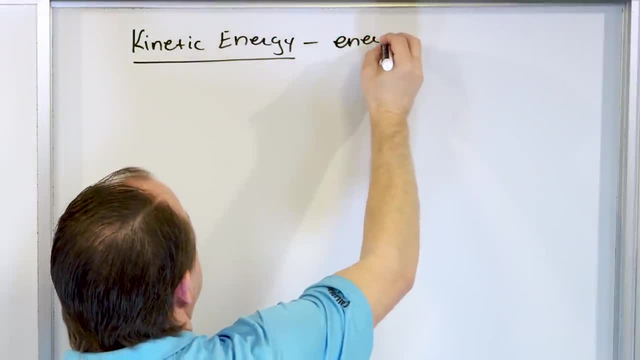 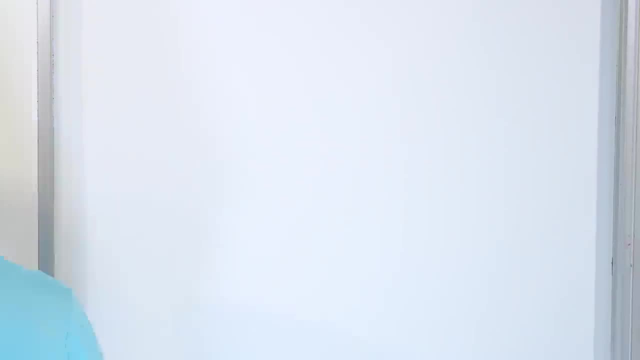 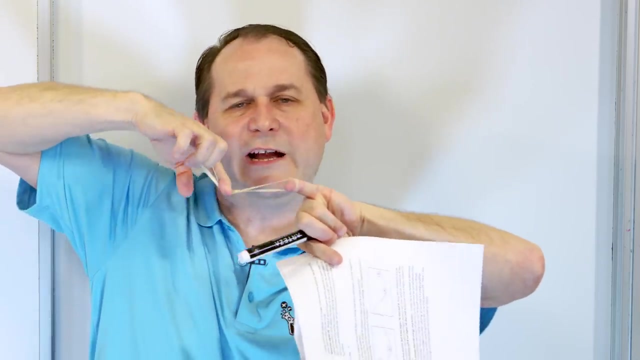 energy of motion. So I'll just say the energy of motion. So, whereas when the rubber band was stretched there was potential to do something right, But if I like take a marble and put it in here and like shoot it across the room, the potential that 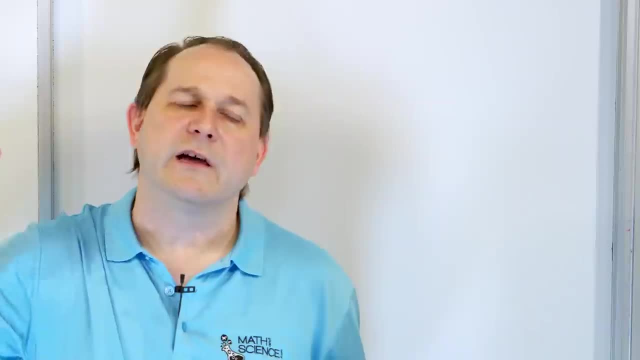 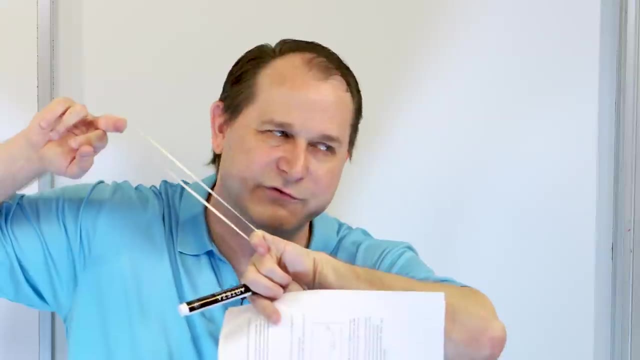 was stored in the rubber band is then converted to motion. Kinetic energy is the energy when things are moving. Potential energy is the potential to do work or to translate to energy when things are not moving. There's nothing moving here, but there's the potential to move Once things start. 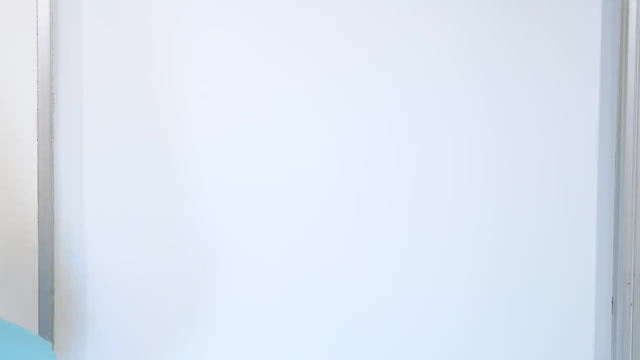 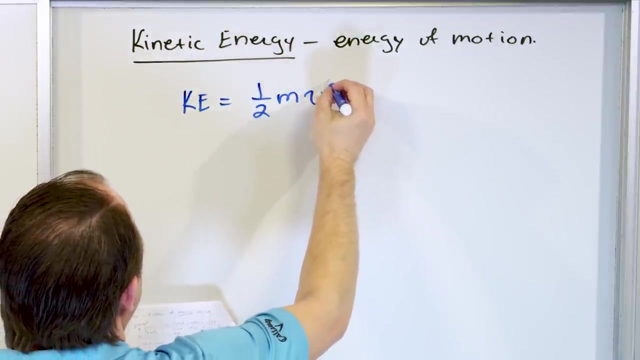 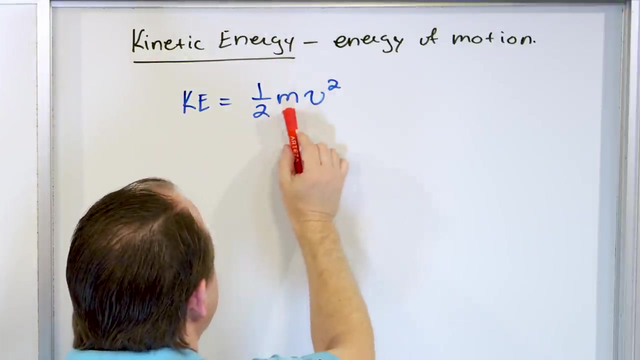 flying. then you have kinetic energy, That's the energy of motion, right. And so the kinetic energy is one half times the mass, times the velocity of the object squared. So the kinetic energy depends on the mass of the object, but it also depends on how fast the object is going. 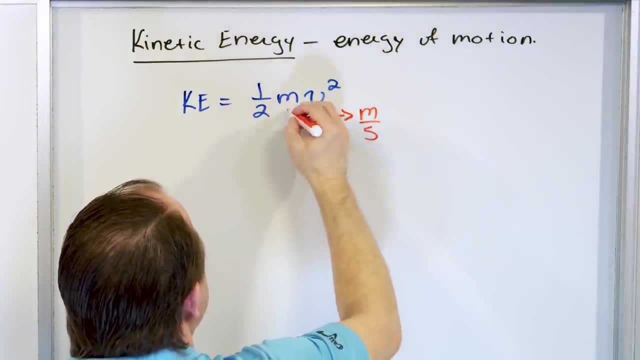 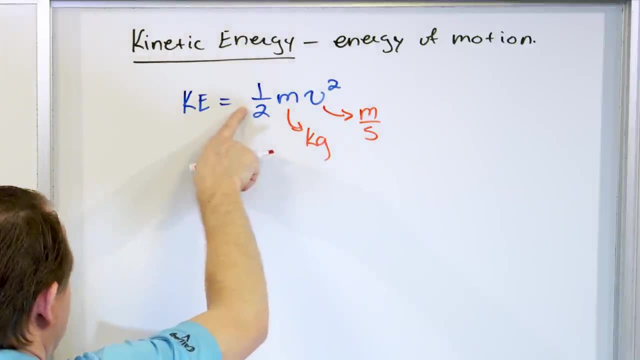 The units here. the velocity is in meters per second, The mass is in kilograms- the same units as before. And when you take a mass times the velocity times velocity, you get a mass times the velocity times one half. then you get a unit here. What do you think? It's joules. 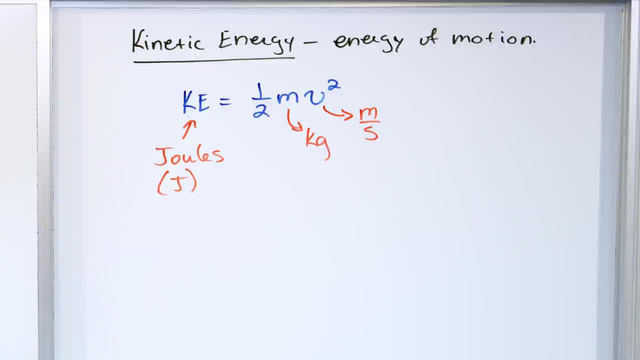 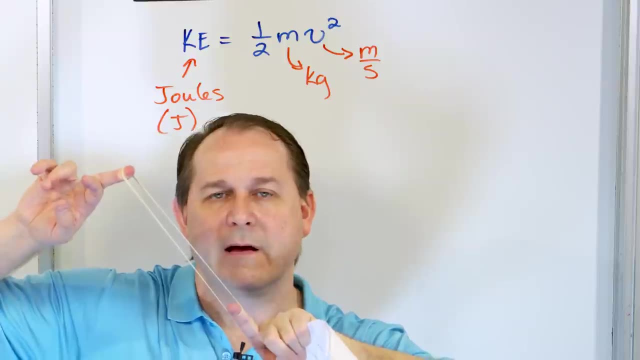 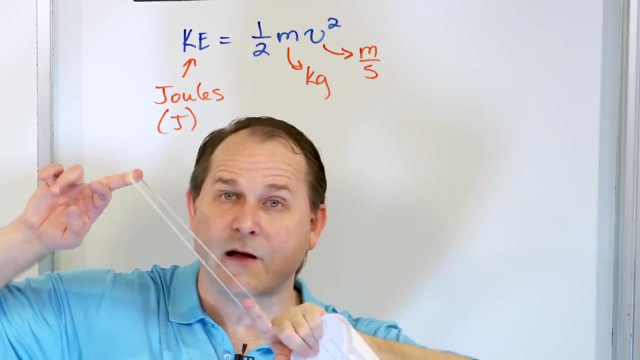 So again, J same exact unit as before. And that is because if I take this rubber band right And I have, let's say, 10 joules of kinetic energy, nothing is moving. but this is the potential. If I could convert all of this potential energy into the energy of motion, and I fling it. 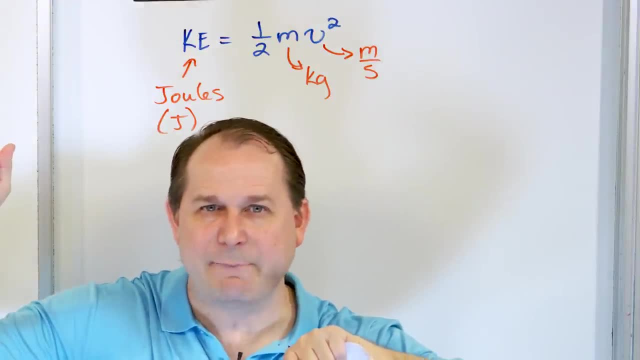 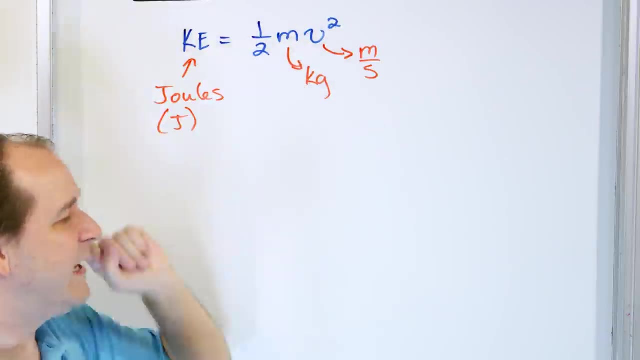 across the room and I could look at its speed immediately when it left my finger and I took the speed and multiplied V times V speed, squared times the mass of that thing times one half, I would get 10 joules of kinetic energy, Because all of the potential energy that was in that. 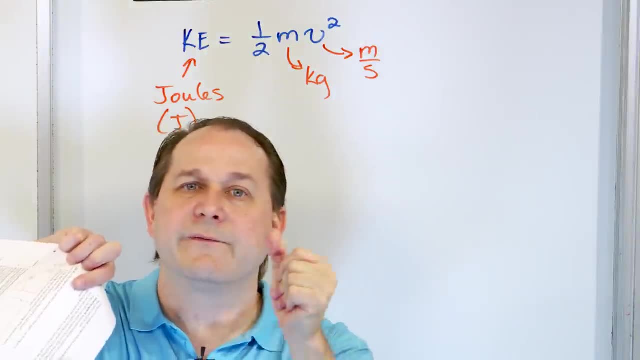 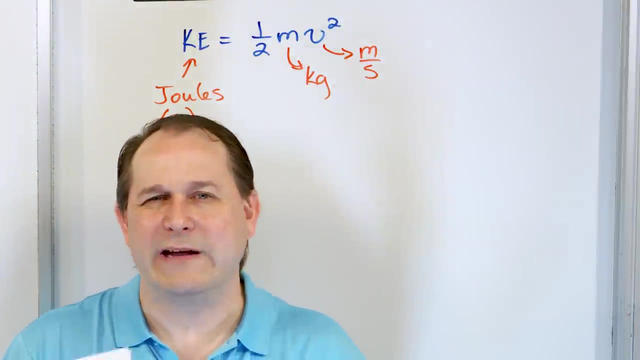 tension and the pulling that was there. it would be converted into the energy of motion. That's what we say. we have a law of conservation of energy. Energy is really not created or destroyed, It's just changed from one form to another. Whenever, I have this box up here. 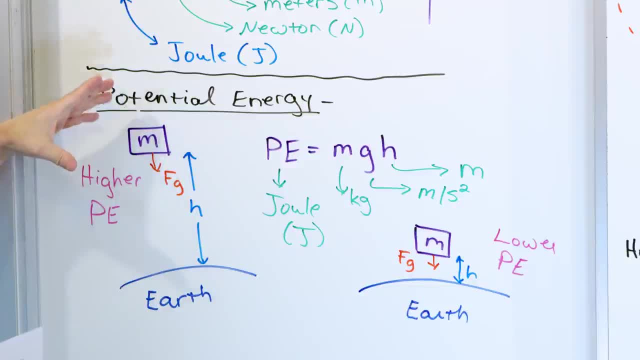 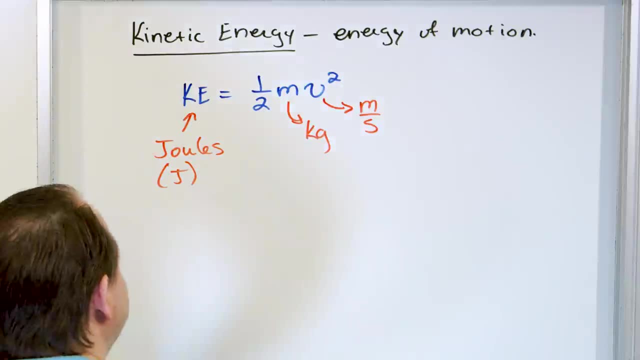 okay, there's a high amount of potential energy, But when I let it go, the potential energy is converted to kinetic energy because it is moving at a high rate of speed when it hits the ground. So the best way to really demonstrate this or talk about it is to talk about a roller coaster. So here's a roller 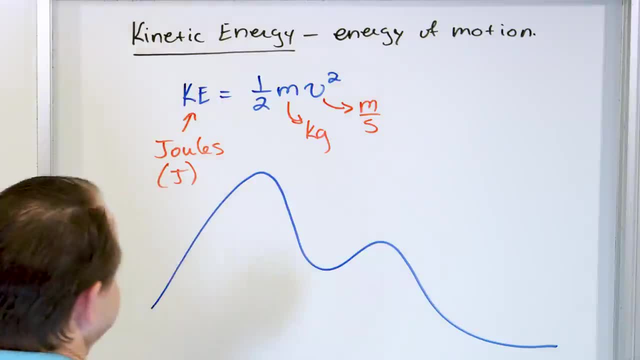 coaster, something like this. So what you do is you start out on the roller coaster and you get to the very high end over here And let's say you're in. let me switch colors. Let's say you're at this position. We're going to talk about what happens when you're at this position on the 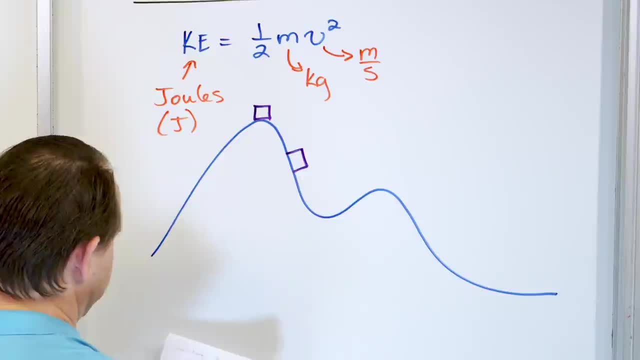 roller coaster, And then we're going to talk about what happens when you're on this position on the roller coaster, And then we're going to talk about what happens when you're on this position, way at the very end of the roller coaster. Of course the roller coaster is moving. 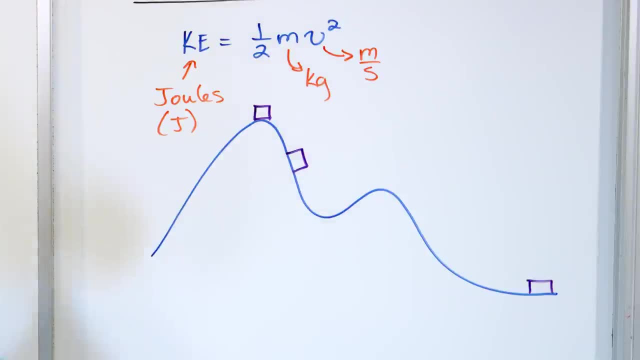 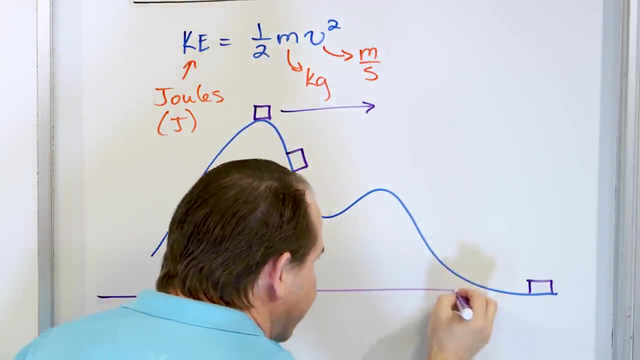 this direction. It's going like this right. So what's going to happen here at this position? What do we have? Well, the ground is right here. So how high are we off the ground? We're the maximum height off the ground. This is going to tell us how high we are off the ground. 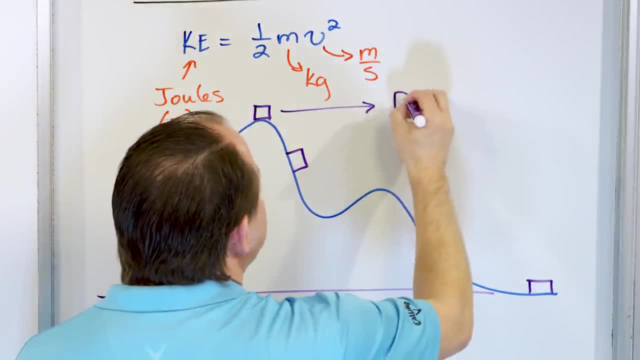 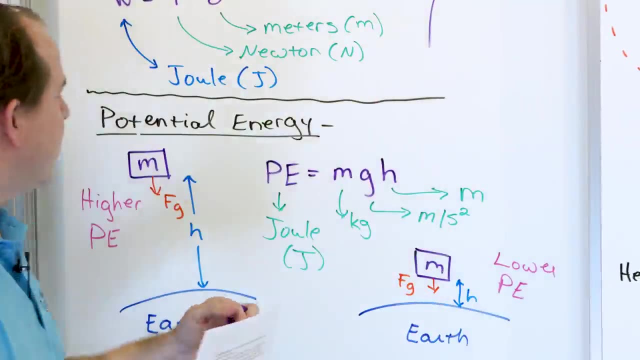 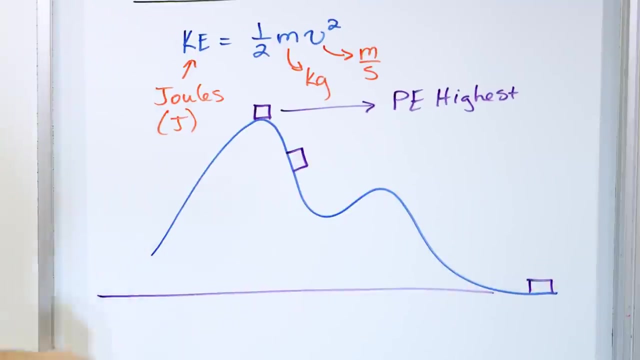 This is going to tell us how high total of an energy state we're in. We have the potential energy is in the highest position Why? Because potential energy is m times g times h, mass times, the gravity times the height off the ground. So in this position we are the highest off the ground. 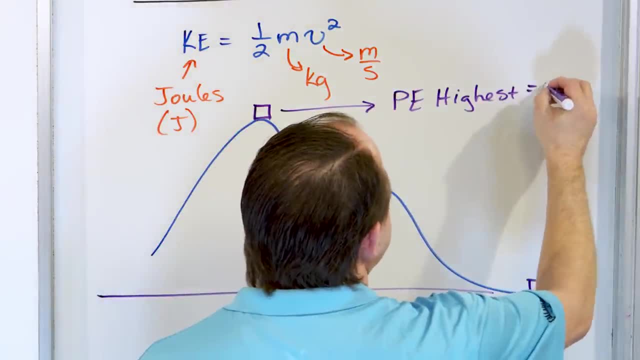 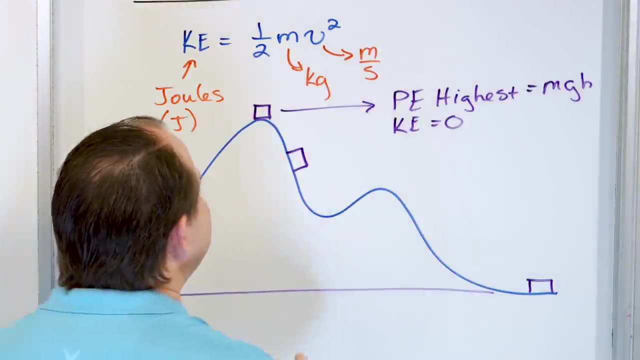 So we have the highest energy mgh. I'll just put m times g, times h- h is the biggest right there, right Now. what is the kinetic energy here? The kinetic energy is zero because I'm not moving. Right at the moment when I stop, right before I go over, I'm not moving. 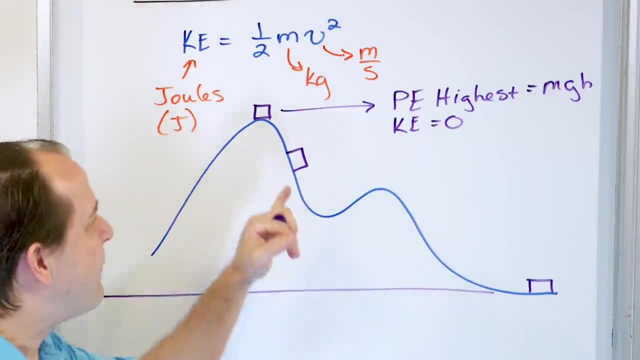 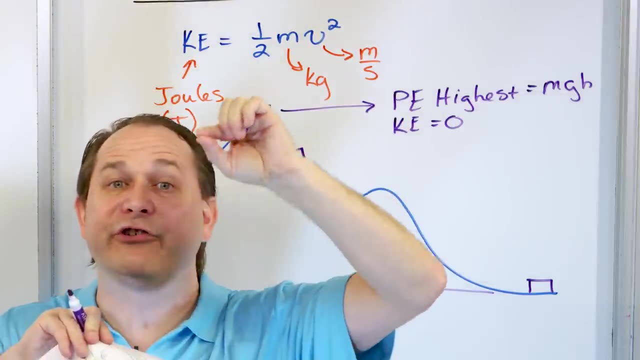 I have no motion, no kinetic energy, But I have a maximum potential energy. You need to start thinking in terms of energy. I have the maximum amount of energy. That is all the energy stored in that system at the top, And it all must come out somehow as this thing goes down the roller. 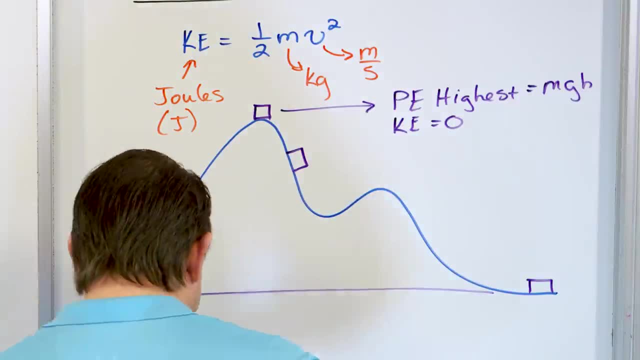 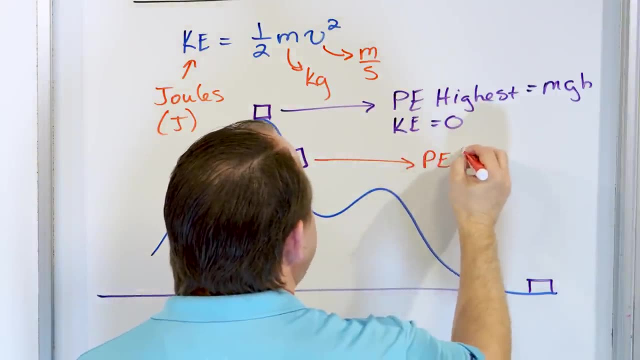 coaster. Now what's going to happen is this thing is going to get to this position right, Which means the potential energy has gone down from here, because I'm closer to the ground, My mgh is because h is now lower. 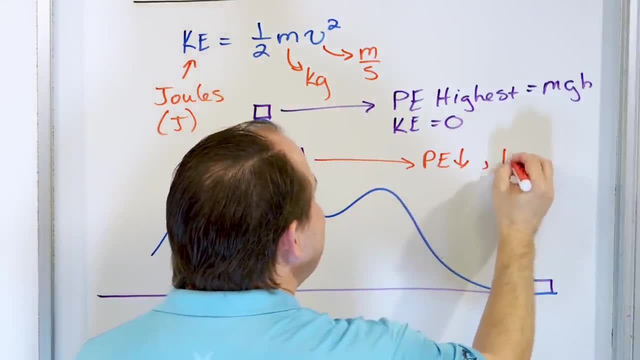 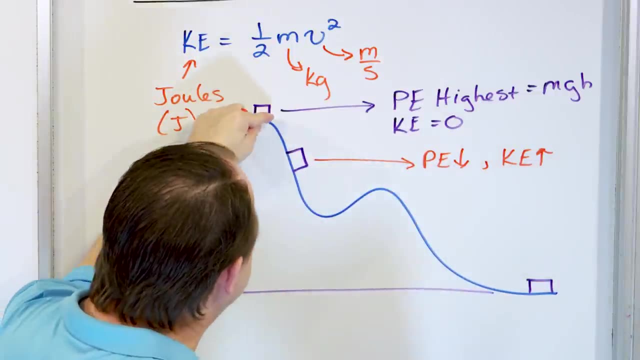 potential energy has gone down But at the same time the kinetic energy that has increased. These are what my arrows mean. Potential energy has gone down because I'm closer to the ground but I've picked up speed. So kinetic energy- one half mv squared is higher. 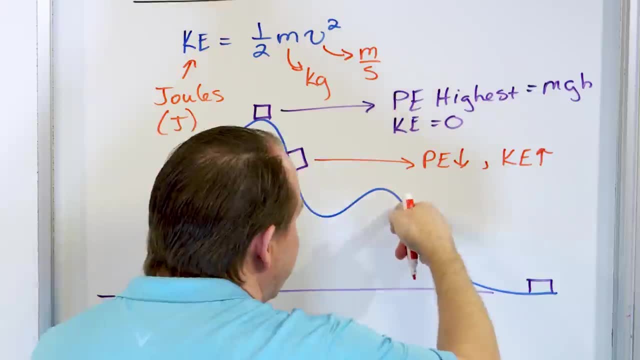 I'm going to do the same thing here. I'm going to get to a local maximum here And eventually, you know, I'm going to slow down, I'm going to pick up speed again. I'm going to get to the bottom. What's going to happen at the bottom? 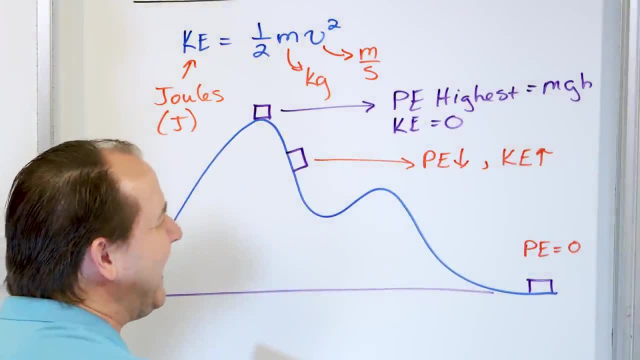 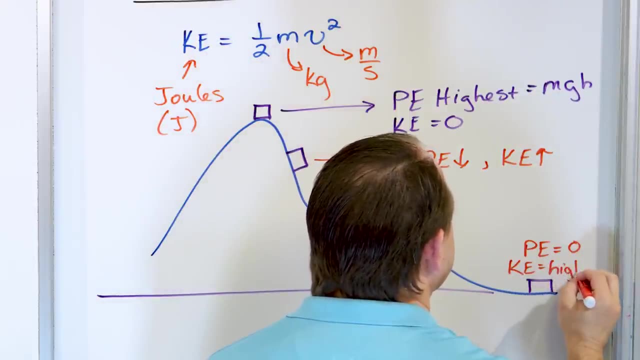 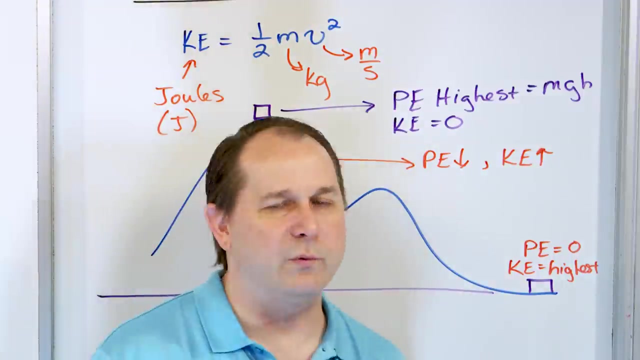 The potential energy is going to be zero because I'm sitting on the ground. There is no h. H is zero, the height, But the ke, the kinetic energy, is highest, Highest. So you see, at the top of the roller coaster the potential energy is the highest, But at the bottom of the roller coaster 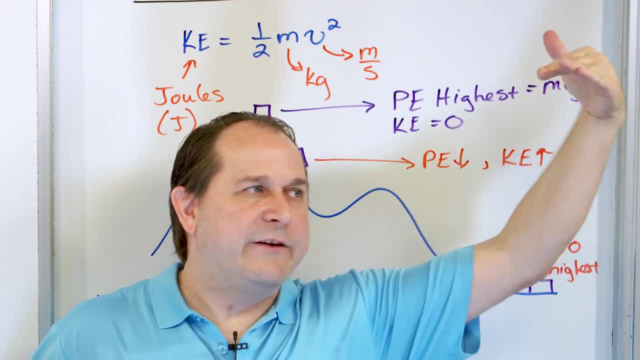 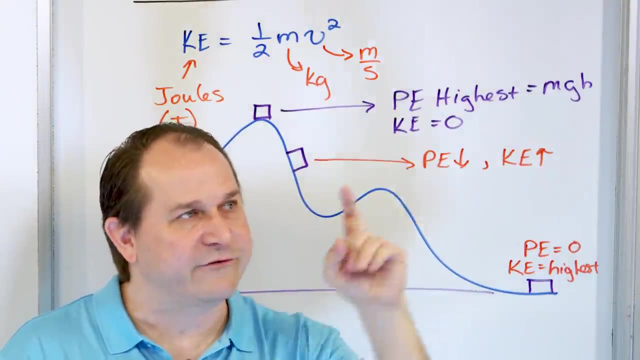 the kinetic energy is the highest, Because at the bottom is when all of that potential energy stored in the system has been bled down to zero. No more potential energy. Things try to go to the lower energy state. So I'm going to get to the bottom of the roller coaster. I'm going to get 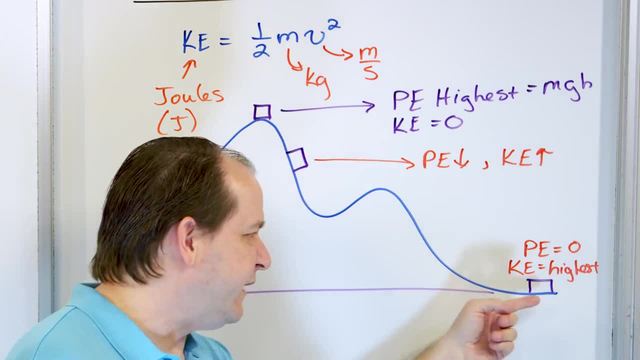 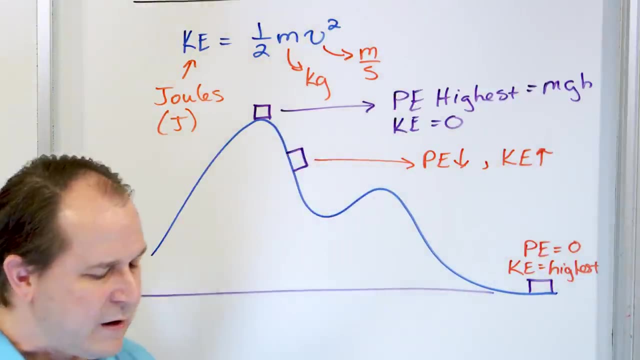 to the lower energy state. But all of it was converted into speed And eventually you slow down with the friction on the tracks and all that stuff. But just forget about friction now. That's going to be the highest speed, highest kinetic energy, So basically energy that was stored by 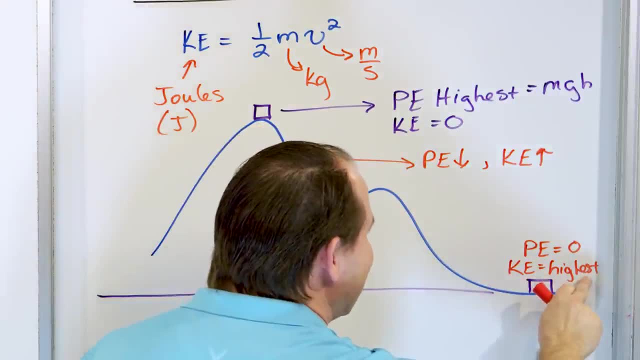 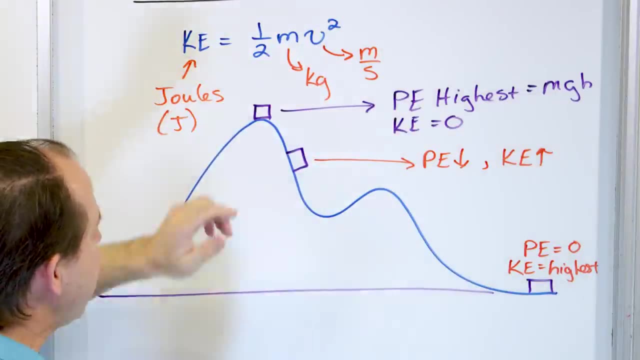 climbing to the top of this thing. it was 100% converted into kinetic energy. No more potential energy, It got put completely to kinetic. If I had 100 joules of potential energy here and there's no other losses due to friction or wind or anything, and it was 100% converted, then it would have 100. 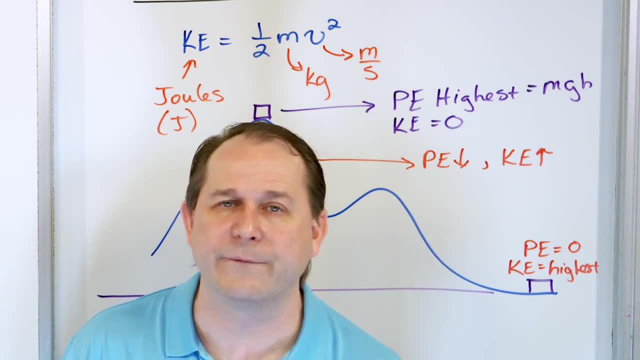 joules of kinetic energy. So I'm going to get to the bottom of the roller coaster And I'm going to get to the bottom of the roller coaster And I'm going to get to the bottom of the roller coaster And at the end it would all be converted from one form to another, from potential to kinetic. 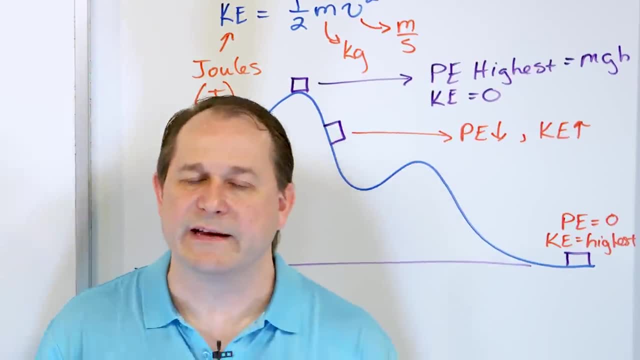 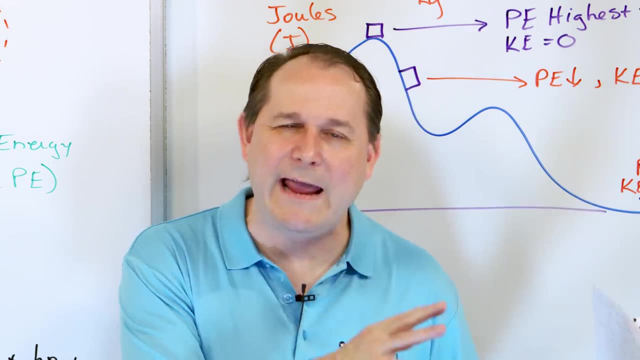 All right, And this is really the punchline of this lesson. Yes, we have a couple of problems I'm going to do at the end, But this is the punchline of the lesson. This part in the next couple minutes hang with me, Because this is literally where it all comes together And I'm 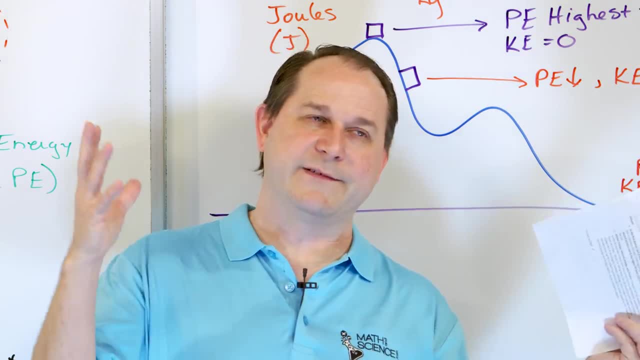 sorry to try to build it up too much, But I'm trying to get your attention, Because sometimes people fall asleep And I want you to pay attention to what we're about to say here. So so far we've done a lot of work And we've done a lot of work, And we've done a lot of work. 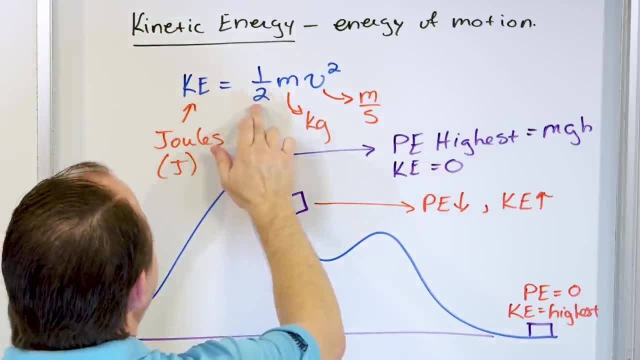 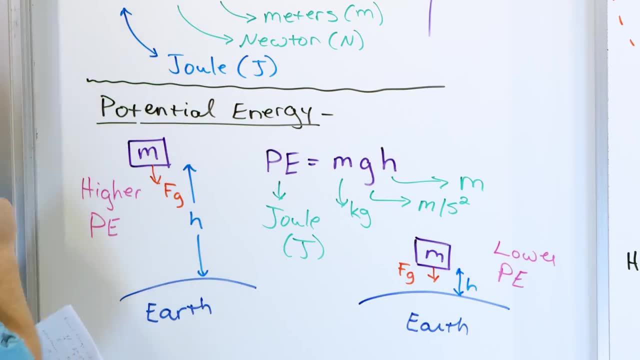 we've been talking about roller coasters. We've been talking about kinetic energy. one half MV squared, that's the energy of motion. We've been talking about potential energy. When things are high off the ground, they have high potential energy. 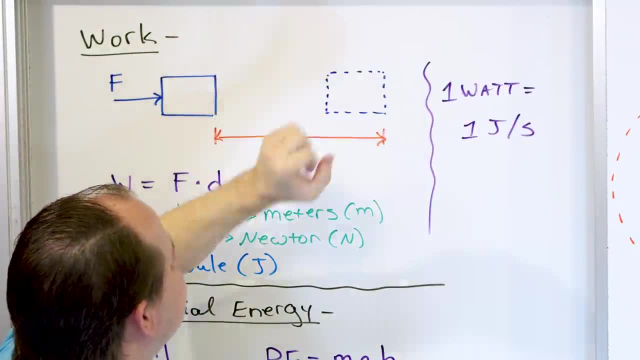 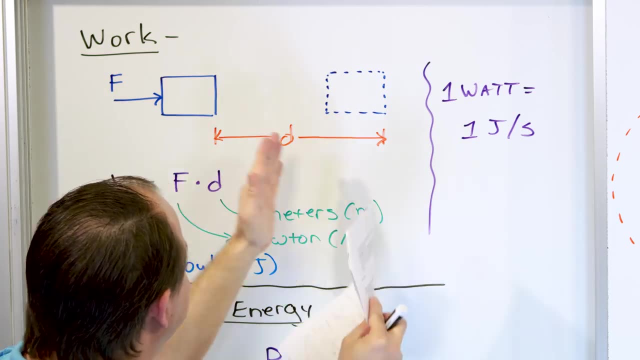 And then we talked about the energy. when something is moved and it gets to a new stopping place, then there is work done on it and you can convert potential energy into work done, Even after the object has stopped. you've done work on the object, there's no motion anymore. 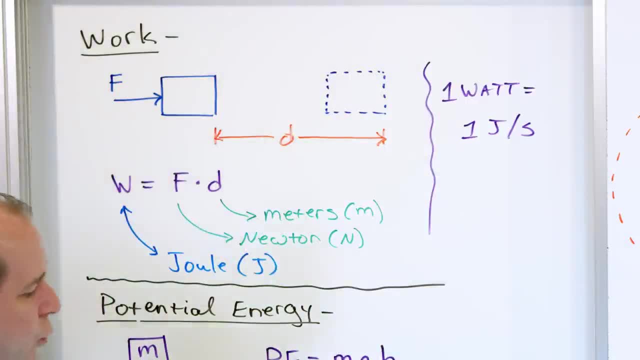 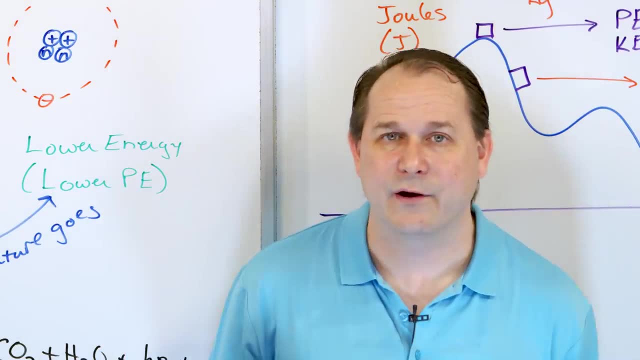 but that potential energy can be converted into a kind of a new kind of energy called work. Now, all of the stuff we've been talking about has always been about gravity, And so now I need to tie it together right, This is not a physics class. 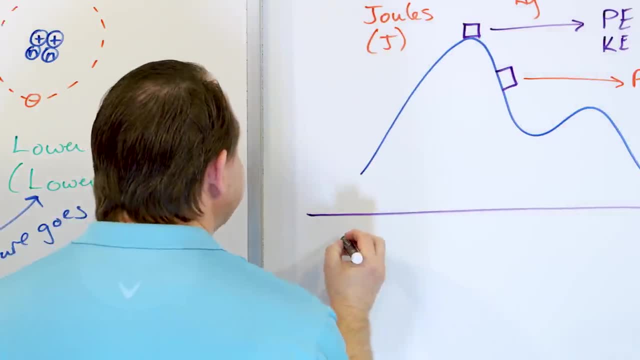 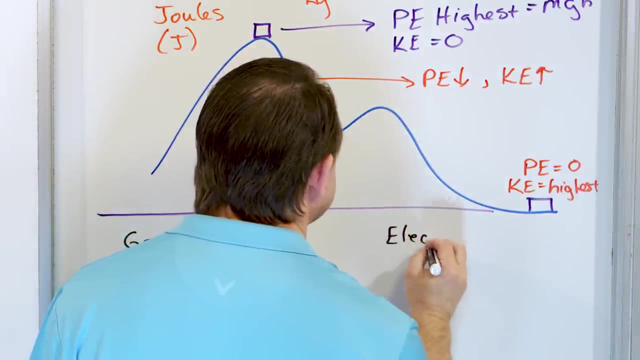 but we can learn a lot by looking at these things. right, Let's take a look at gravity And we're gonna compare this to the electric force. Now I've told you that the electric force is millions and millions and millions of times. 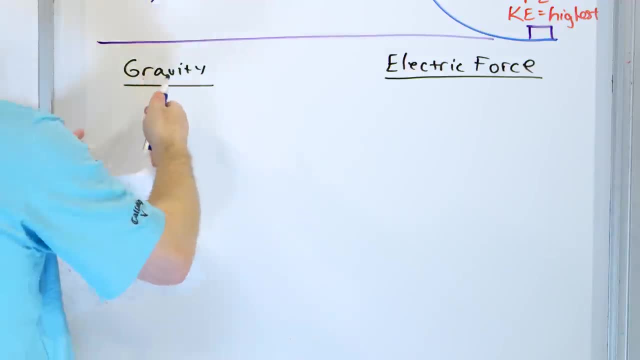 stronger than gravity. that is true. However, the equations for gravity and the equation for the electric force, they look really, really similar. Let me show you what this is: The force of gravity between any two objects, like two apples, or two planets, or two, anything right. 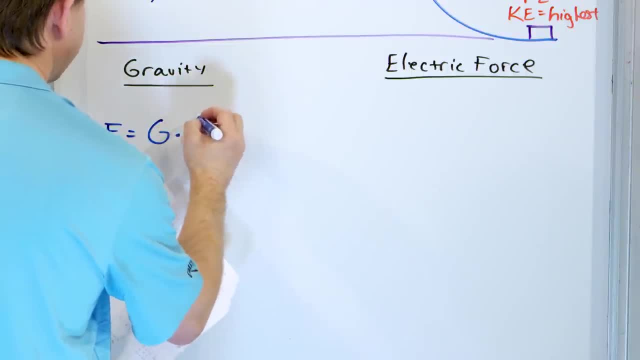 is just what we call the gravitational constant G, multiplied by mass number one of object, one times mass of object number two, and then it's gonna be divided by R, squared the distance between the objects, right? So if I have basically two objects here, and this is M1,. 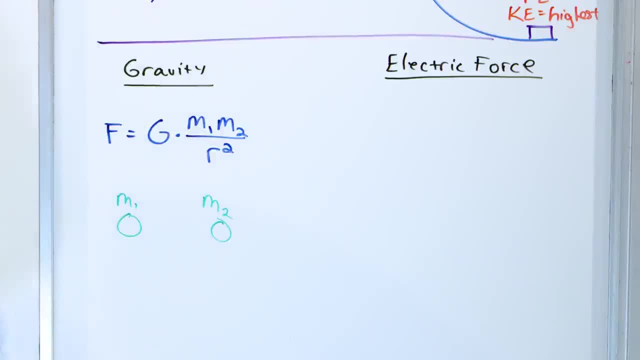 and right here this is M, mass number two. it depends on the masses of the objects, and gravity is always attractive, right? So there's gonna be some attractive force right here and it's gonna be F, essentially a mutually attractive force called F. 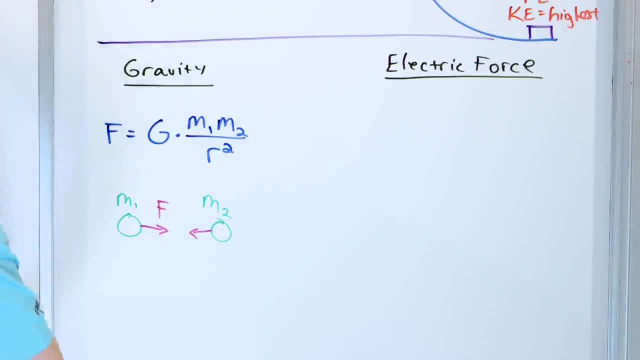 between them and it depends on the distance between them, which is, I have to label here as well, and the distance between them here is R. So you can see that as R gets bigger and bigger and bigger, the objects get farther apart. 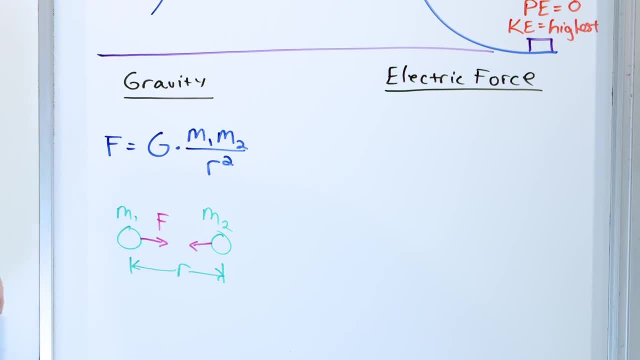 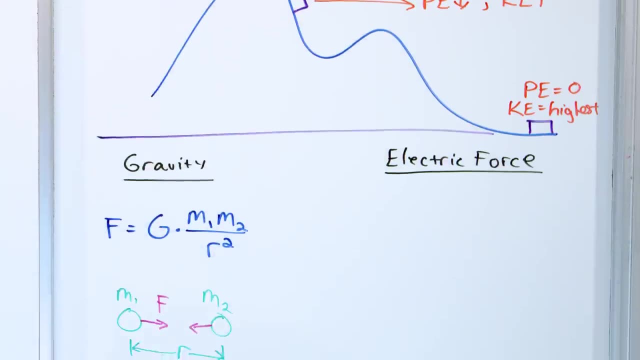 If this denominator gets bigger, the force gets smaller, and so that means an object across the universe from you does not pull on you very much, compared to two objects next to each other. All right, but notice, it's G, some constant. this is just a number. 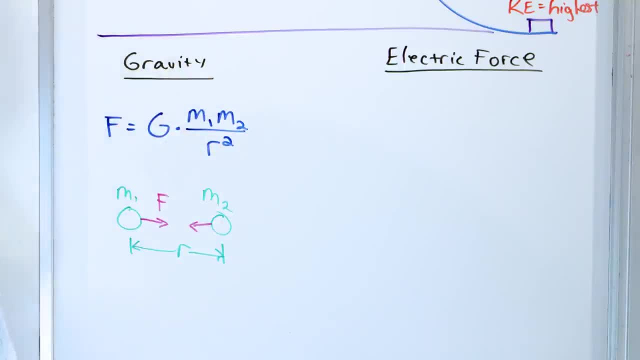 times the two masses in kilograms divided by the distance between them in meters, and you gotta square it. everything's squared there. Then you get a force which is in. can you take a guess The force is gonna be in newtons. 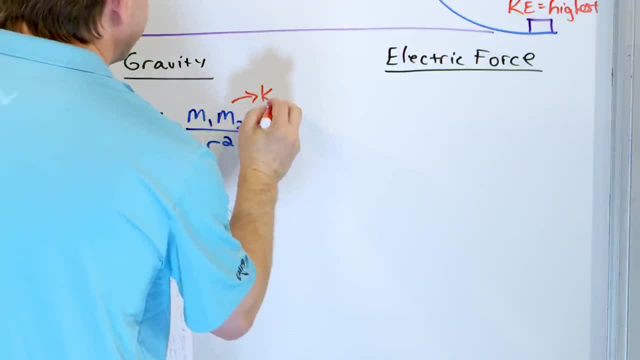 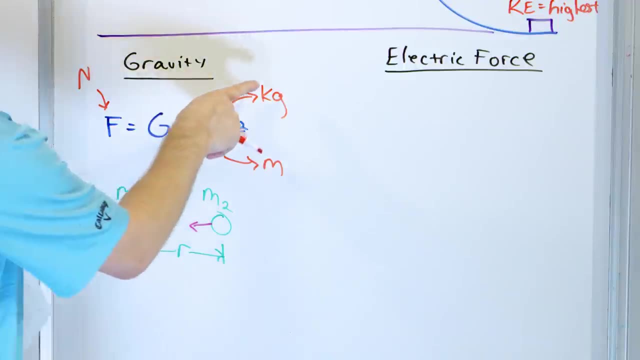 So this is newtons, right? And then these are in kilograms And these are in meters and the units of G are chosen. You can look in a physics book and look at the units of G, but basically you put in kilograms, meters. 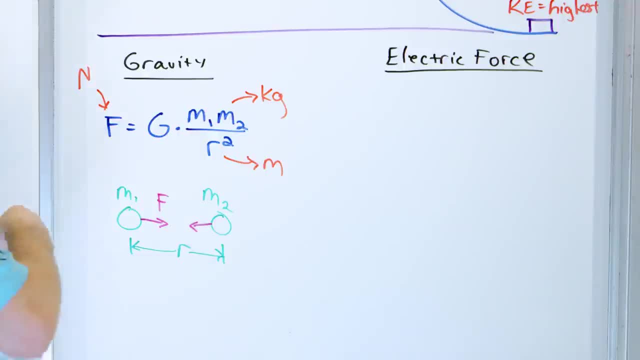 and then you multiply by G and out spits a force in newtons. Now why are we saying all this stuff? Because check out what the force, the electric force, We'll put F sub, we'll call it F sub, G for gravity. 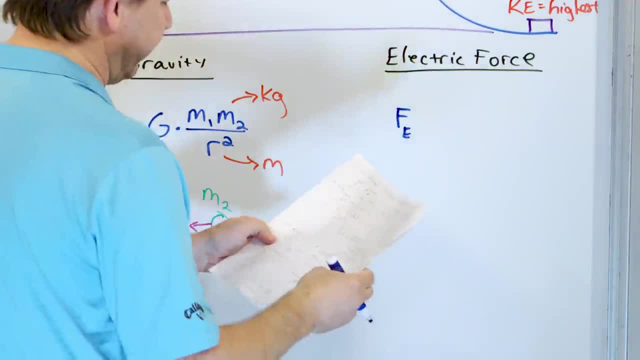 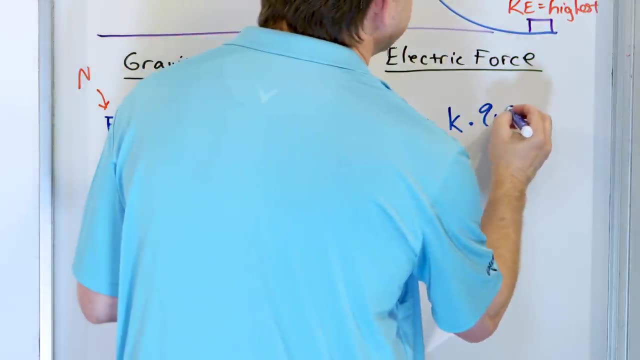 Let's take a look what F sub E is for the electric force. It is some constant called K, multiplied by the charge on object number one, multiplied by a imiz by the charge of object number two, and you divide this by r squared. Take a look at these two. 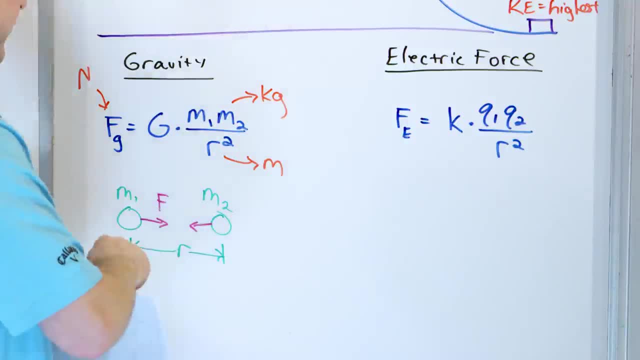 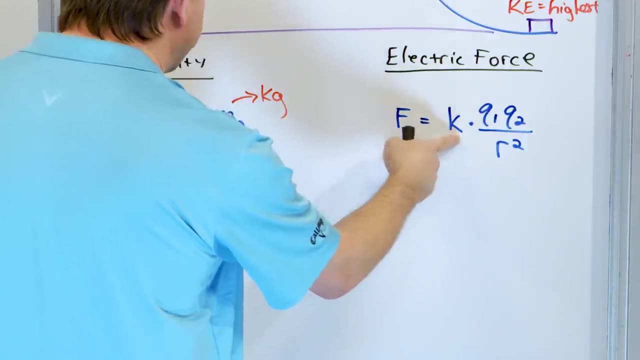 equations. Don't they look the same? And yes, they are the same. Basically they're the same form. G is called a gravitational constant. It's just a number. K is called an electric constant. It's just a number. R is the distance between the objects in meters. R is the distance between: 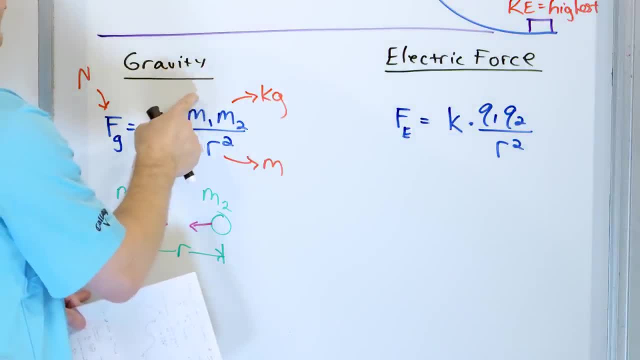 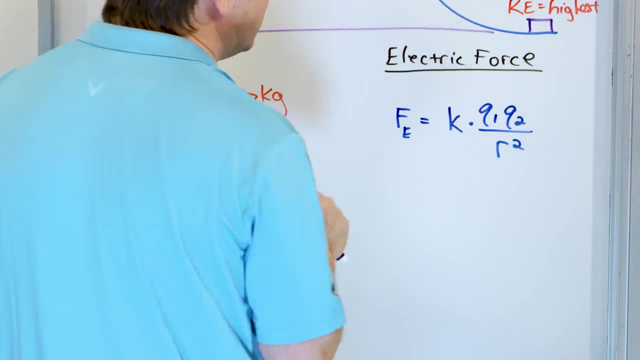 the object meters Here because it's gravity and it's always attractive. it's related to the mass of the objects, how much of the object we have Here. it has nothing to do with the mass, It's just how much charge An electron has a negative one charge. A proton has a positive one charge. 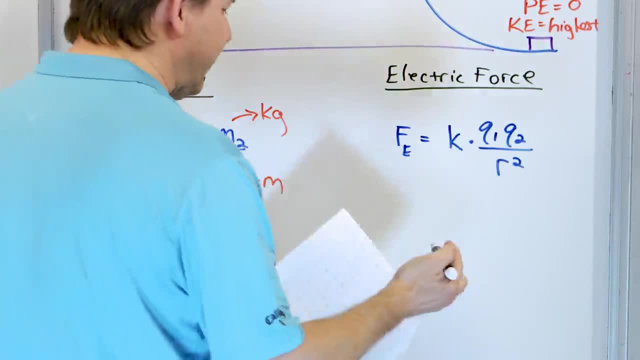 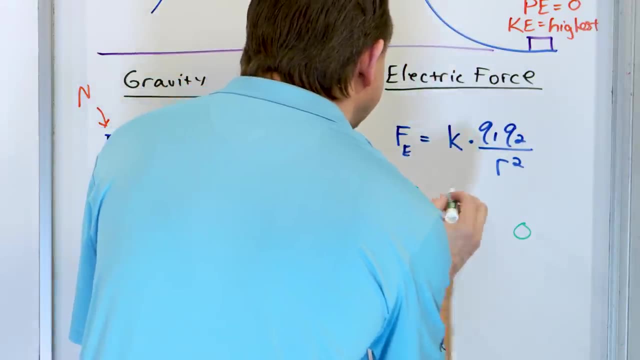 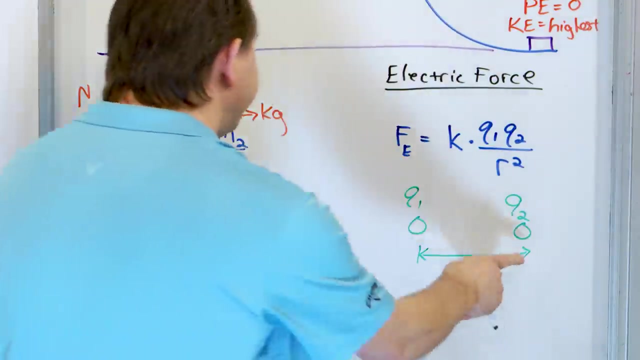 right, But the actual form of the equations are exactly the same. So let's kind of draw particle number one, particle number two like this: This will have some charge on it, like an electron or proton or something like this, and the distance between these guys is r. So the diagram is the. 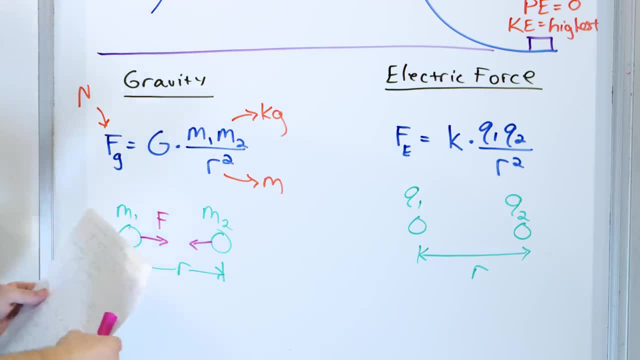 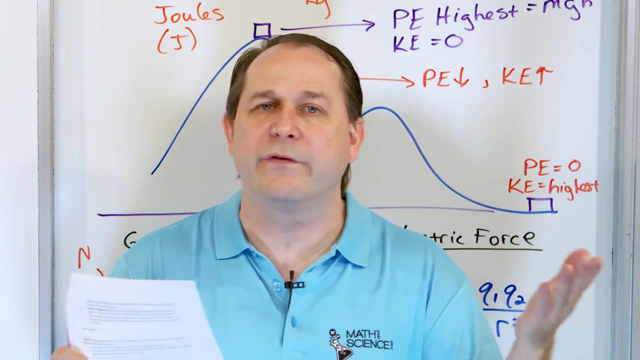 same. Now, the main difference is that gravity is always attractive, but electric charge can be attractive or repulsive. That is a main, main, main, major difference. But besides that, these forces look the same. I mean, obviously electric force is stronger, but the equation 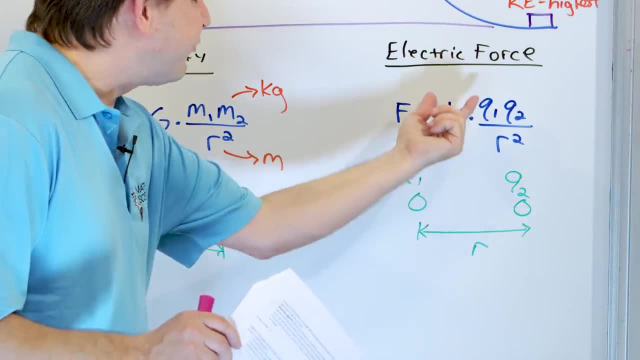 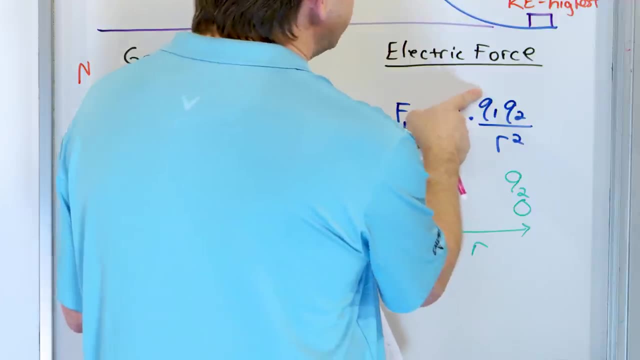 looks the same right. So how can you get attractive and repulsive forces right? So the charge here is going to determine that If you put two positive charges here, then you're going to get a positive answer and they're going to be pushed away If you put two negative charges here. 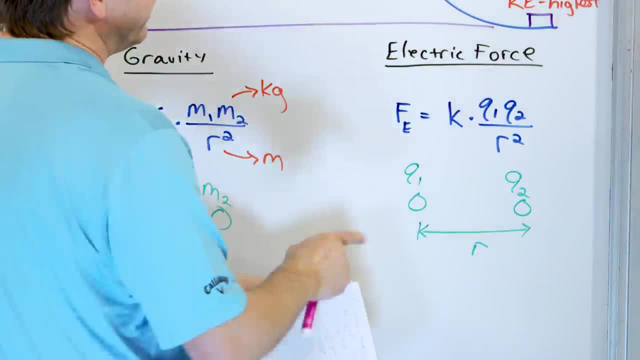 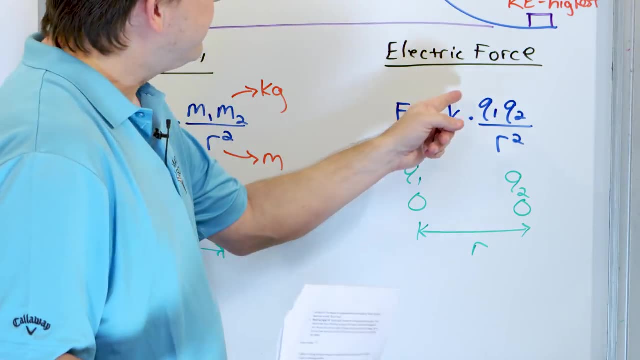 negative times. negative is positive, you're still going to get a repulsive force. If you put one positive and one charge is negative, you're going to get a negative answer and that means it's attractive. So the charges, you know, opposites attract and like charges repel. you just dump the. 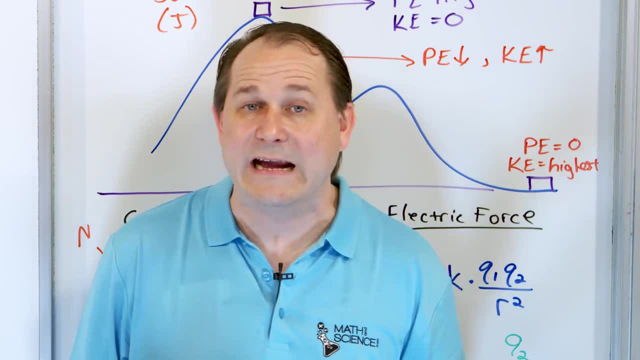 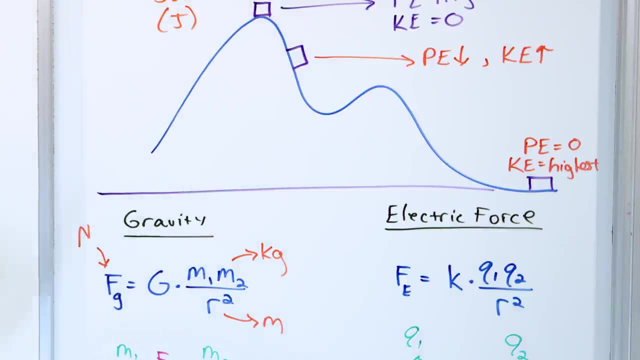 charges in there with their signs and then the sign of the answer in Newton's tells you if it's attractive or repulsive. So why am I saying all this stuff? Because I told you that chemistry is governed by the electric force. It's governed by the forces. between all these charges on a 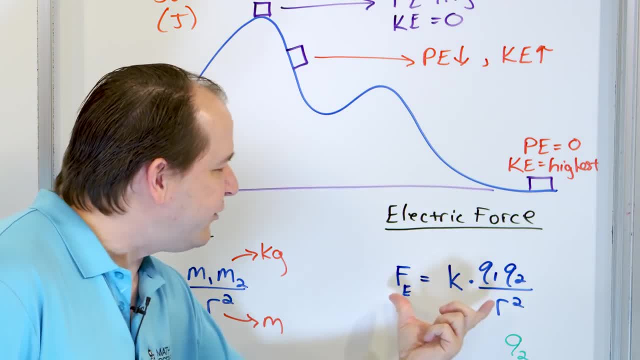 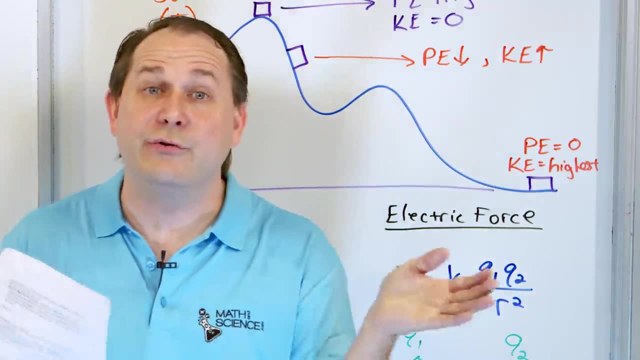 microscopic level. But then now I'm telling you that the electric force is governed by the equations that govern the electric force. We don't have to be an expert in physics to see that this is the same as gravity. So then, it allows you to use your knowledge of gravity to kind of predict. 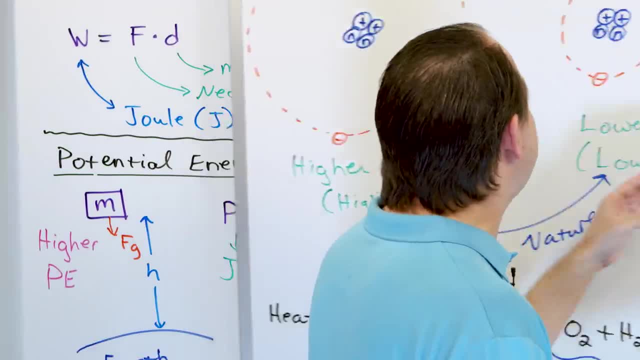 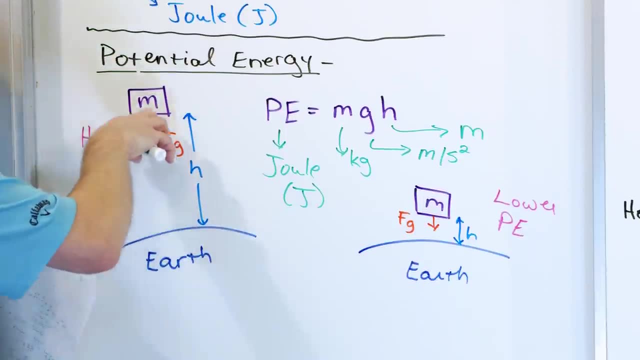 sort of what's going to happen, And that's why I spent the beginning of the class talking about all of these things that don't seem to have anything to do with chemistry. Potential energy is how far away something is from the ground. It's m, times g, times h when it's talking about. 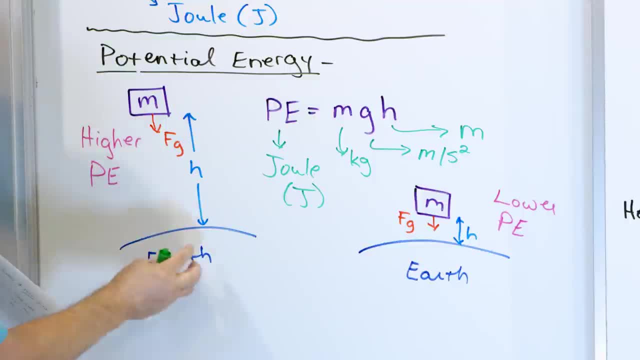 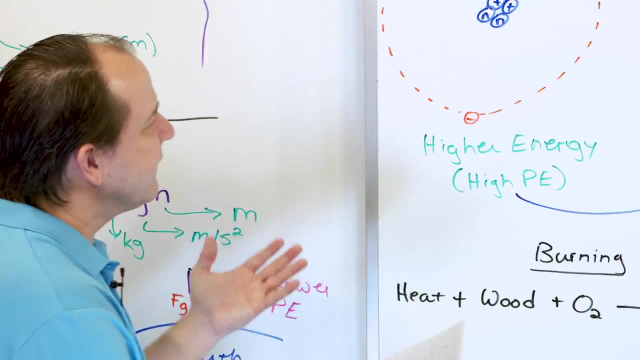 gravitational potential energy. The farther away you are from the planet, the more potential energy you have. The closer you are to the planet, the lower potential energy you have. Because of the similarities between gravity and electricity, the farther away an electron is in a higher energy. 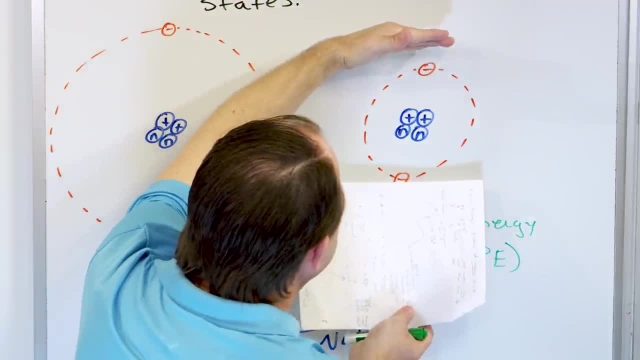 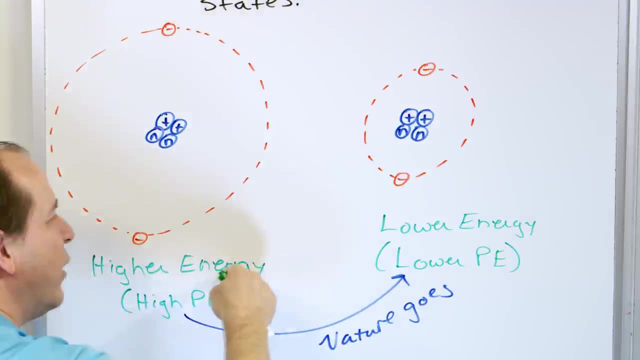 level, that means it's a higher potential energy. The closer it is to the nucleus is the lower potential energy. Just like things like to fall from high to low energy, electrons like to go from high energy state to low energy state. This manifests itself when we actually burn things. 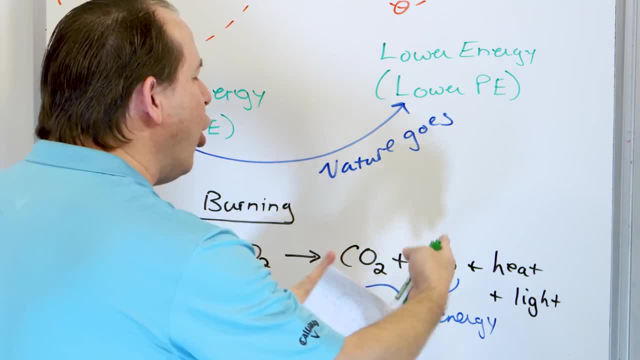 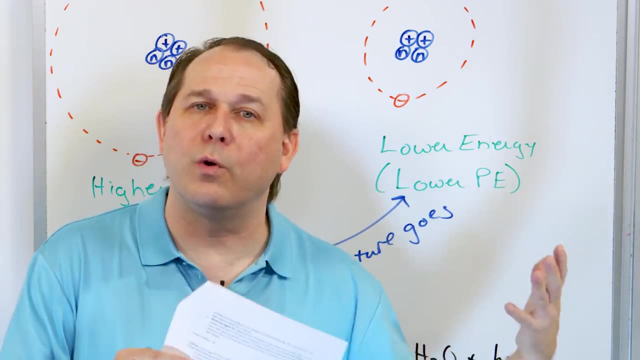 because we break the bonds and then they're allowed to rearrange, But they always go into a lower energy. I shouldn't say always, because you always find some exception, But they almost always go into some lower energy configuration. And when I tell you: 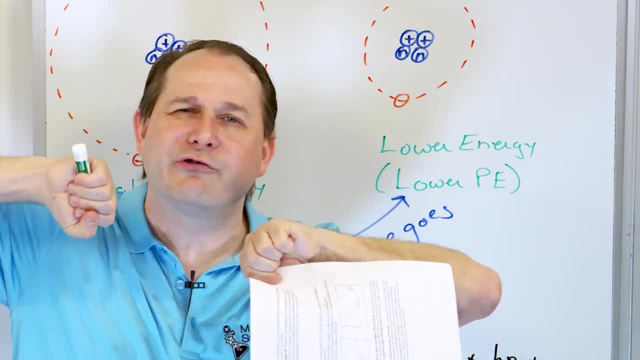 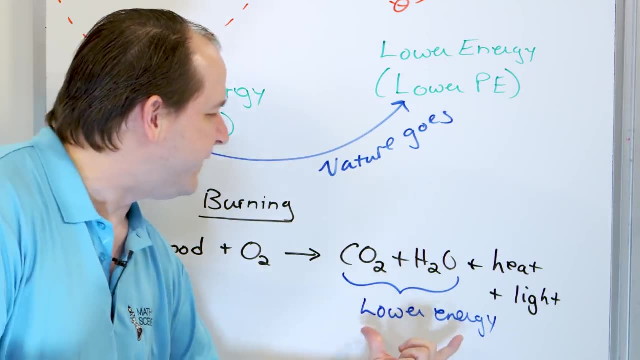 lower energy configuration. I'm talking about the rubber bands. How strong are the forces? How close are they? How much force is there? That is the potential energy. And the potential energy of these bonds is going to be less than what the sum of what we started with, because the reaction 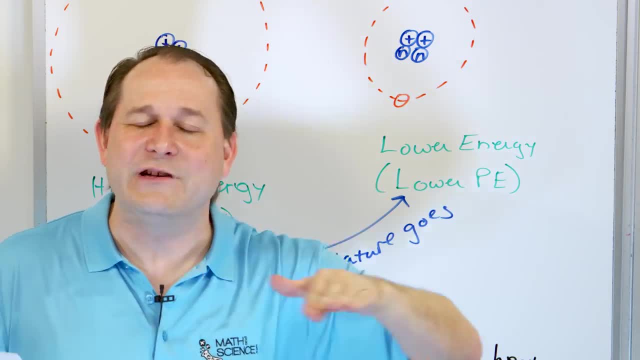 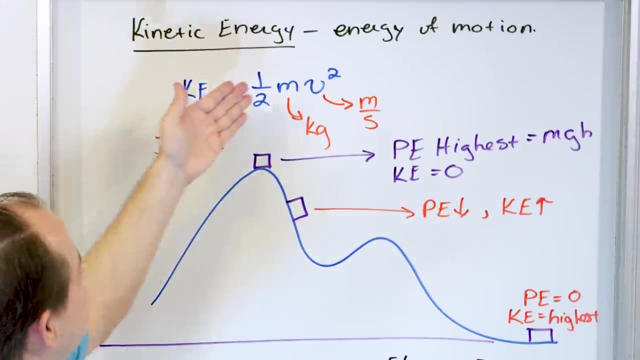 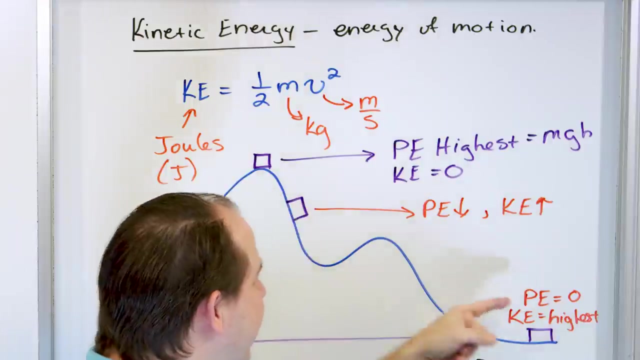 proceeds like this. This is a lot of what governs if a reaction happens or it doesn't happen. Then we talked about the idea of kinetic energy. This is the energy of motion. High potential energy. low potential energy at zero: Zero kinetic energy. highest kinetic energy: This means the 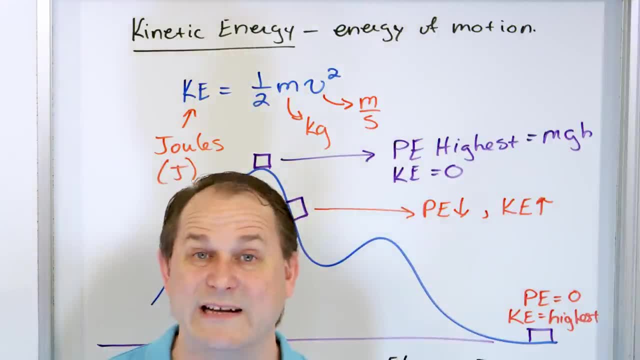 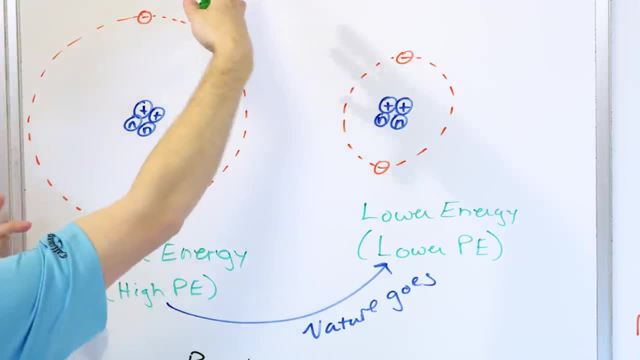 potential energy is converted into motion energy, called kinetic energy. at the end of the roller coaster run, If you had some reaction, where electrons were in a high energy state and they were allowed to combine down and get into a lower energy state, what do you think is going to happen? 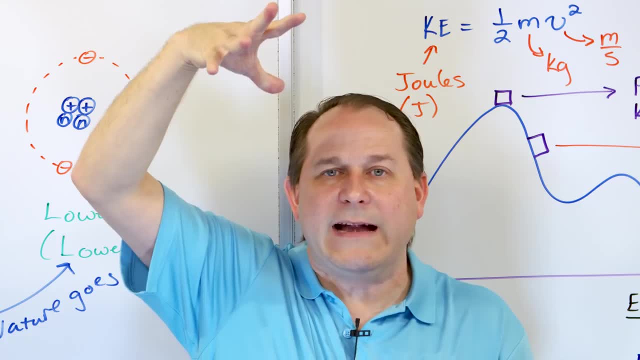 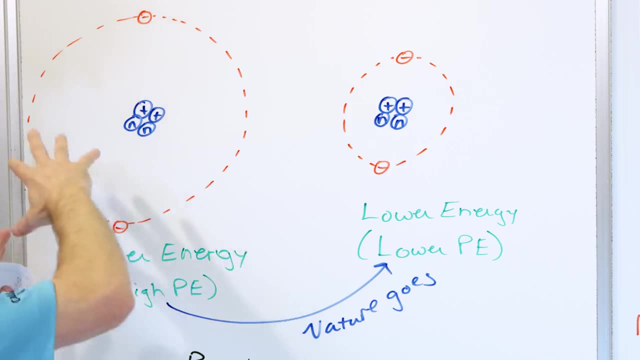 They kind of crash in, right. Think about if you drop a bowling ball and it accelerates down and smashes into the ground. It kind of like creates heat and vibrations when it hits the ground, right? Well, if you allow these things to rearrange and the electrons crash into a lower 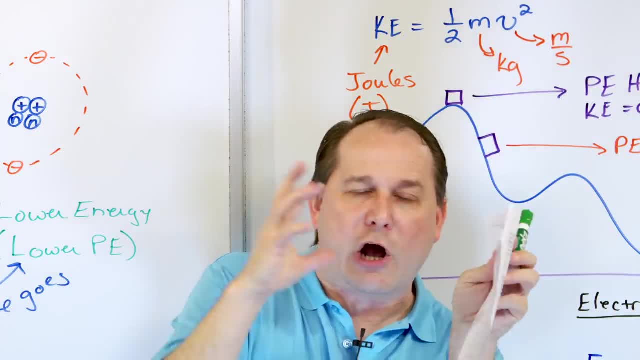 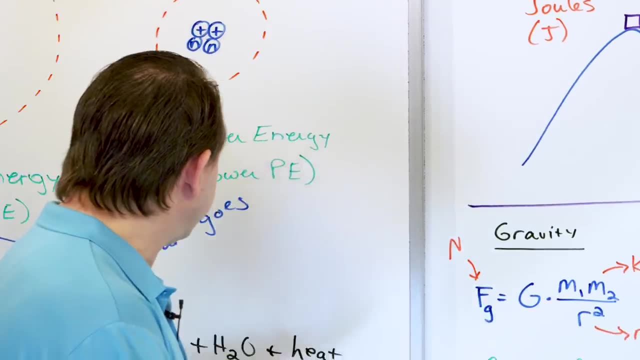 energy configuration. you can kind of think of them as crashing in and causing vibrations And that manifests itself as heat, Not always in every chemical reaction, but you can think of the burning that's going on as breaking bonds, forming bonds in a lower energy, And some of the energy 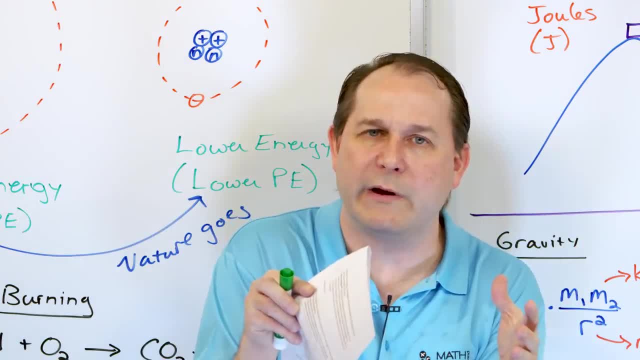 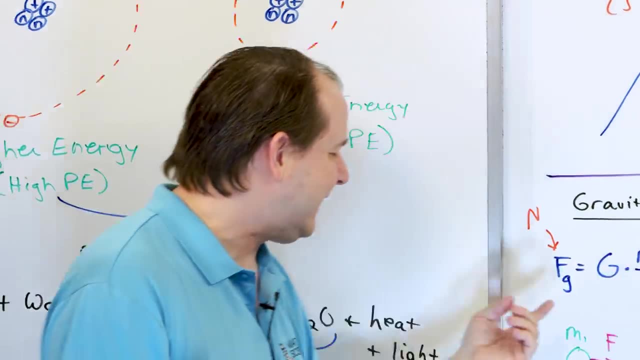 must come out of heat, And that's what we're talking about. So if you have a lower energy state heat- because when the electrons crash down into a lower energy state, everything's vibrating- once it crashes down like this, and then you have some heat that is released And that heat then goes. 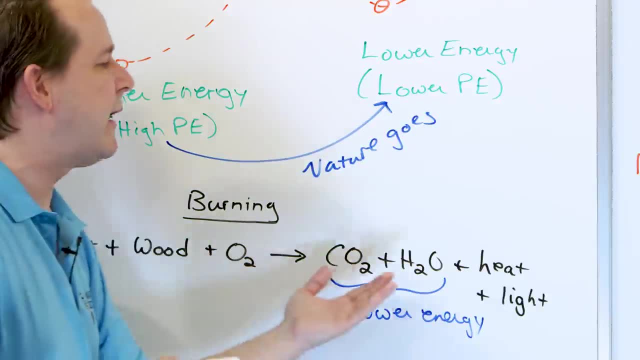 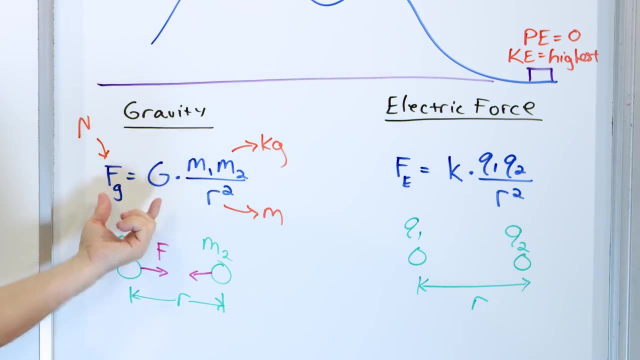 back to breaking up more bonds of wood and oxygen and continuing the process until your campfire is burned out. And all of this is true because the electric force and the gravitational force have similar forms, So the intuition that we can get from physics applies to chemistry. 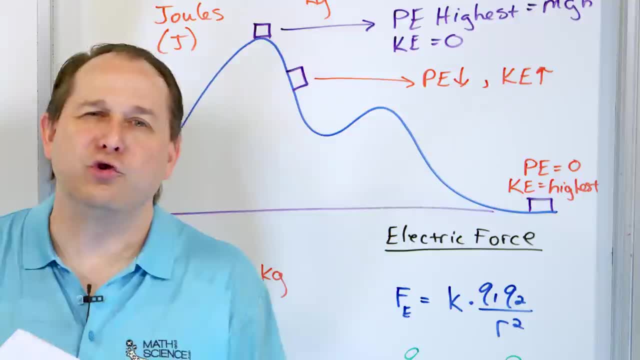 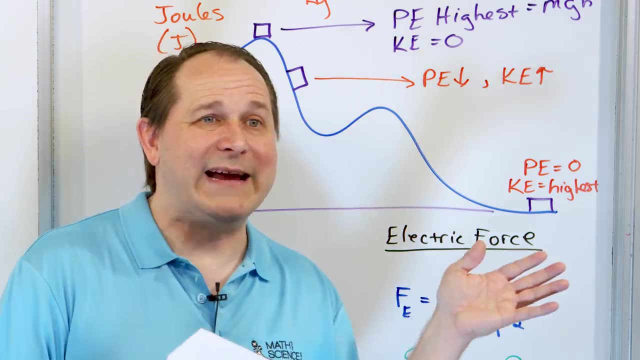 This is what I'm trying to tell you is the punchline. This is something that you normally don't. really you almost never see it in a chemistry class really laid out like this, But if you do get it, it's like two months or three months in. 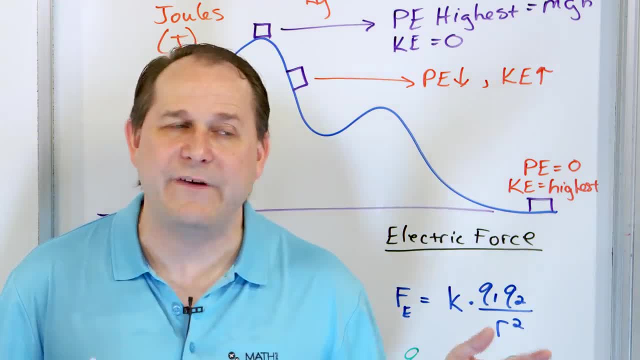 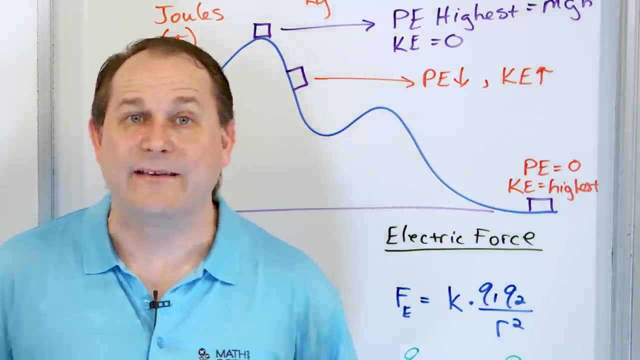 the future, And you really need to have this in the beginning. I think it's very helpful to know, to break down the mystery: Why is this thing reacting? Why is it doing anything? Why doesn't it just sit there? And that's the reason why: Because the nature likes to go from high energy. 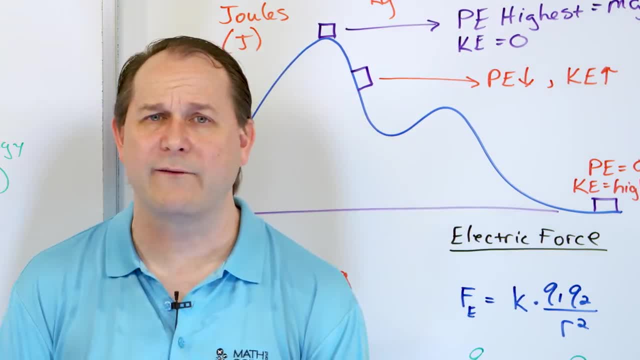 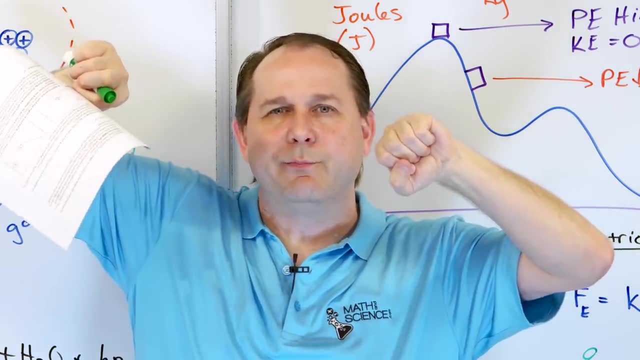 states to low energy states. So, in summary, before we solve our problem, if we start in a high energy state, high potential energy, if we allow the system to pull and literally have a force acting through a distance- and now I stop again- then the potential energy. 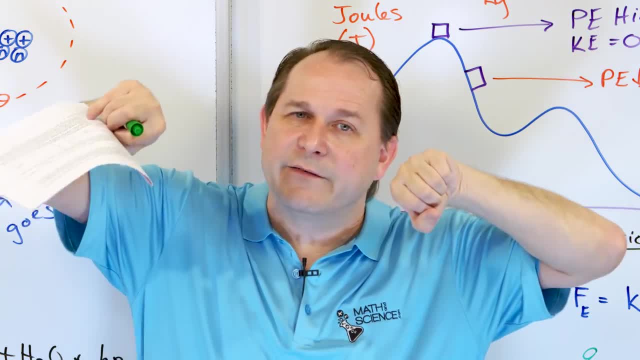 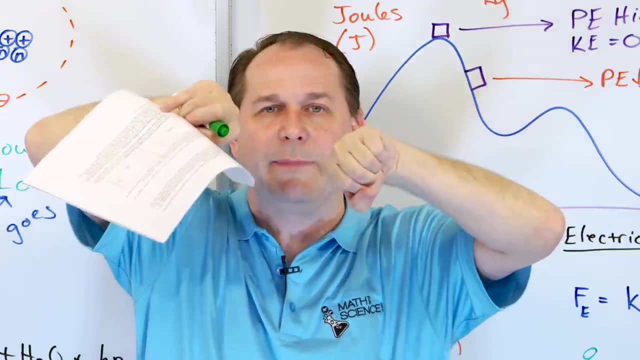 is converted into the energy of what we call work, Because a force acted through a distance and now the molecule is stopped again, There's no motion happening. If I allow the rubber band to pull on me and I stop again, I'm not moving anymore. So there's no kinetic energy, but the energy. 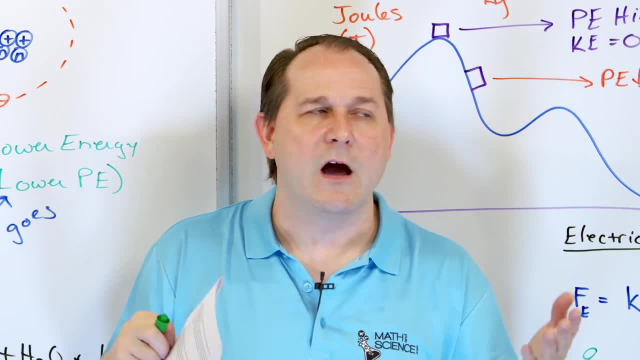 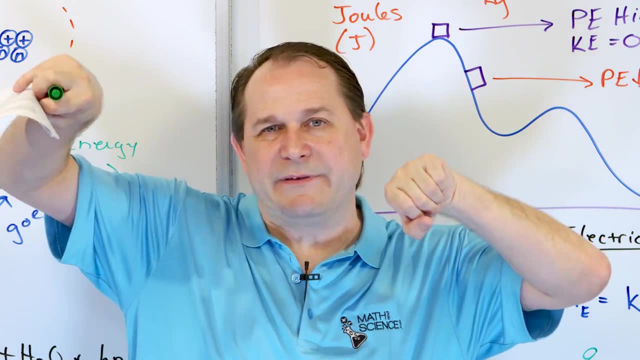 was converted to work. That's just another way of solving the problem. So if we start in a high energy state, it's another way of manifesting energy When things move, but then they stop again. That's case number one. Maybe the potential acts on something and then it stops. Okay, 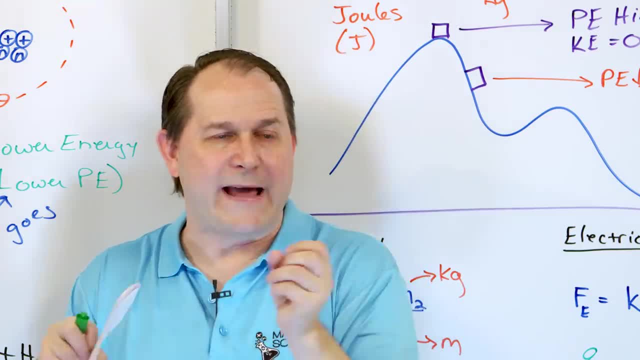 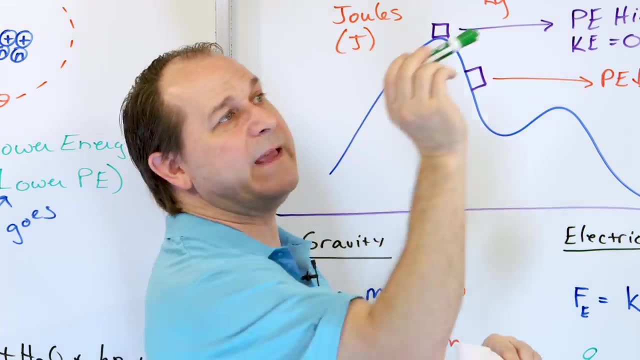 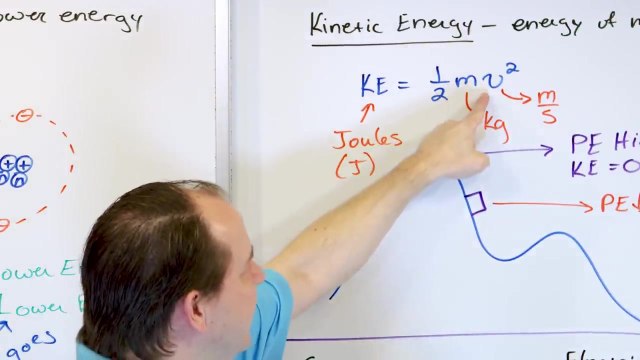 so it's converted to work. But if I pull the rubber band and I shoot this marker across the room, the potential energy is converted to a different kind of energy called kinetic energy, because now the thing is moving with velocity v And notice that it's one half mv squared. So the velocity 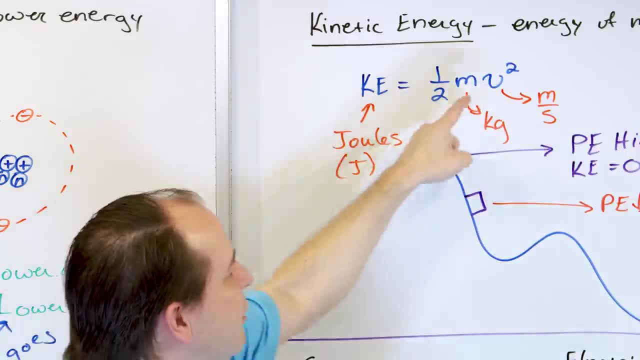 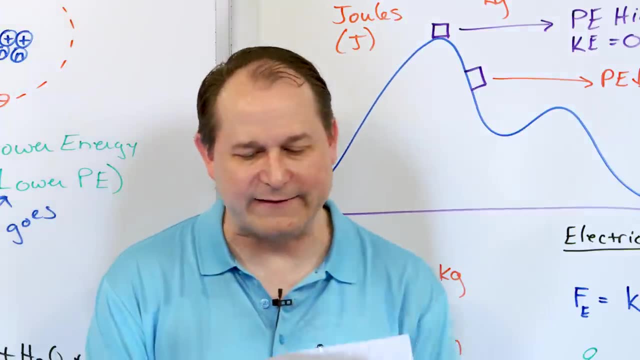 actually matters a whole lot more than the velocity. So if I pull the rubber band and I calculate in the kinetic energy- because it's velocity squared, Velocity times, velocity, All right. kinetic energy, potential, energy work, Lots and lots and lots of stuff there I really 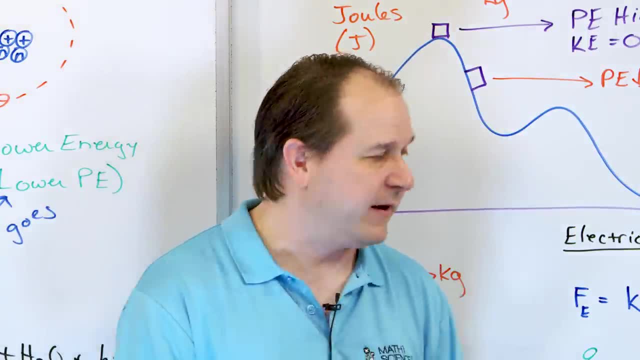 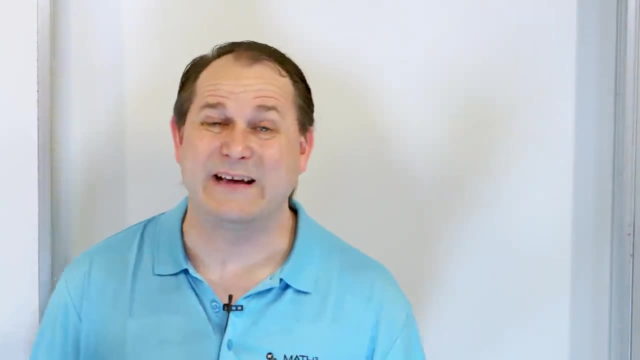 would like you to solve, to watch this a few times, because it takes a while to sink in. Now I do want to do a couple of really quick problems. One of them is going to be calculation and one of them is going to be conceptual, Just to do something in this first lesson here. Here's: 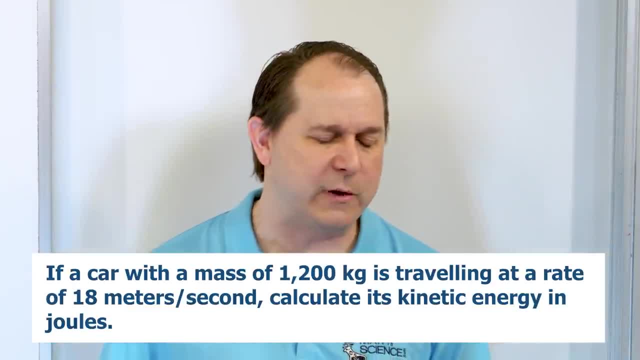 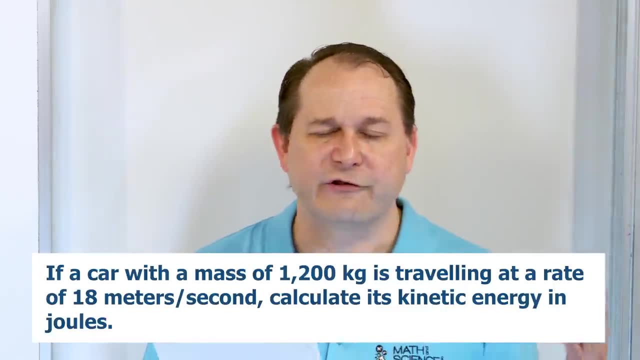 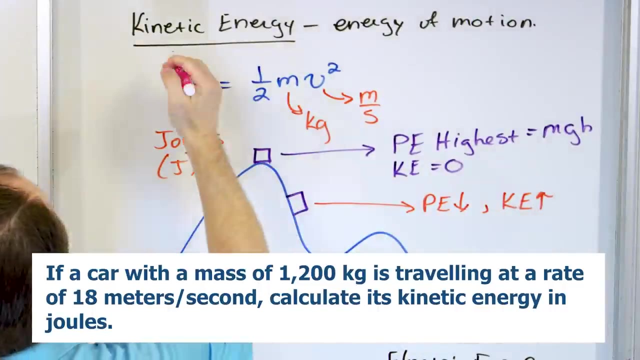 the problem. If a car with a mass of 1,200 kilograms is traveling at 18 meters per second, calculate its kinetic energy in joules. So this is a straightforward application. If I had to circle the equations that were most important in this lesson right, this would be one that was: 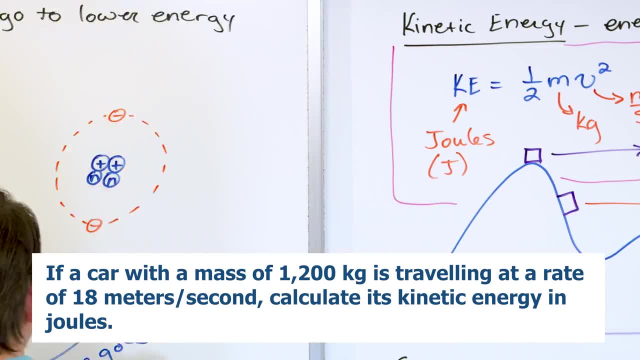 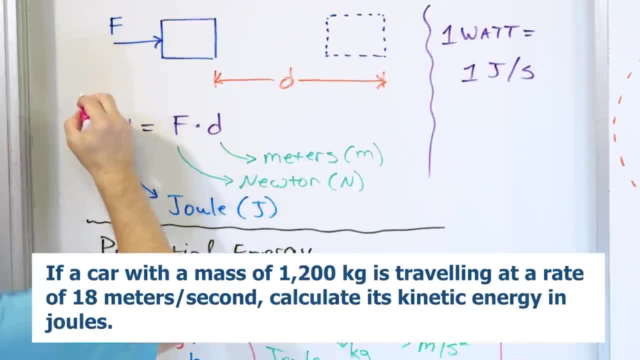 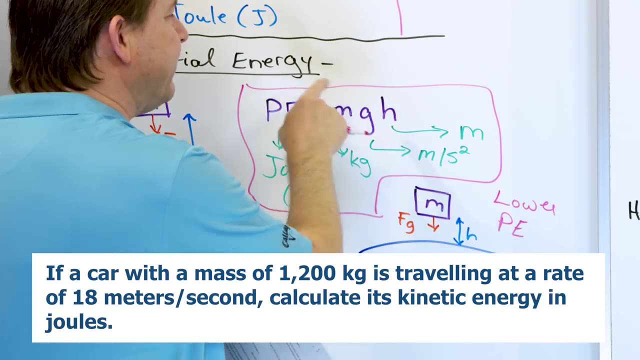 extremely important, right, And then over here, this would be one that's extremely important, And then the last one would be this one That's extremely important. There's basically three equations: Work is force times distance, Potential energy is m times g times a. And then the last one. 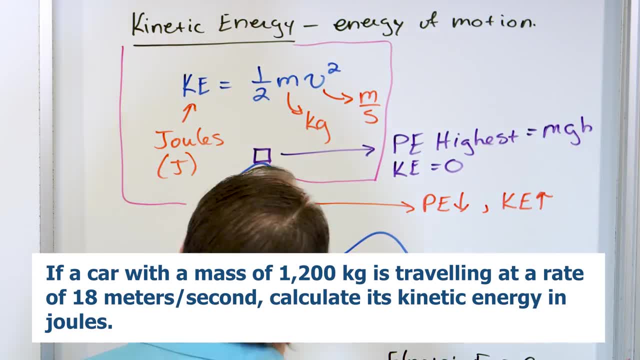 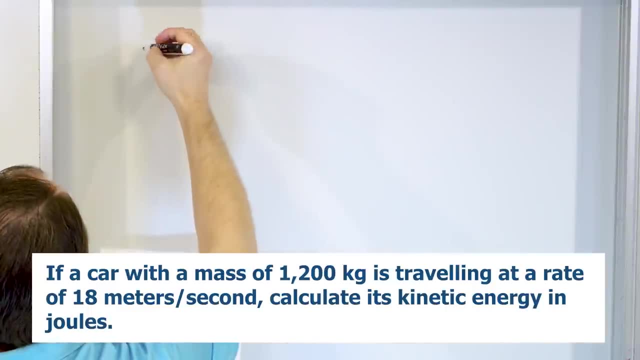 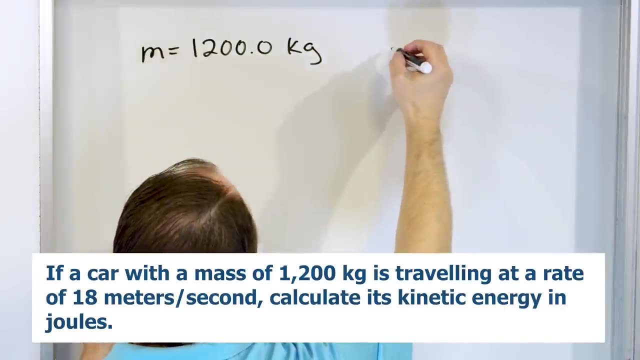 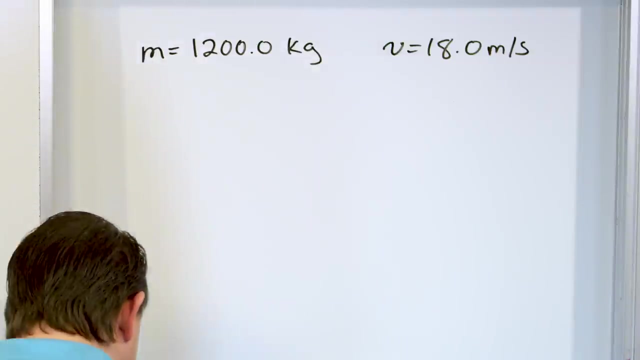 is h, And then finally, we have 1 half mv squared for the kinetic energy. So in our problem statement it says that the mass of the car is 1,200 kilograms And it's traveling at a velocity of 18.0 meters per second. So how do we calculate the kinetic energy? Well, it's a straight plug-in. 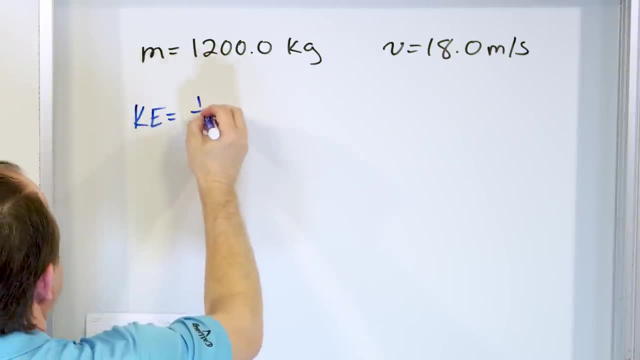 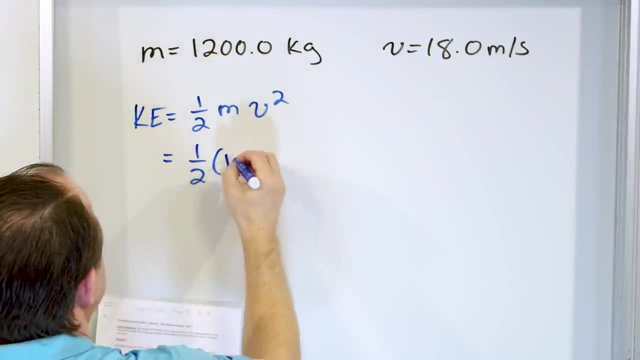 type of situation. The kinetic energy is 1 half mv, squared for the kinetic energy, And then finally, we have 1 half times m times v squared right, Which is 1 half times the mass of 1,200.. And then we have the velocity, which is 18 meters per second. If you were not given 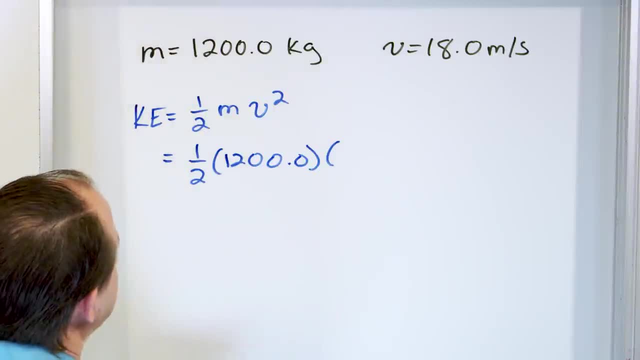 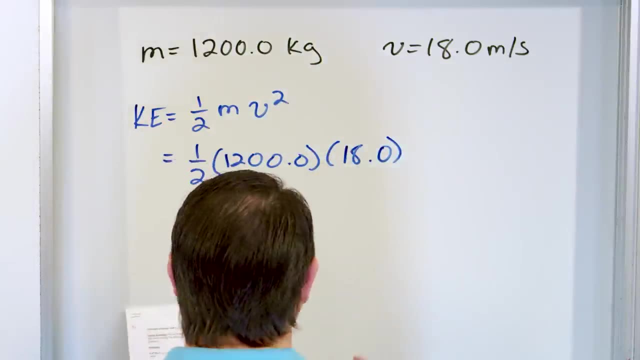 the velocity in meters per second, you would have to convert it to meters per second. If you were not given the mass in kilograms, you would have to convert it to kilograms. But here everything is already given to us like this: We just times 18, and it's got to be. 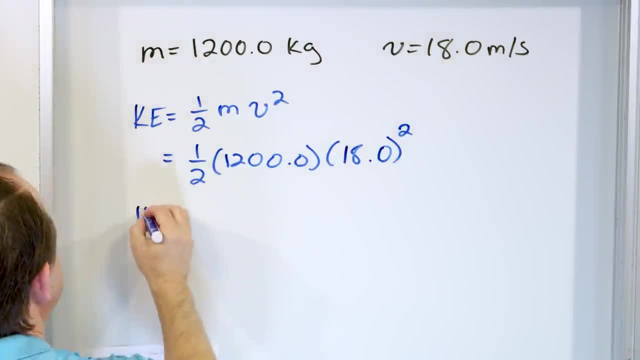 squared 1 half mv squared right, And when you calculate this you get an answer of 1 half mv of 194,400 joules. So 194,400 joules. And then we can just kind of write that in scientific. 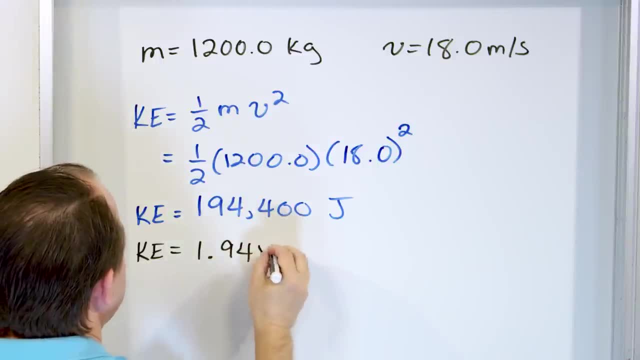 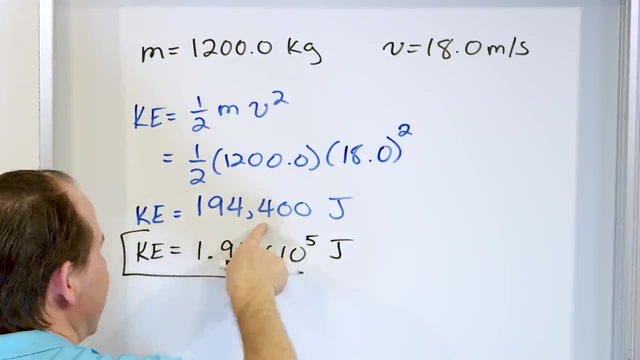 notation and do some rounding with, say, 1.94 times 10 to the starting here: 1,, 2,, 3,, 4,, 5 joules. You can write it any way you want. I'm rounding here because this is a 4.. And I don't. 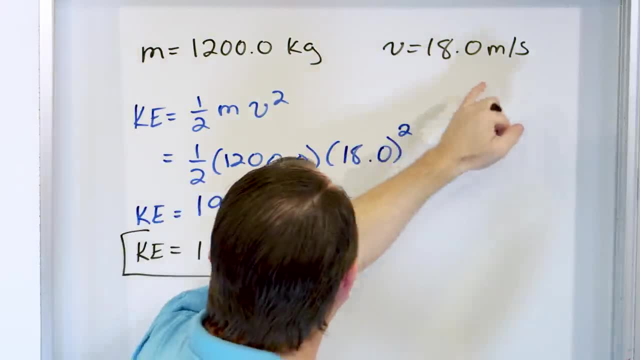 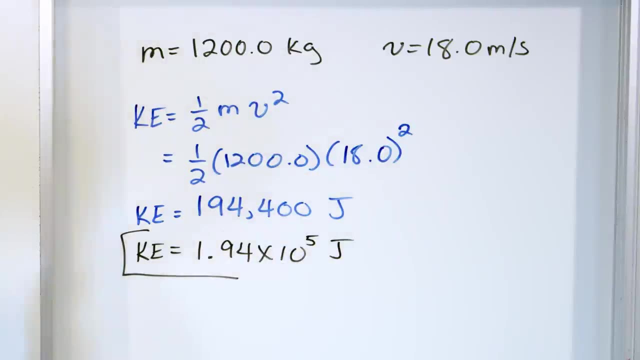 need to keep all the. you know I only have my velocity to three digits here, So I'm going to keep three digits here. 1.94 times 10 to the 5. That is a unit of joules. Now that's the kinetic energy, right? So this is a car with that mass. 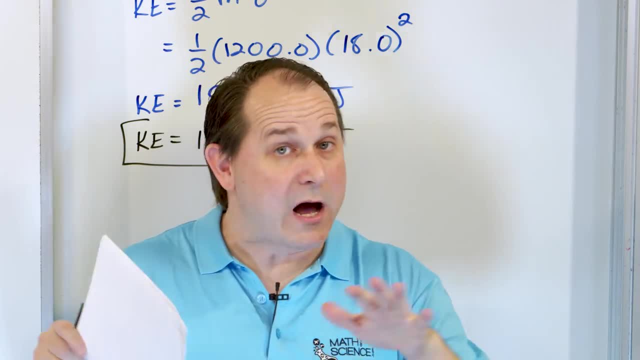 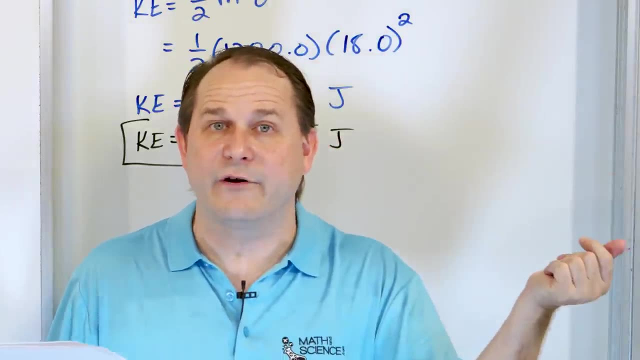 that's traveling at that speed. Now, if you're at a red light and you're not moving, and I asked you how much potential energy was used to accelerate the car to that speed, then you know the answer, because if the car now has this much energy, then that must have been the potential energy used in. 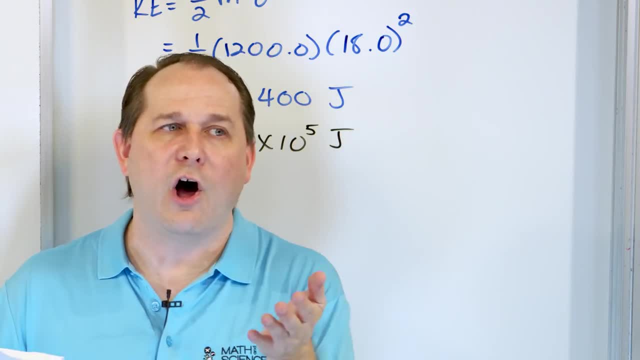 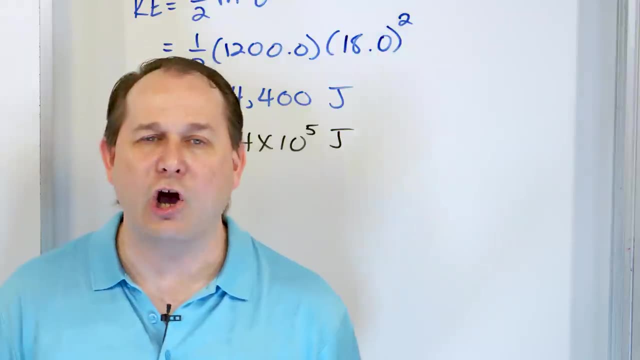 the gas tank and the combustion to get the thing to accelerate, because all of the energy of motion has to have come from somewhere. Just like the roller coaster, it all came from gravitational potential energy. In the car, when you start from a dead stop, it has to come from the gasoline. And where does that come from? Breaking 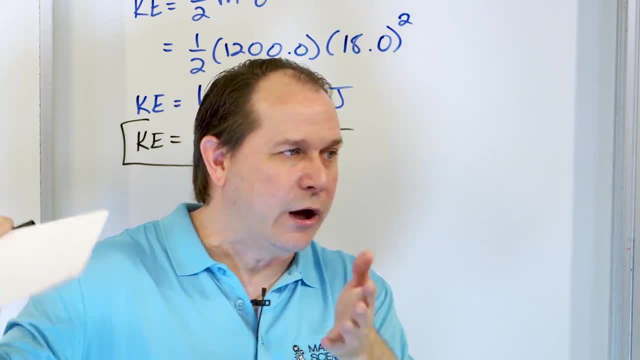 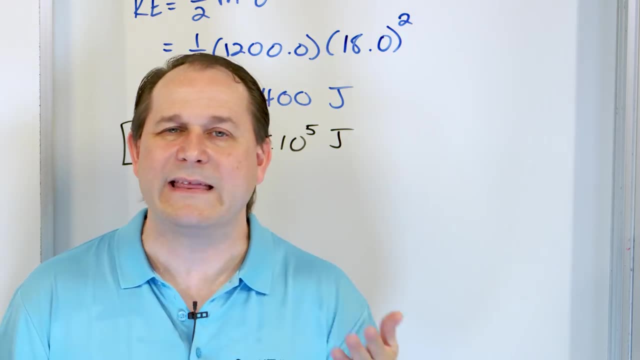 the bonds of the gasoline and burning it goes to a lower energy state in the pistons and creates heat, And that heat is essentially the. you have losses and everything, but that is what's driving the car forward, right? So that's problem number one, just a straight calculation of kinetic energy. 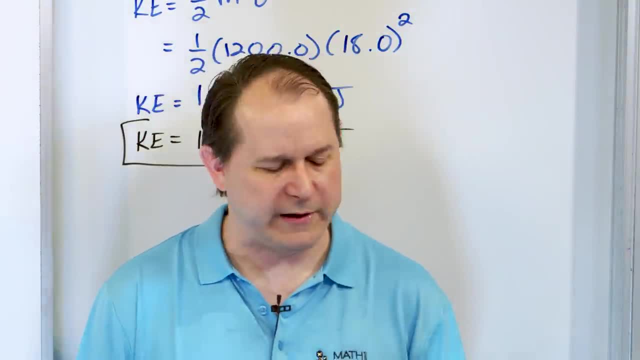 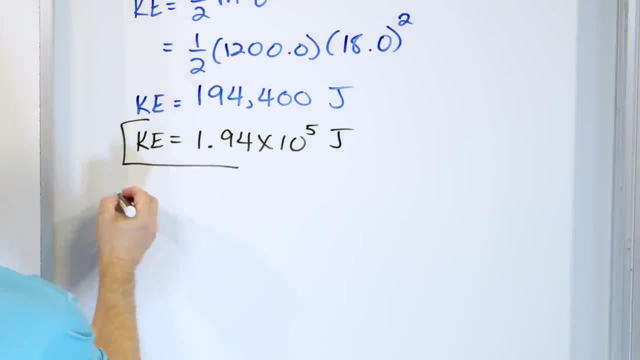 Now here I'm just going to read the question out and just kind of talk about the answer. There's more than anything. Here we go For each of the following: explain which has the higher potential energy and why, And so I'll just put A and B. There's really two little things that we're. 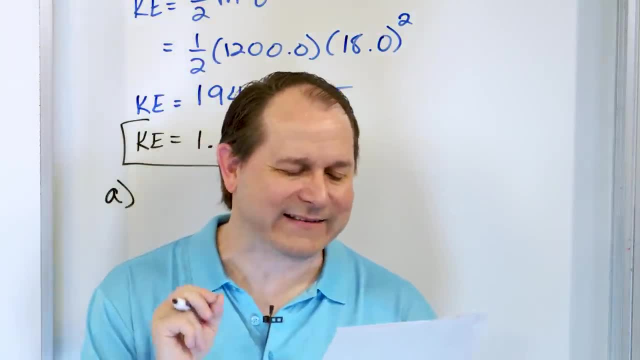 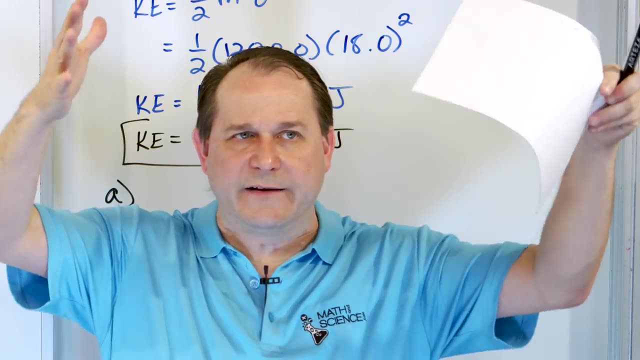 going to talk about Which one has higher potential energy and why: The gasoline in your car's tank or the gaseous substances coming out of the car's tailpipe. So you have like a box called a car. Gas is in the tank, Gasoline is in the tank, It goes to an engine. a chemical reaction happens. and what comes out? The tailpipe. You're not an expert in cars, neither am I, but it's carbon dioxide and water. Most things that burn give you CO2 plus H2O, So the question is, which has the higher potential energy? 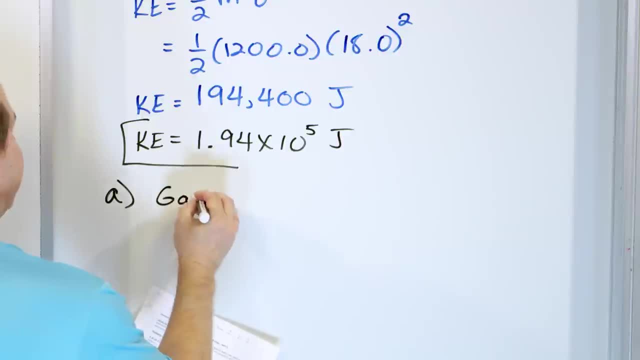 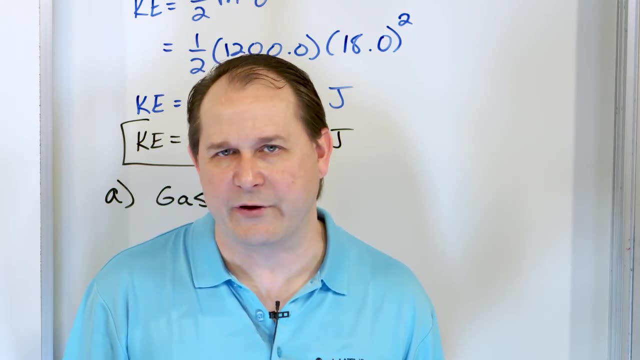 Well, the answer is: the gasoline has the higher potential energy, And you know this because the car's function is to move, And the only way to get it to move is to get energy from somewhere, And the only energy you put into the car is the gasoline. So the energy has. 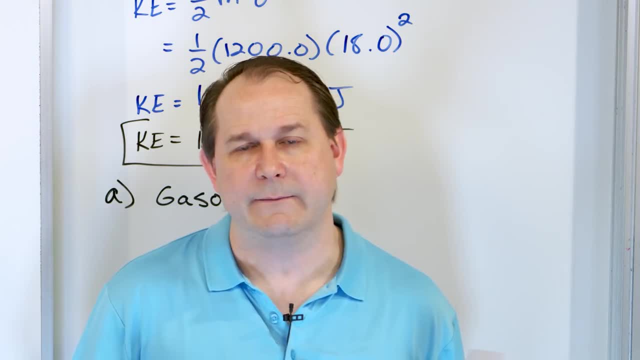 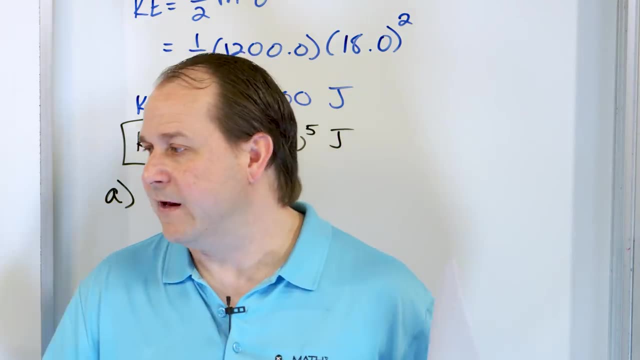 to come from the gas Where? From the chemical bonds of the gasoline, Because when it burns those bonds are broken down and that energy goes into the energy of heat, into the exhaust And of course that's moving the pistons. The heat is moving the pistons. 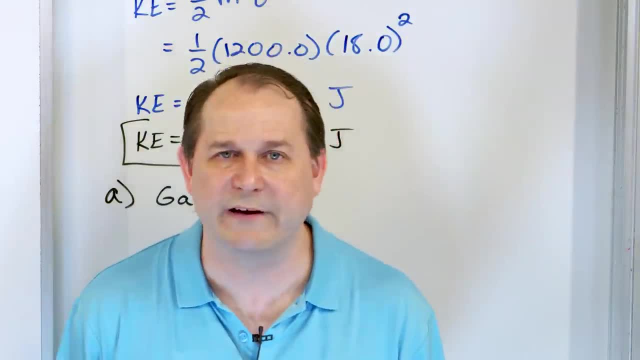 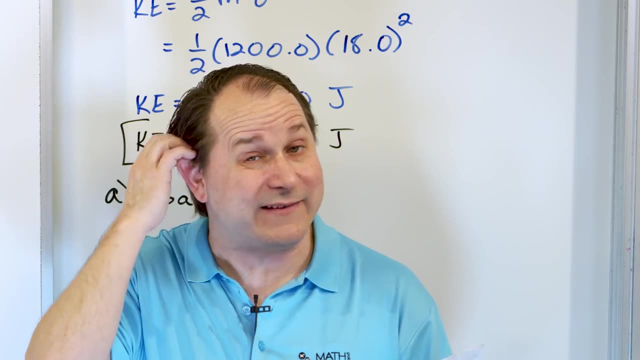 and that energy is driving the car forward. Now it's not 100% efficient. A gasoline energy is not 100% efficient, Not even close to 100% efficient, But that is where the energy is coming from. So because of that, we know the gasoline has to have higher potential energy, Whatever comes out. 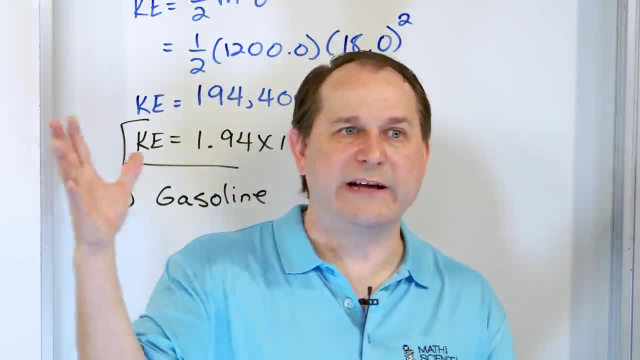 the tailpipe has to be in a lower energy state In order to get the car to do anything. we have to get the energy from somewhere And that's what the car is going to need. That's what the car's going to need. So we're going to have to place everything in the car if that's what we want. So if you do, 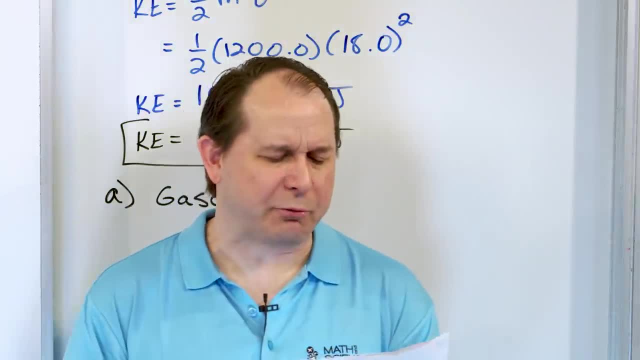 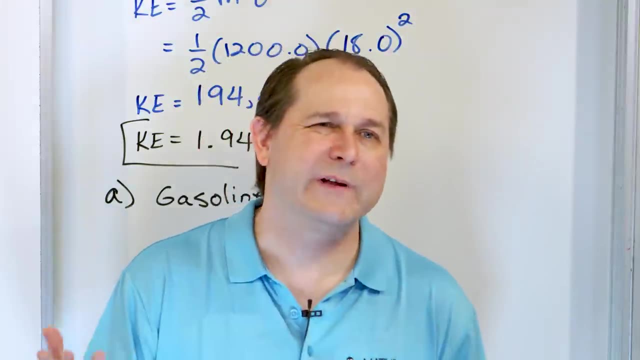 energy from somewhere. And the last problem: which one's higher, which one's lower? Wood in my fireplace, or the ashes that remain after a fire, And it's really kind of the same question, because we know gasoline is burned, We know wood is burned in a fireplace. So what has the higher? 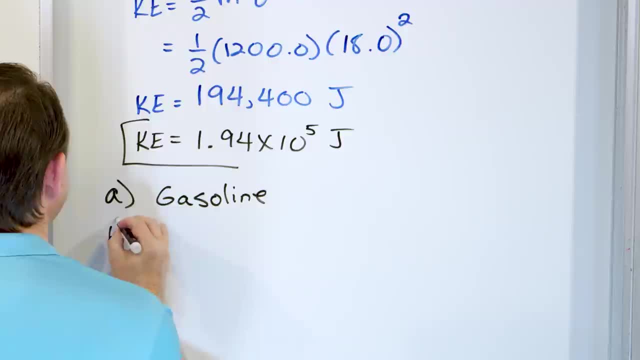 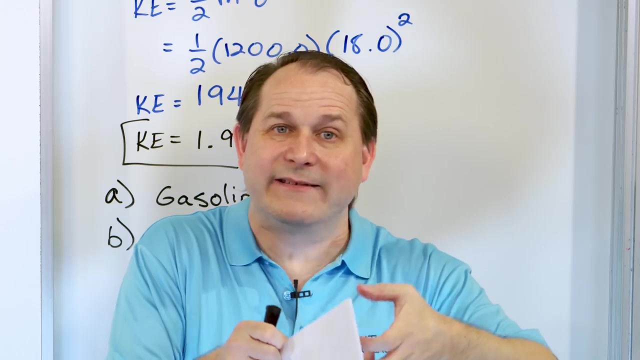 potential energy. It's going to be the wood. So we'll say wood, We'll say it has the higher PE and gasoline has the higher potential energy. Same exact reason When you burn wood. where is the heat and the light coming from? Well, it's coming from the bonds inside the wood. And 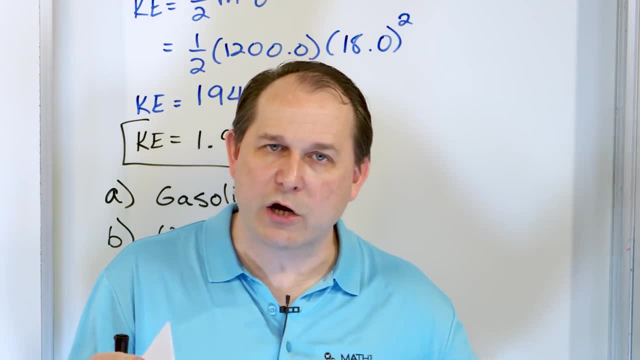 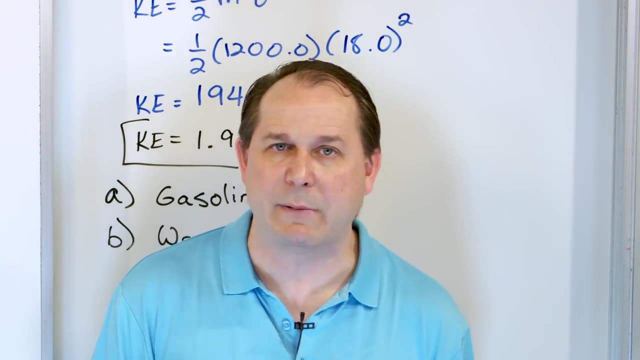 when you burn it, you're breaking those bonds. You're combining it with oxygen and water and carbon dioxide are produced, And those substances, as I told you a few times, are in a lower energy state. So the ashes that are left behind, the soot and all the things that floated up from the 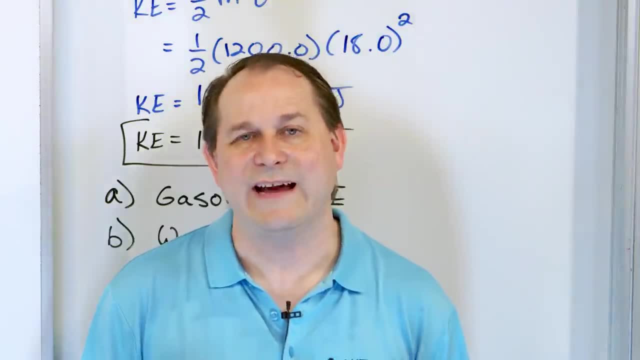 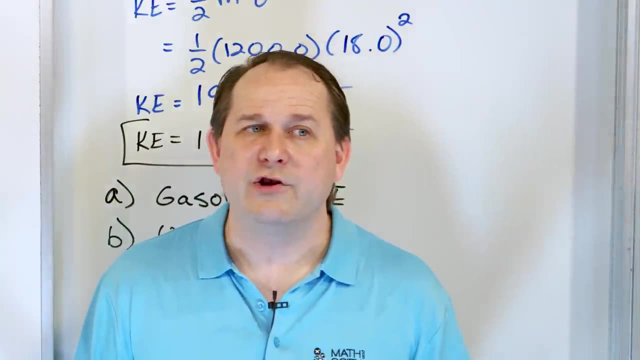 campfire. if you add all that stuff together, that's all in a lower energy state. It has to be because the Fire released energy in the form of heat and light And so that energy had to come from somewhere. You can't just have a reaction where you get free energy. So a lot of people say